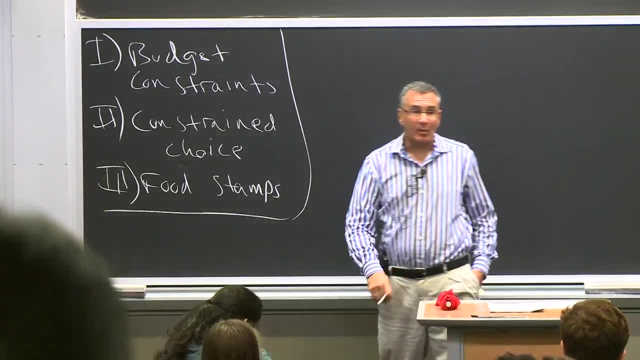 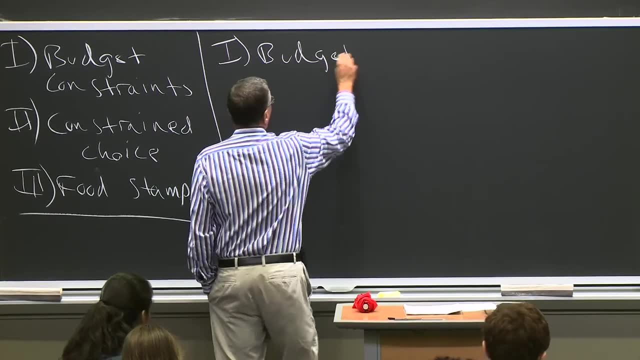 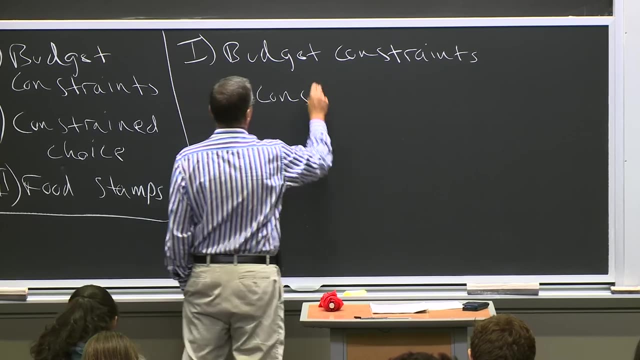 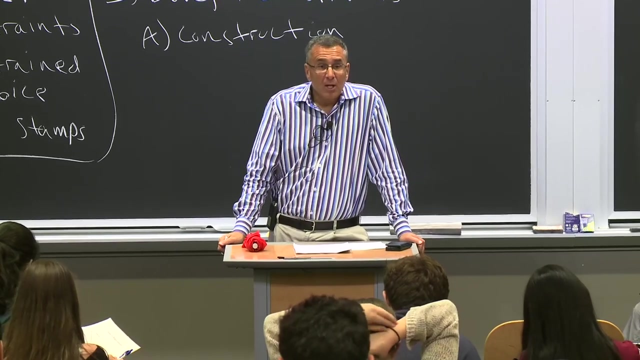 talking about how consumers make constrained choices, and then we'll end with an example of food stamps. So let's start by talking about budget constraints And we'll start by talking about their construction, the construction of budget constraints. So, basically, last time we talked about the fundamental axiom of consumer choice, that more is better. So 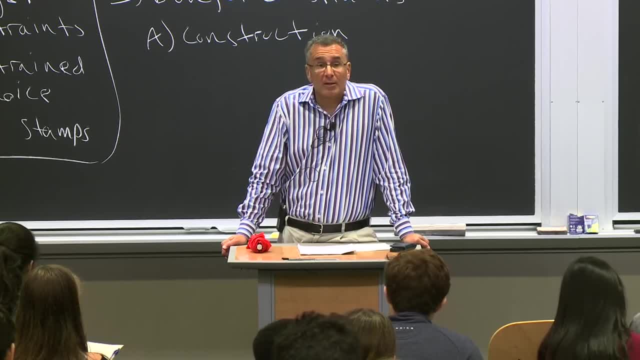 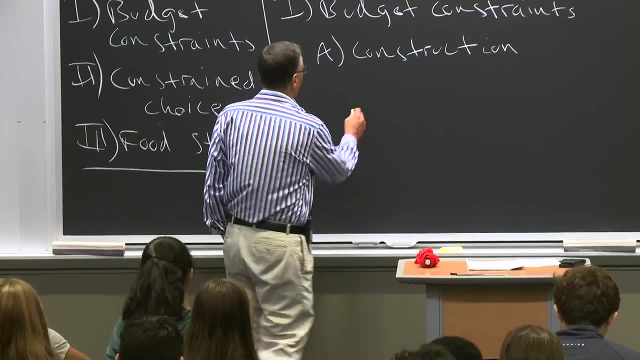 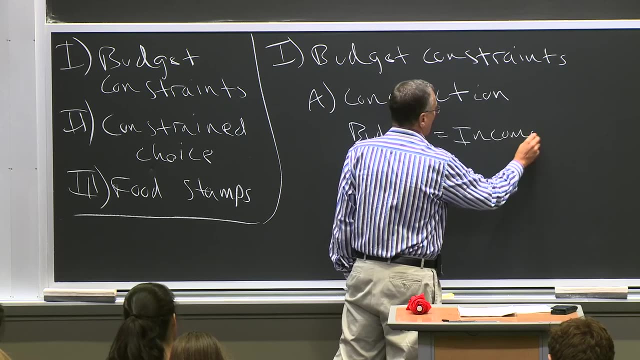 what's the opposite? It's their budget constraint, It's their limited resources. Now, for most of this course, we're going to make a simplifying assumption: that your budget- that is what you spend- equals your income. That is what you earn. Okay, That is. there won't be any savings. 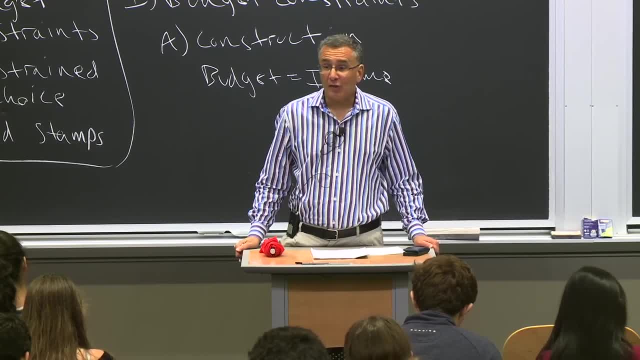 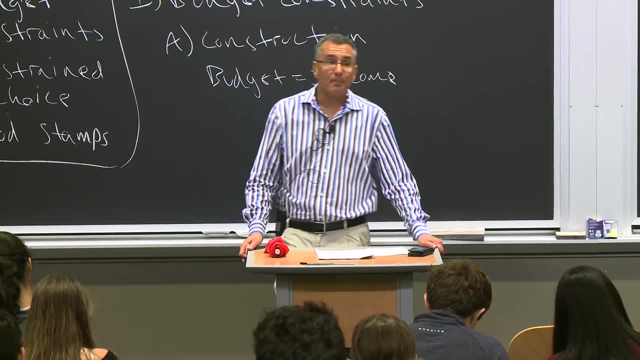 or borrowing. Okay, Now, that is a simplifying assumption, and indeed we'll spend a couple lectures at the end of the semester talking about what happens when people can save or borrow. That said, this is not a terrible description of most Americans: The median 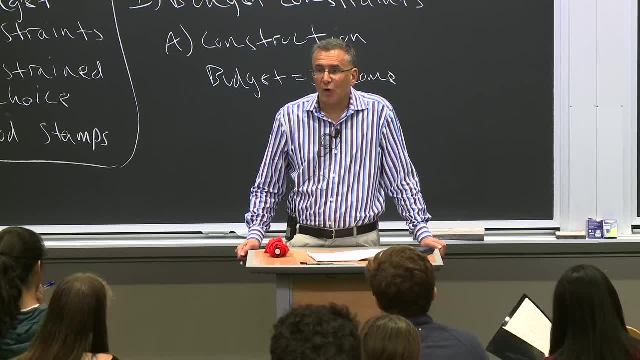 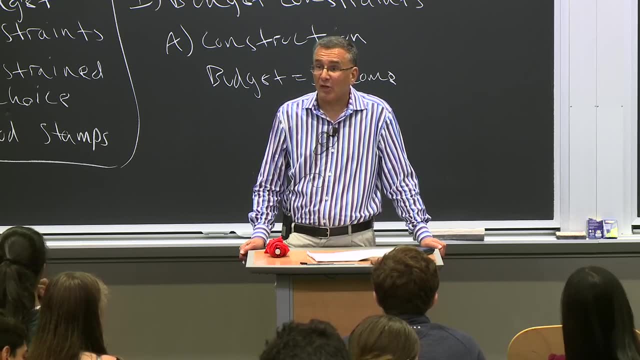 American household has $400 in the bank. So this is not kind of a terrible description of the way most people live their lives in America, which is what they earn each week is what they spend each week. So that's what we'll do. It also might not be sort of a terrible. 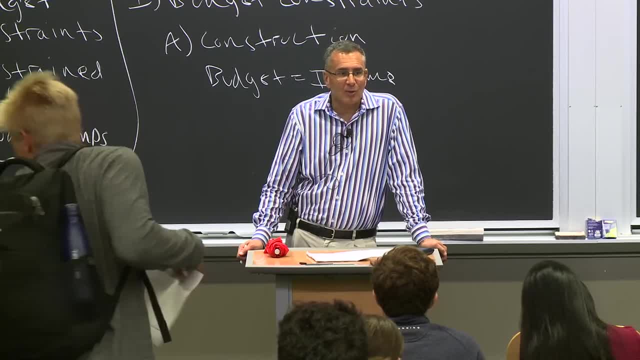 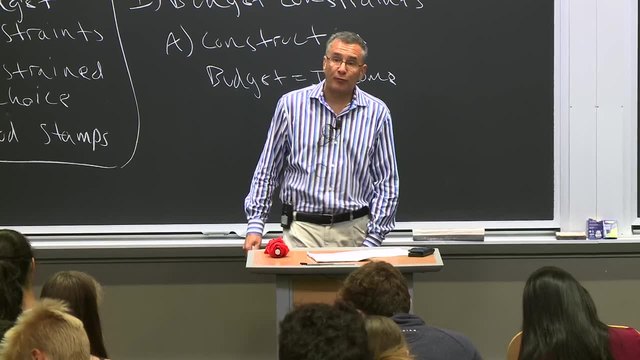 description of your life. I presume in college you're not doing a lot of savings. You maybe do a little borrowing, but not a lot of savings or borrowing. So we're going to talk about that. What we're going to do is we're going to assume that's true for you as well. We're going to 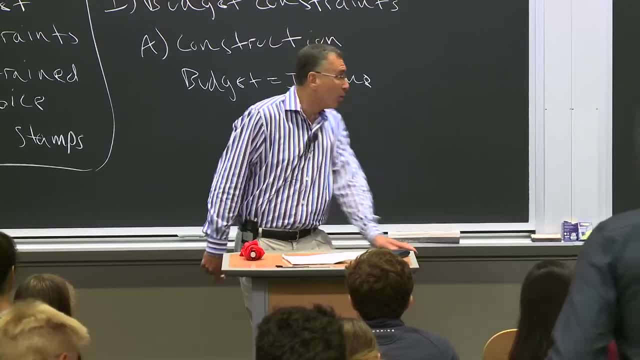 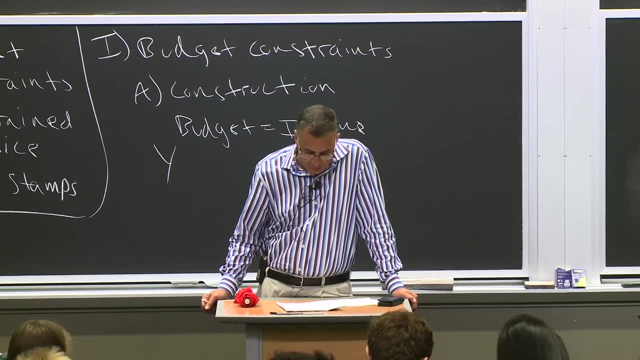 assume your parents have given you some amount of money to spend. We'll call it Y Your income. Y is the amount of money your parents have given you to spend for, say, the semester or the month. And once again, let's say, all you spend your money on is pizza and cookies. 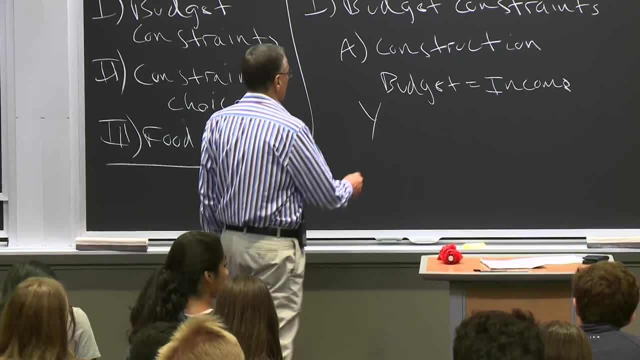 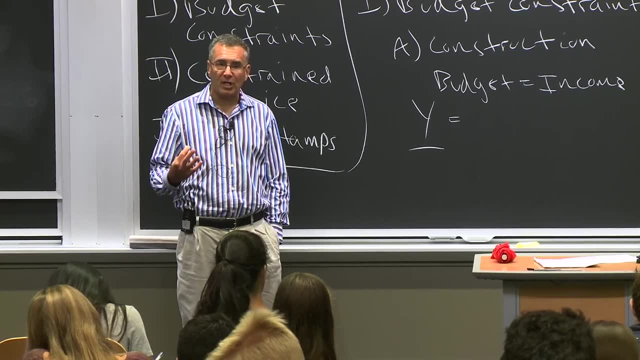 Okay, That's all you want to spend your money on. We write the budget constraint as saying that your resources, your income Y can be spent on either pizza or cookies, And that's what we're going to do, And the constraint is that you could spend it, that that budget has to be divided between. 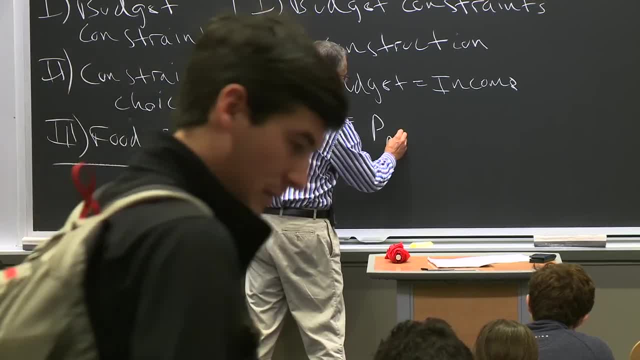 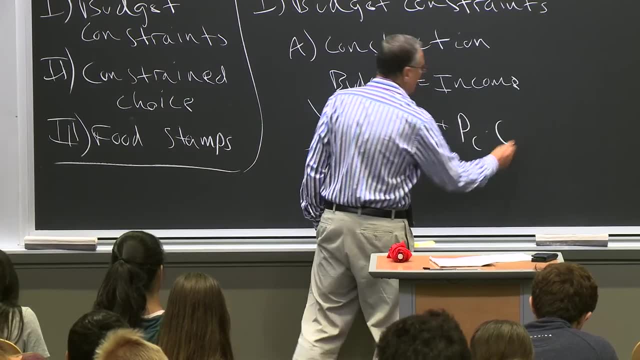 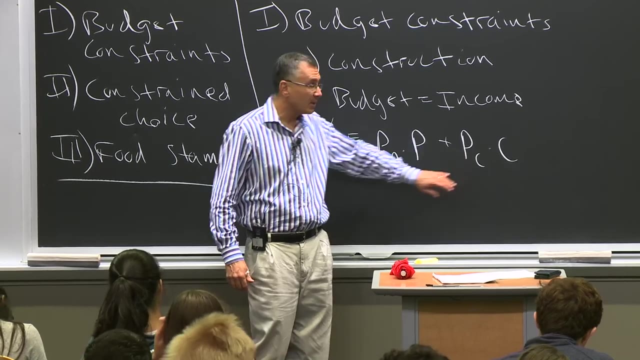 pizza, where there's the price per slice of pizza times the number of slices of pizza, or cookies, where you have the price per cookie times the number of cookies. So P sub P is the price per slice of pizza, P sub C is the price per cookie, P is the number of pizzas. 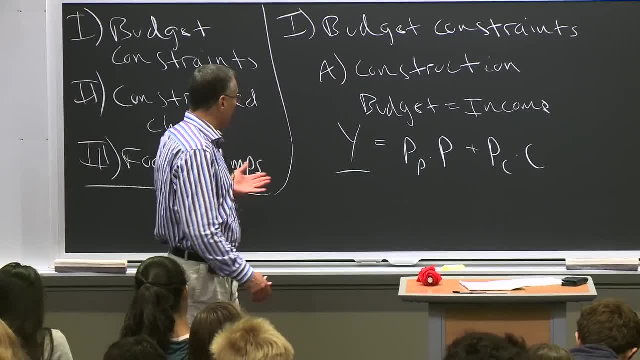 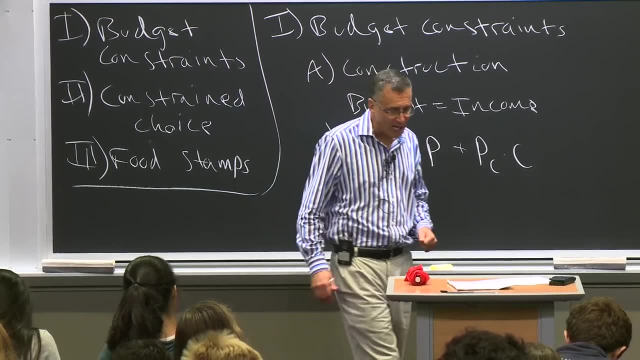 and C is the number of cookies. That's your budget constraint. You can essentially devote your income to some combination of pizza and cookies, but you have to consider how much they actually cost. in doing that, I find this easier to see graphically. so let's turn. 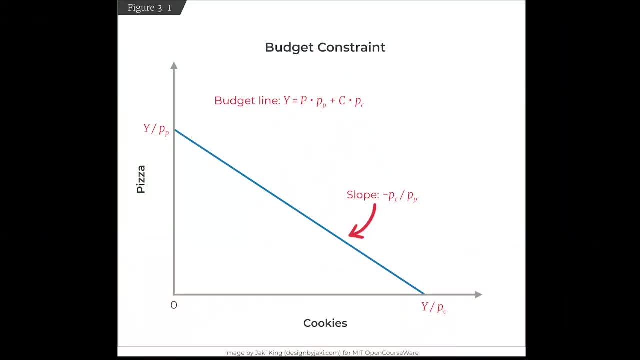 to figure 3-1.. Figure 3-1 shows a budget constraint. So how does the budget constraint look? Well, the x-axis is your income divided by the price of cookies. That is, if you decide to devote all your income to cookies, then how many cookies can you have? Y over PC, If your income 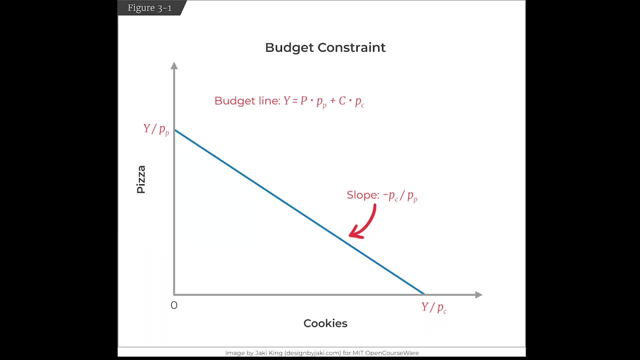 is $100 and cookies are $10, that means you're going to insomnia cookies, then you can only have 10 cookies, et cetera. Likewise, the y-intercept is the income divided by the price of pizza. That's how many pizzas you can have. The budget constraint represents the budget. 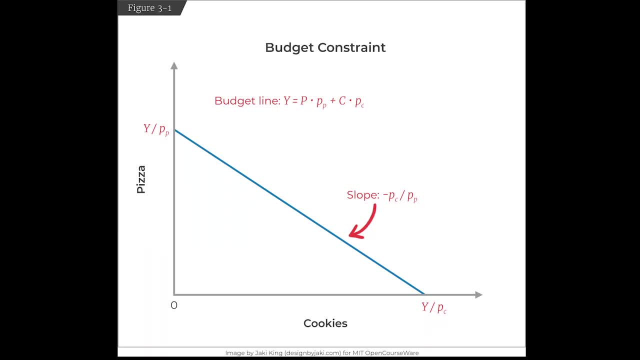 constraint, The slope of the budget constraint, is the price ratio. the negative of the price ratio: Good, Because it's a downward sloping line. PC over PP, That is, every extra cookie that you buy, holding your income constant, lowers the amount of pizza you can have by P sub P. So let's consider: 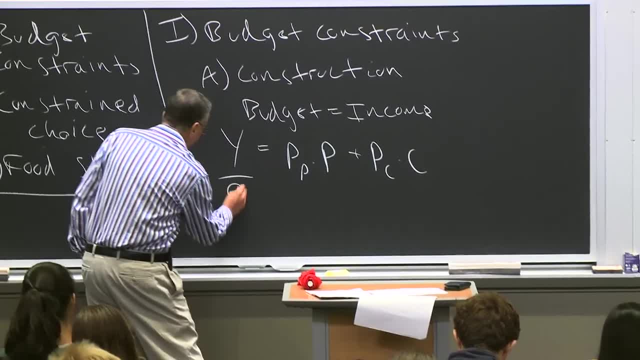 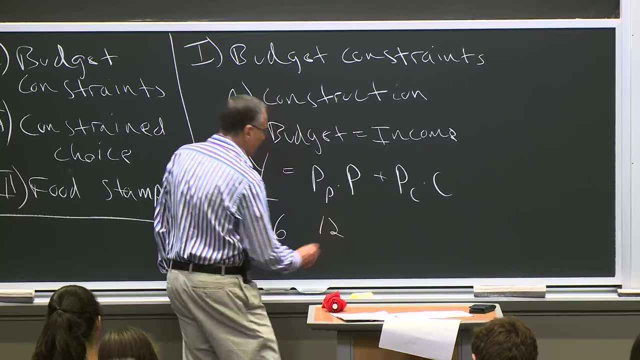 an example: Suppose that y is $96, that the price of pizza, this expensive pizza place, is $12.. Let's take a look: $96 and the price of a cookie is $6.. $6 is a $12 free pizza. 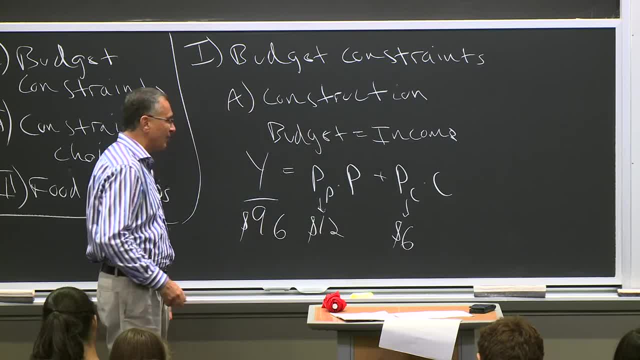 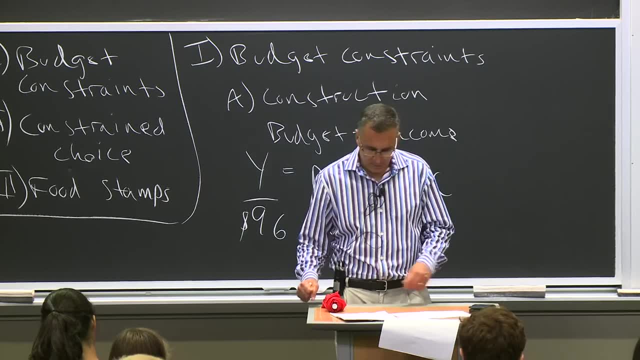 And the price of a cookie is $6.. $12 for pizza. This is like downtown San Francisco or New York: $96 income, $12 for a slice of pizza, $6 for a cookie. I'm sorry, We're going to make Y-72.. 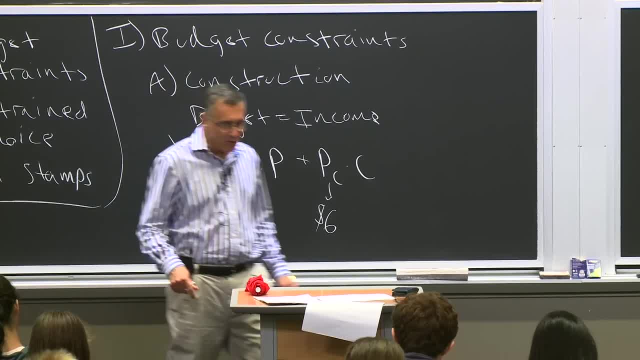 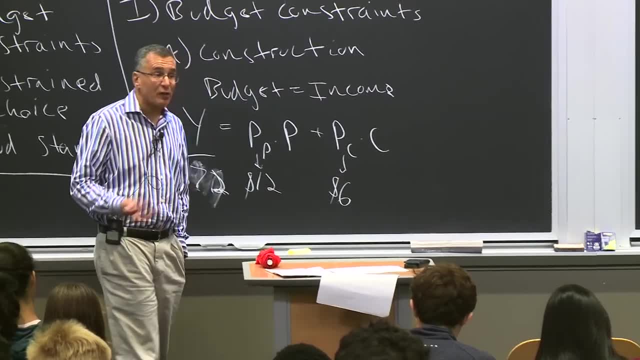 My bad, It's Y-72.. Your income is $72.. And you could spend it on pizza and cookies, And those are the prices. What that means is, if you want just pizza, you can get six pizzas. If you want just cookies, you can get 12 cookies. 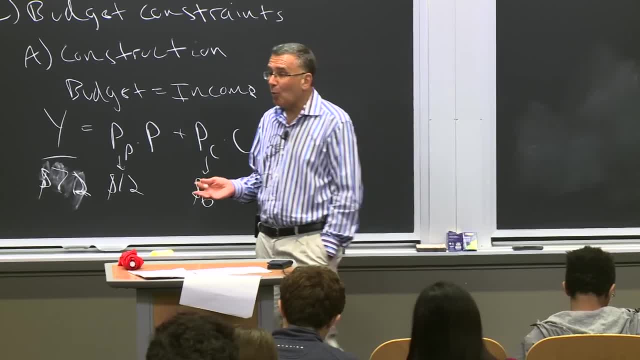 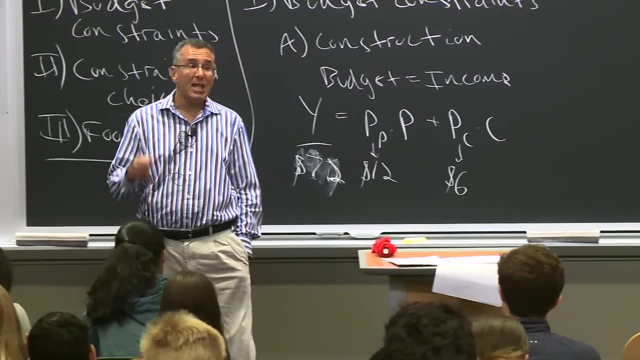 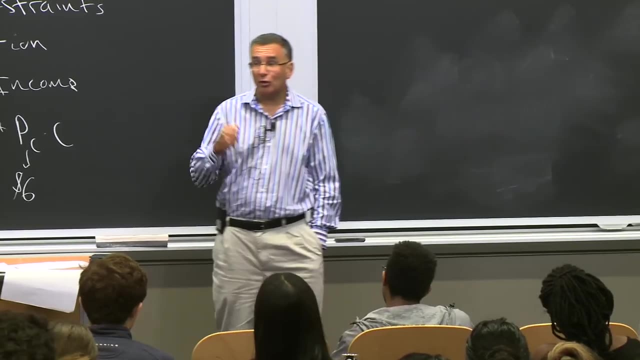 And generally the rate at which you can trade off pizza for cookies is minus a half. That is, every additional cookie would require giving up half a slice of pizza. Every additional cookie requires giving up half a slice of pizza. that's why the slope would be negative a half. 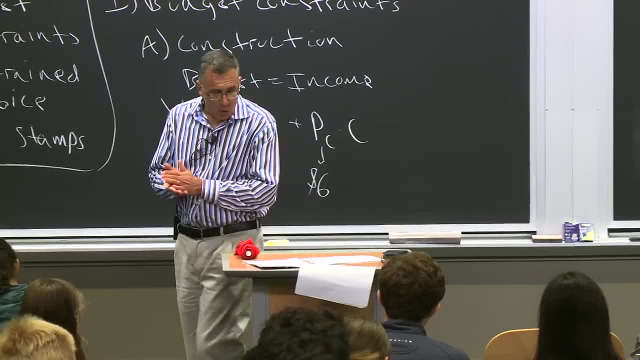 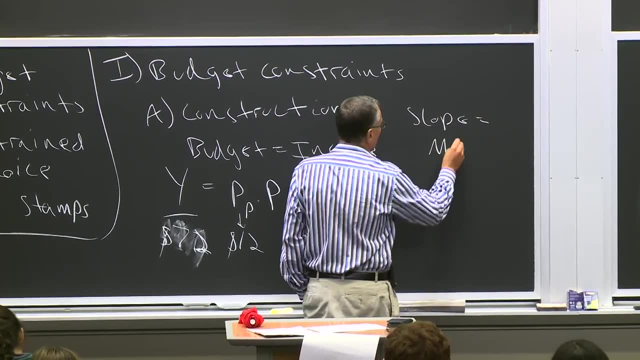 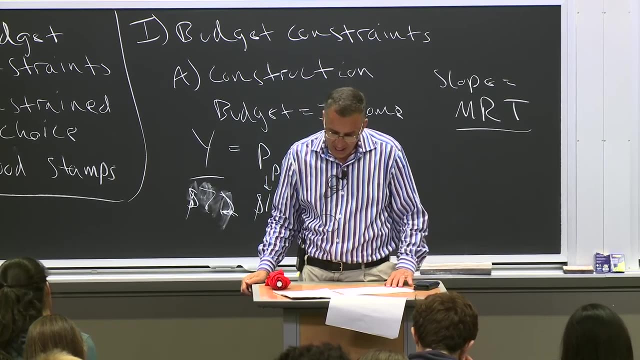 So basically, we're going to call the slope of the budget constraint the slope. we're going to call the marginal rate of transformation, The MRT. last time with the MRS, the marginal rate of substitution, Now we're going to have MRT- the marginal rate of transformation. 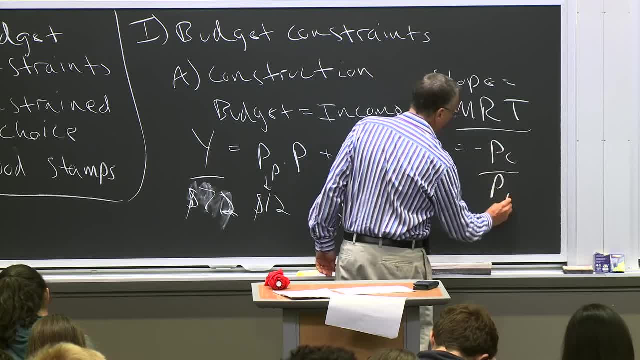 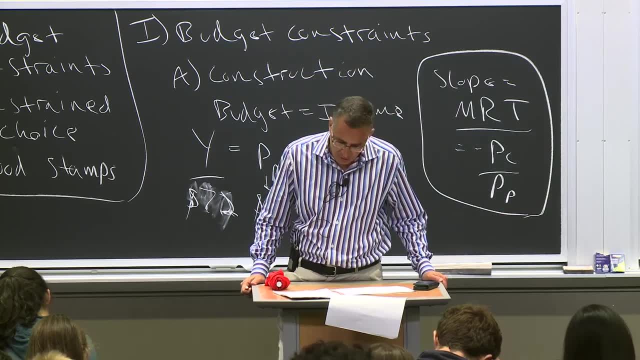 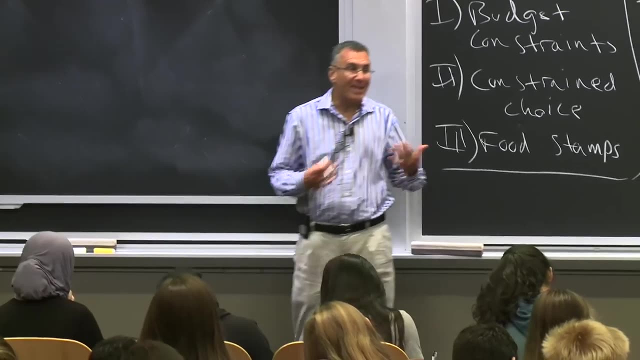 which is equal to minus PC over PP or the slope of the budget constraint. That is the marginal rate of transformation. Now, this class is not alchemy. We are not literally transforming pizza into cookies. That would be kind of cool, but we're not doing that. 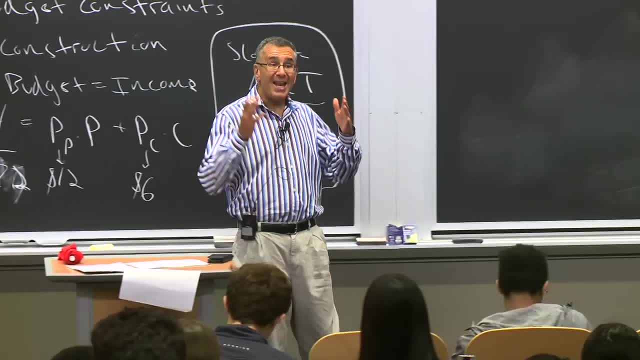 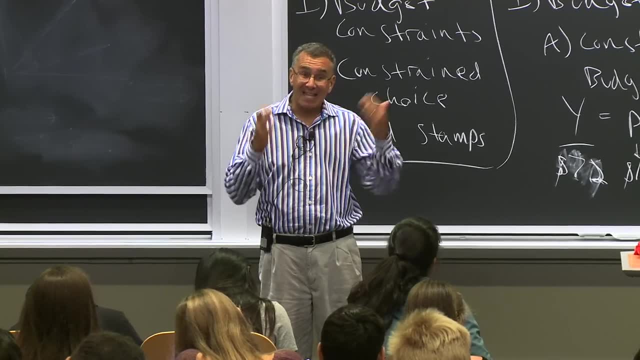 That's somewhere else at MIT, But effectively doing the same thing. What we're doing is, given that we have a fixed amount of money and given that we're going to spend it all, the more you spend on pizza, the less you spend on cookies. 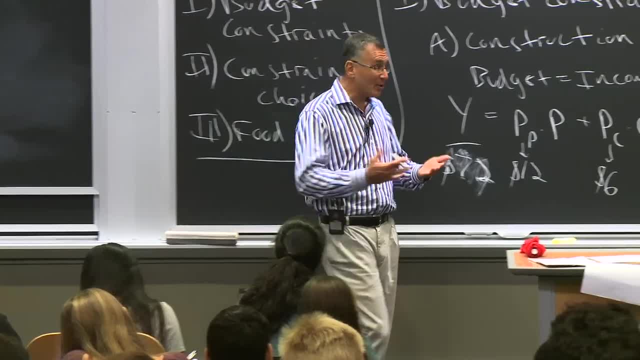 So you're effectively transforming pizza into cookies and vice versa, Because you're going to spend it all. You're not going to spend all your money. You've got to spend it on something. So the more you spend on one, the less you get of another. 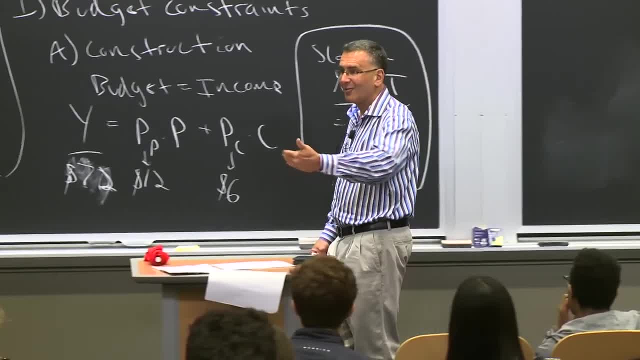 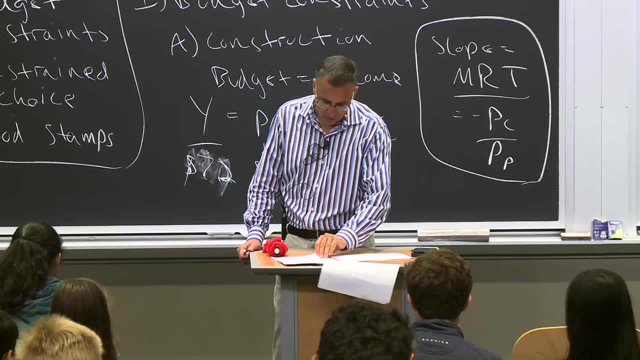 So, through the budget constraint, we are effectively transforming one good to the other. By having more of one, we're getting less of the other. So that's the sense in which we call it the marginal rate of transformation. So, basically, this comes back to the key concept we talked about in the very first lecture. 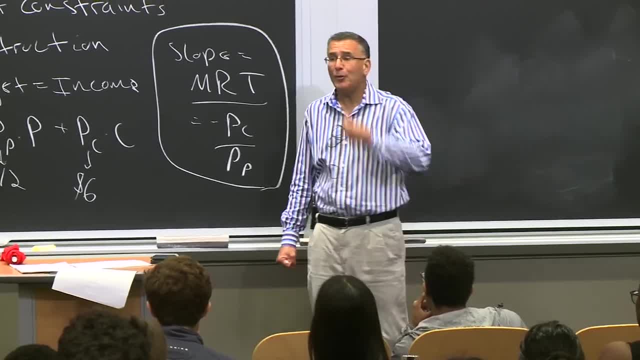 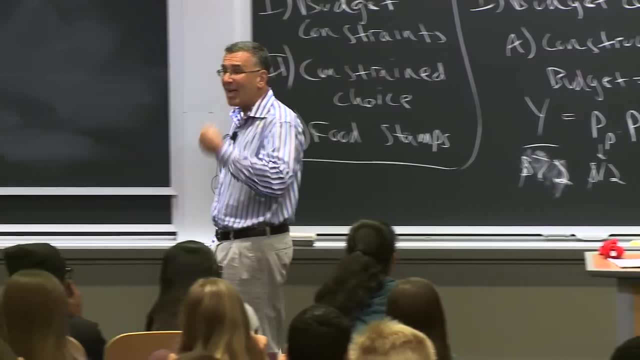 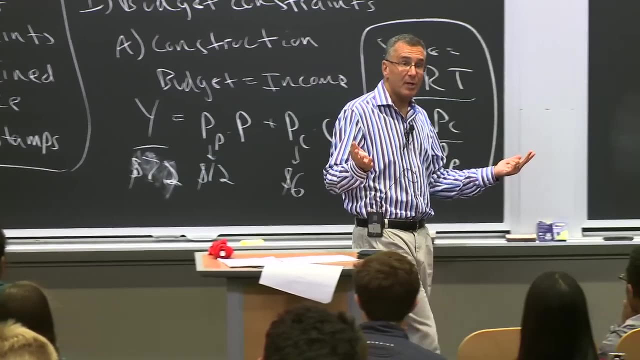 opportunity cost. The opportunity cost of a slice of pizza is two cookies. Remember, opportunity cost is the value of the next best alternative. The opportunity cost is the value of the next best alternative. Well, here you only have two alternatives: pizza and cookies. 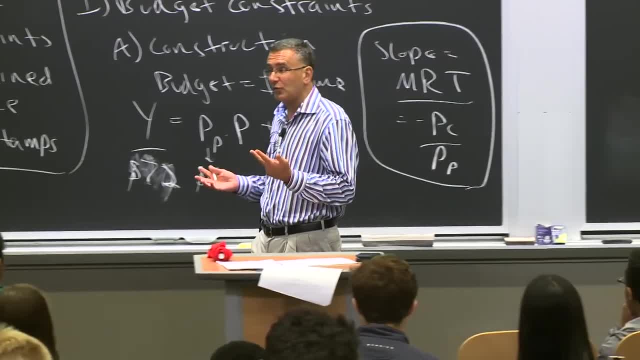 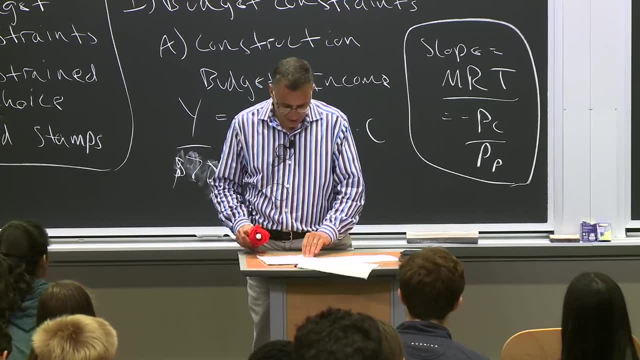 So the opportunity cost of a slice of pizza is two cookies, And that's the sense in which you're transforming pizza into cookies or cookies into pizza. Now this seems kind of abstract, but let's actually think of an organization which has taken this principle to heart. 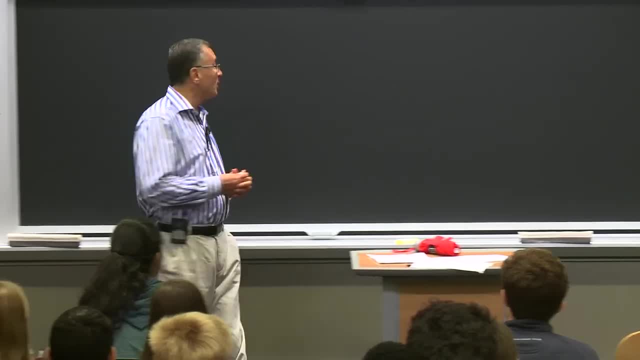 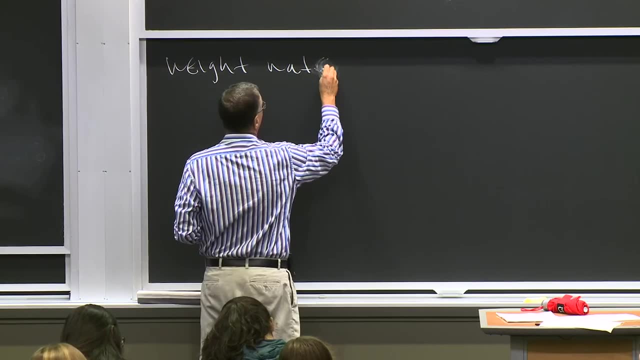 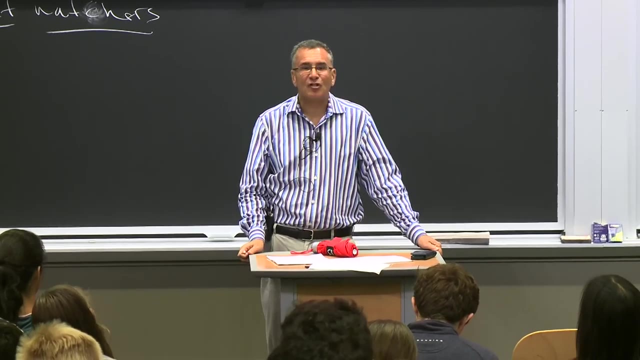 to develop the best method of weight loss in America, which is Weight Watchers- Okay, Weight Watchers. Now it turns out that dieting is super hard and basically doesn't work. There's a large literature which says that people go on diets all the time. 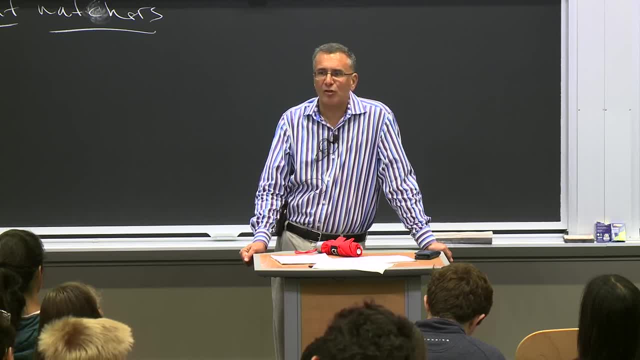 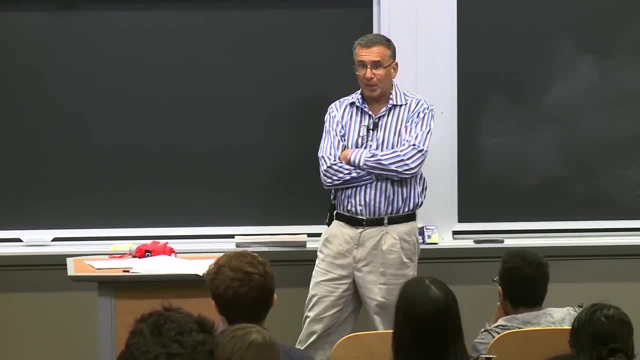 then they stop them and they gain the weight back. Dieting is incredibly hard and basically doesn't work, But a much more successful approach has been established by Weight Watchers. It's not the only approach, but it's been proven to be much more successful. 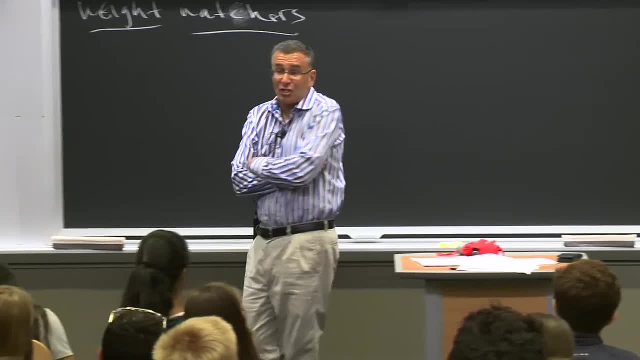 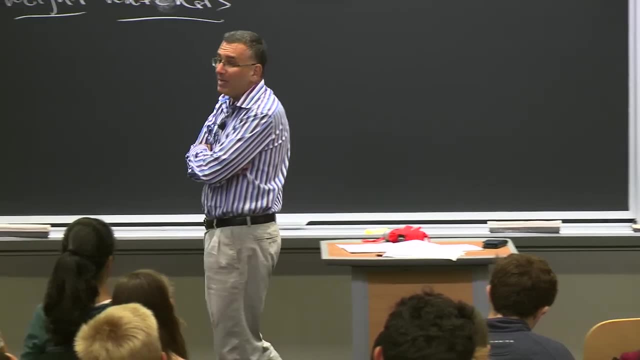 And essentially, what does Weight Watchers do? They set up a budget constraint and ask you to follow it. So, for example, they essentially assign point values to every good you might consume. You go on the website and everything in the world you might want to eat has a point value. 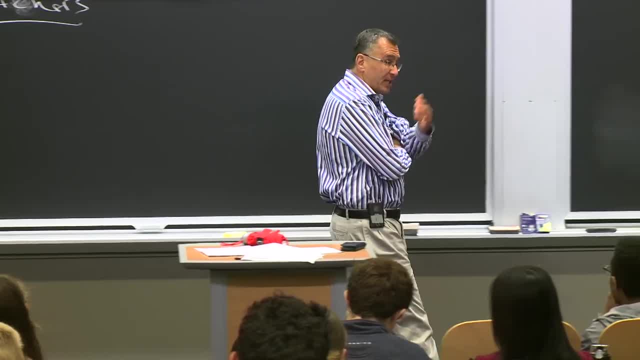 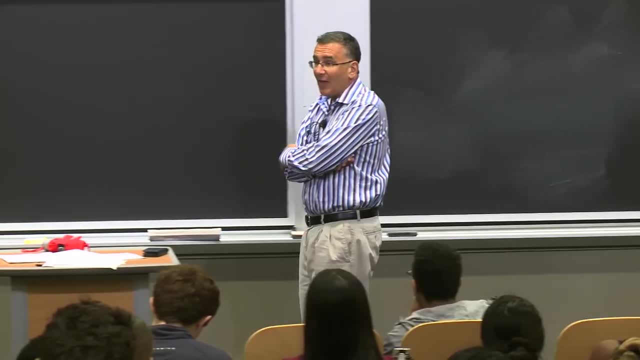 They then ask: well, what weight are you today? What's your age and gender? That stuff matters for weight loss. And what weight do you want to achieve? And they say: if you want to achieve a weight loss of X over Y days, 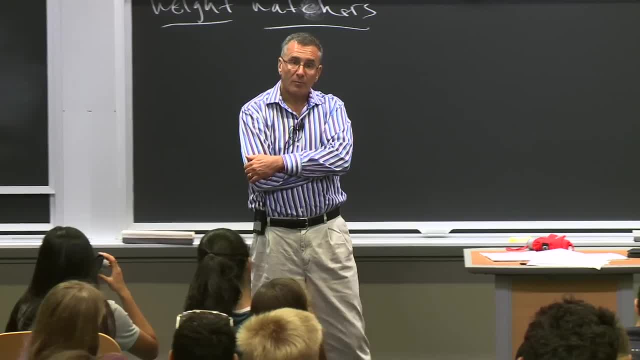 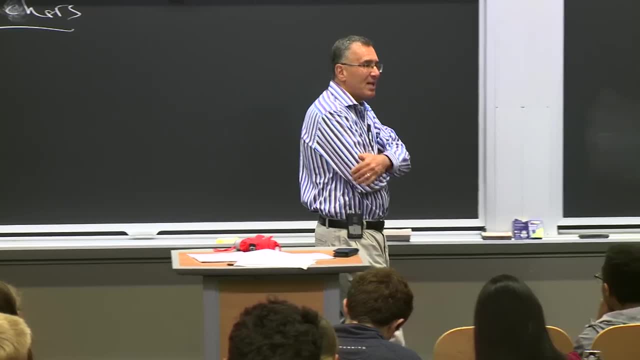 then you've got to limit yourself to Z points. So essentially, your goal is to lose weight. so we're going to give you the budget constraint. We're not going to tell you what to eat. That's why it's better than dieting. 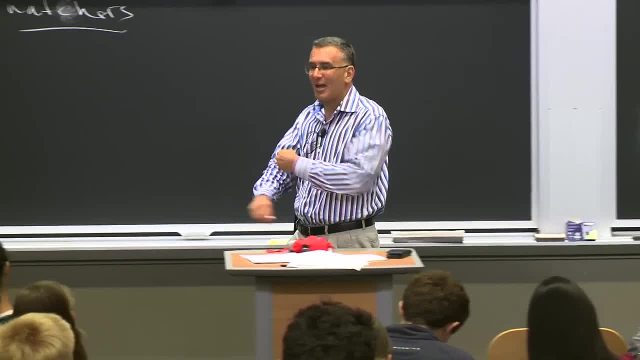 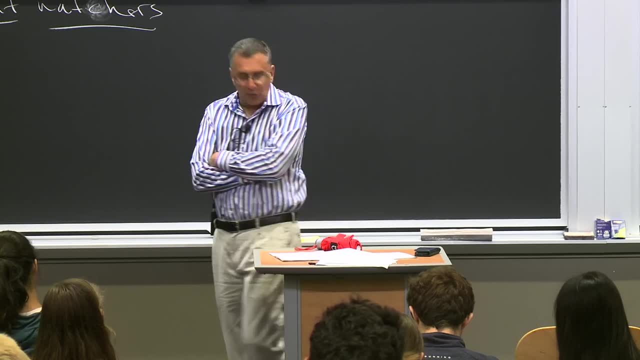 Because, once again, Adam Smith was right. People like to have choices, They like to let choice drive things. But we are going to tell you your total budget. So, for example, vegetables are like zero points, Snickers bars are like six points, et cetera. 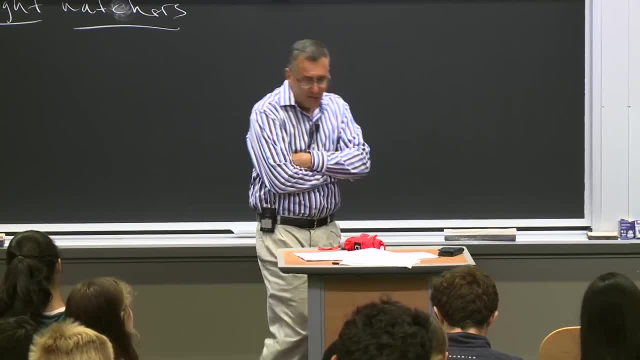 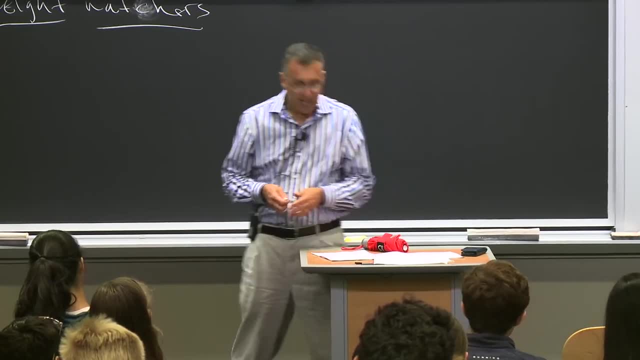 They have various point systems. So, for example, suppose your budget's 30 points, which would be pretty typical- Suppose you go to McDonald's for lunch and you get a number one. The number one at McDonald's is a Big Mac which has 14 points. 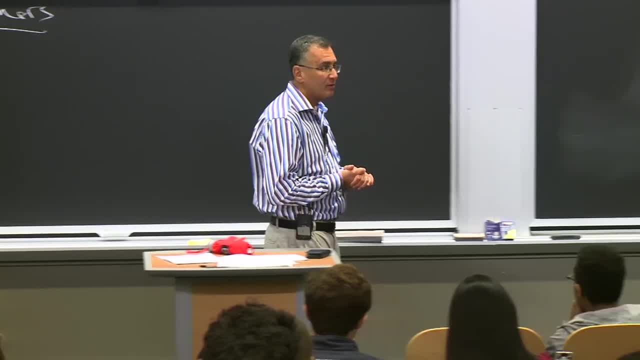 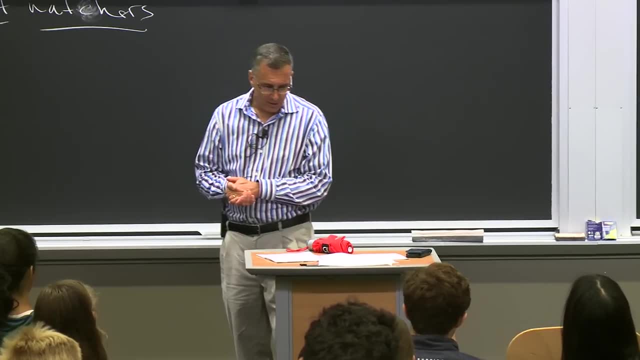 fries which have 10 points and a Coke which has six points. That's 30 points. and it's only lunch. You've blown your whole budget for the day on lunch. Now you could just get depressed and say: screw it. 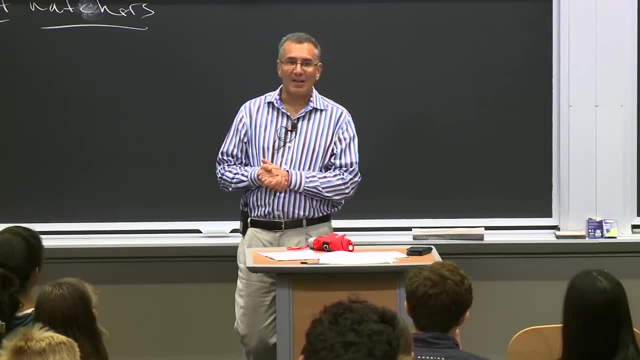 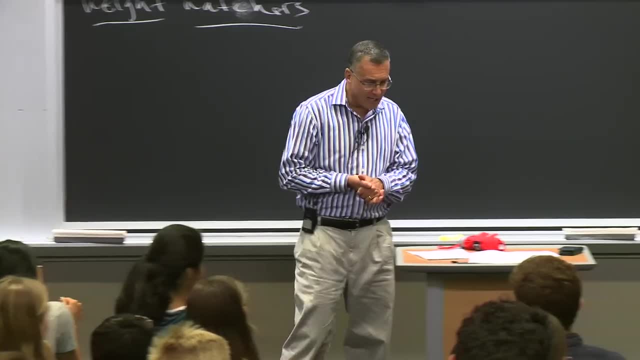 I'll just be fat. But clearly, looking around the room, you guys have not made that choice. Or you could look at the budget constraint and say, well, what else can I get? Well, it turns out you could get a 10-piece nugget, which is 12 points. 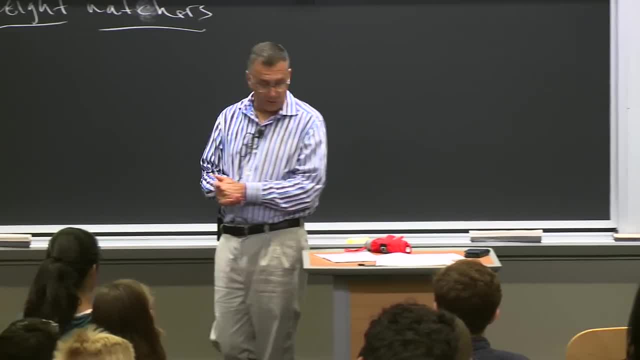 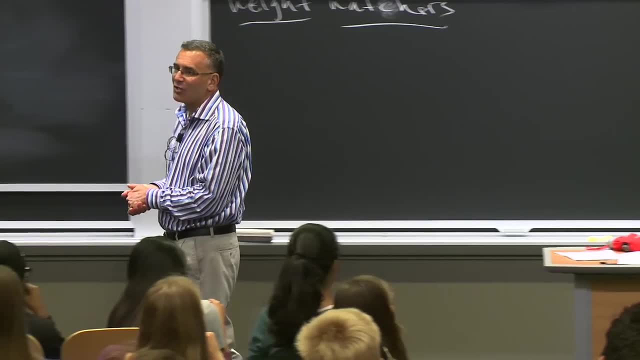 apple slices, which is one point, and a Diet Coke, which is zero points, for a total of only 13 points. Now, you have 13 points and plenty of room for dinner. Now, to be honest, anyone who tells you that? second of all, 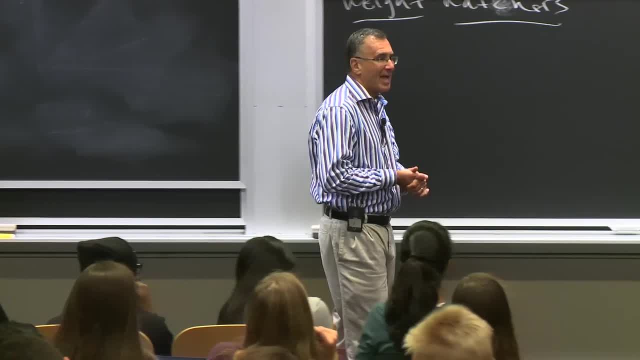 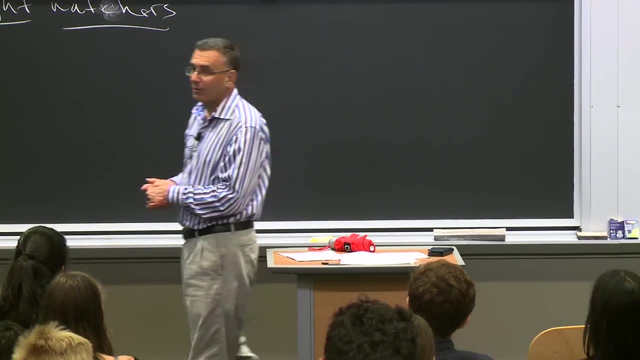 my lunch is good, because that first lunch is a liar. I'd much rather have a Big Mac and fries and a Coke than nuggets and apple slices and a Diet Coke. Give me a break, But I'd also much rather have dinner. So basically, this lets you make the trade-off by imposing a budget constraint. 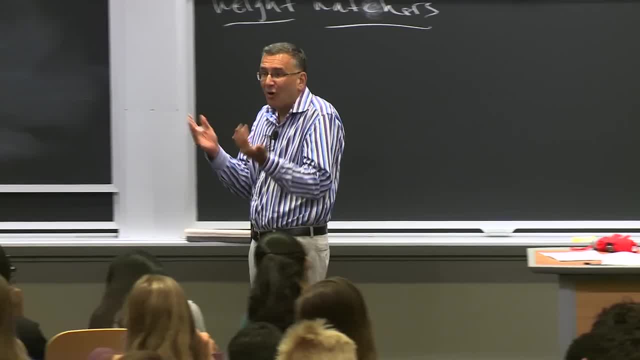 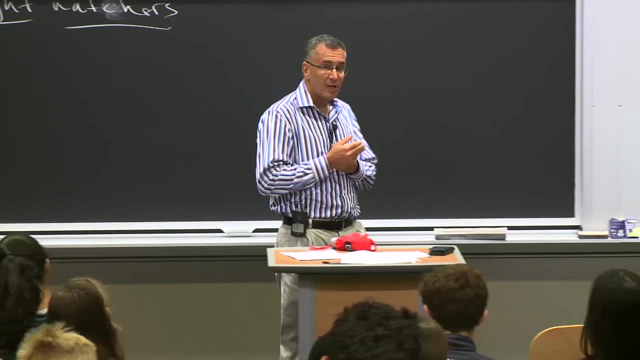 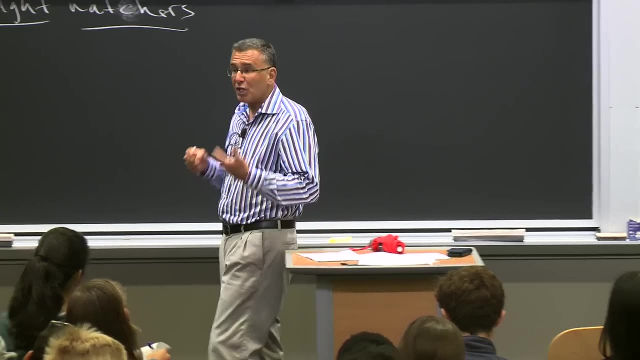 by setting relative prices across goods, The points are like noodles, They're not meaningful, They're only meaningful relatively. Let's just say relative price across goods and then it lets you essentially optimize across those various goods. So, budget constraints, essentially by setting up this marginal rate of transformation. 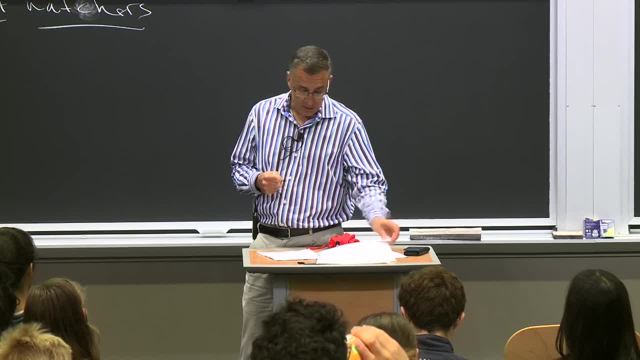 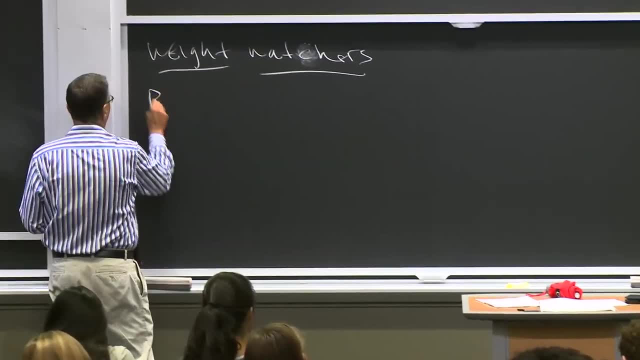 can help with a lot of kind of decisions in life. Questions about that Now: what happens if we shock the budget constraint? So we talked about constructing them. What about shocking the budget constraint? We're going to do a lot in this class of what we call comparative statics. 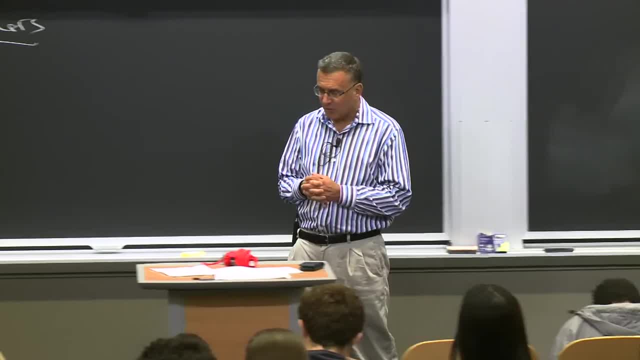 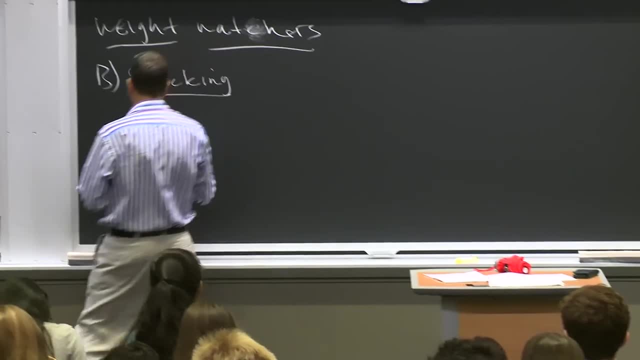 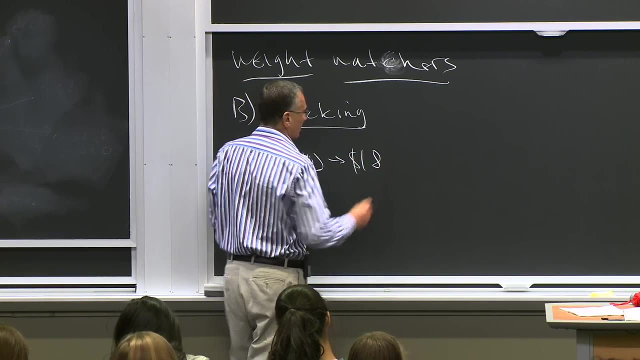 which is essentially making changes in one thing, one thing or another and seeing what it does to the system. So let's talk about shocking the budget constraint. Let's start first with a change in prices. Suppose the price of pizza goes from $12 up to $18.. 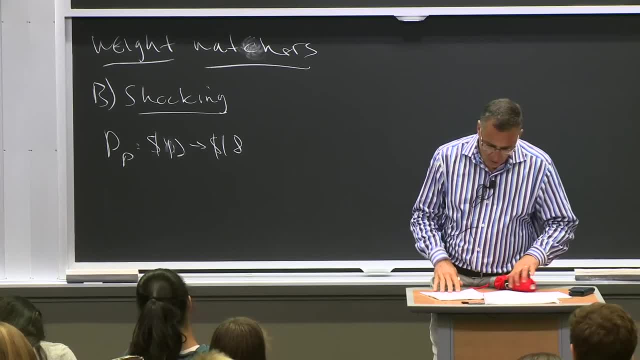 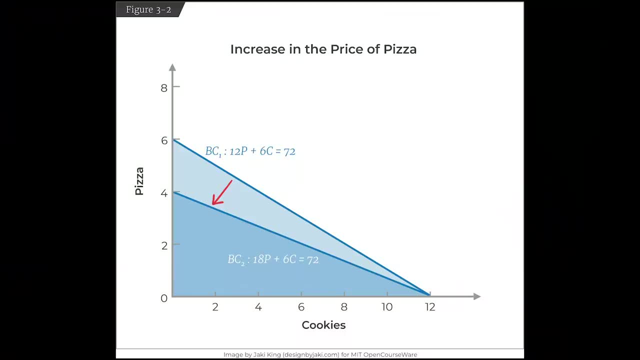 This is a really good slice of pizza. Well, what happens to the budget constraint? Let's look at Figure 3-2.. Figure 3-2 shows what happens, Your original budget constraint BC-1.. The equation of that line is: 12p plus 6c equals 72.. 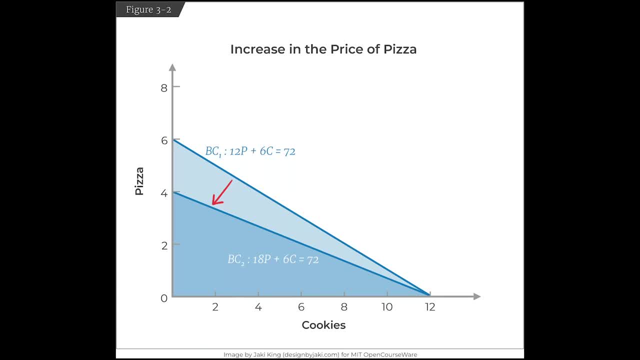 The price of pizza. the number of slices of pizza plus the price of cookies times the number of cookies equals 72.. Now the price of pizza has gone up. What that's done is that has pivoted inward your budget constraint to BC-2.. 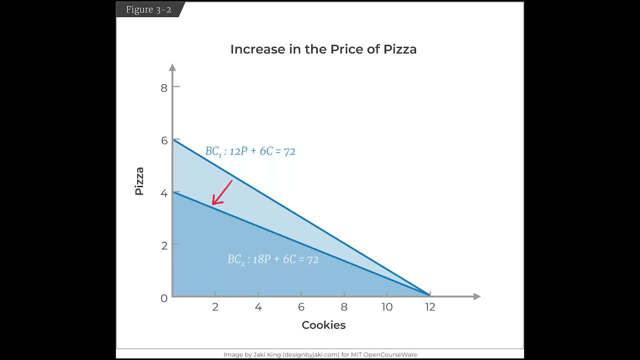 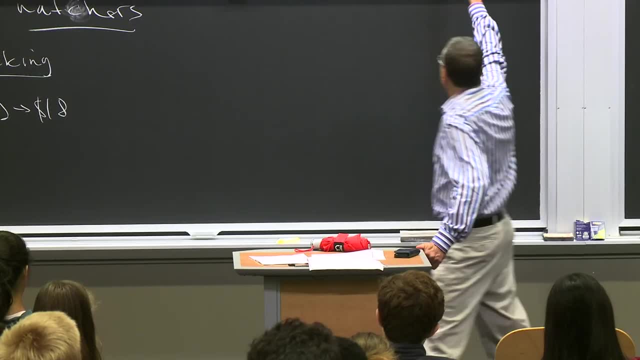 It has flattened the budget constraint, Because the slope, remember, is the ratio of the price of cookies to the price of pizza. Right, That's our ratio. Well, that ratio has just fallen. It used to be a half, Now it's a third. 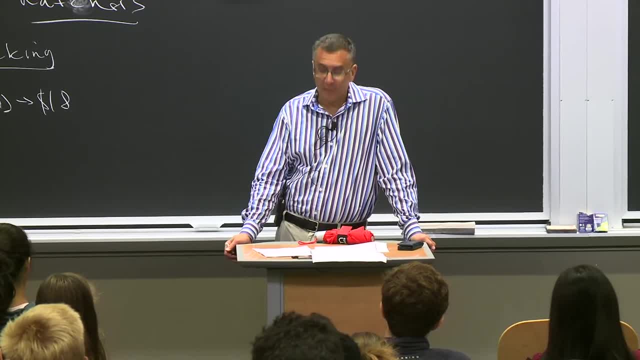 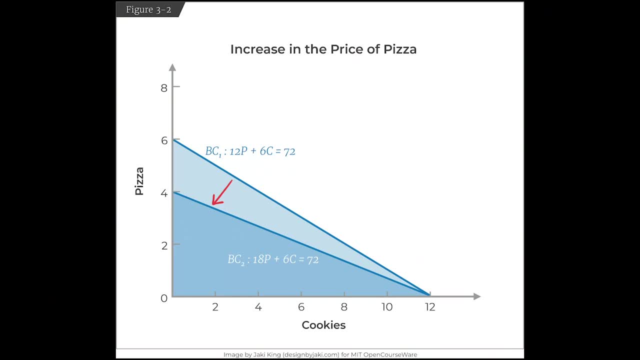 Negative a half. Well, it used to be a half, Now it's a third. So the slope has fallen from negative a half to negative a third. So what's happened is you can still have as many cookies as you had before. The y-intercept has not changed. 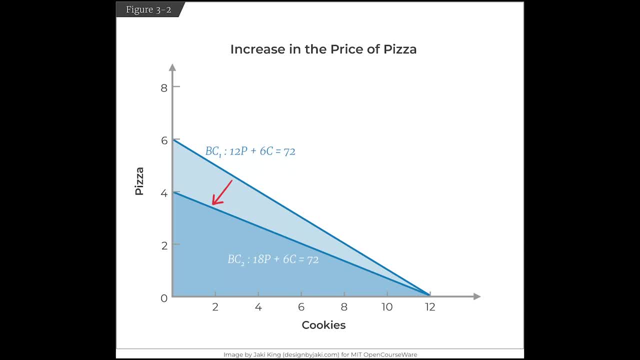 But you can have fewer slices of pizza. That's why it's a pivot, Because one price has not changed, only the other price. So it's a pivot inward. The other thing: here you'll notice, we have all these funny dots. 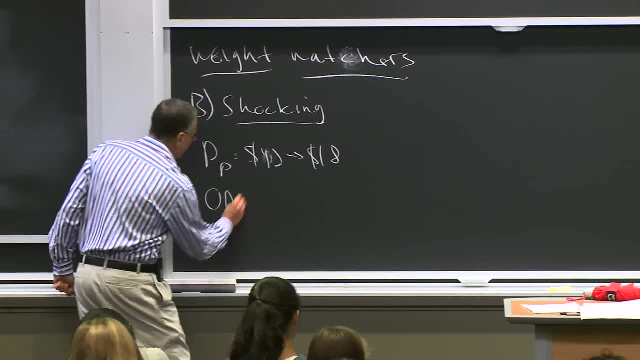 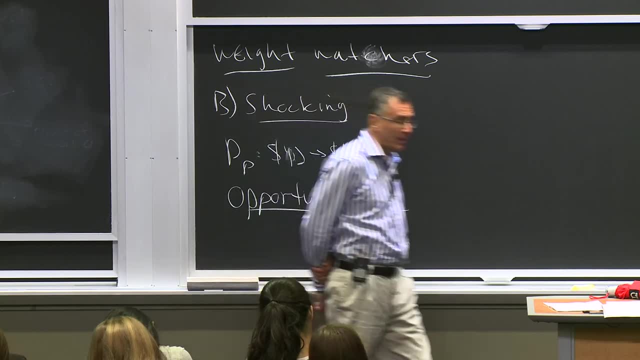 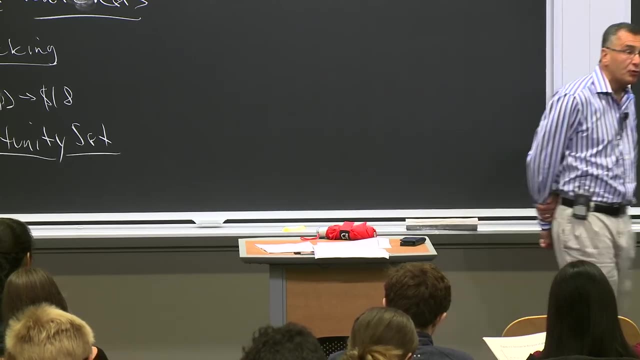 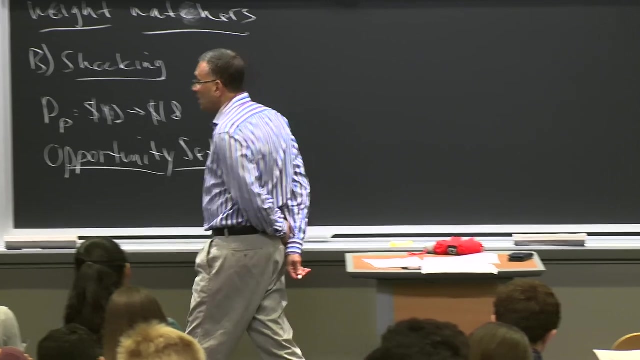 That represents what has happened to what we call your opportunity set. Your opportunity set, which is an important concept, Your opportunity set is the set of choices available to you, given your income and market prices. The set of choices available to you, given your income and market prices. 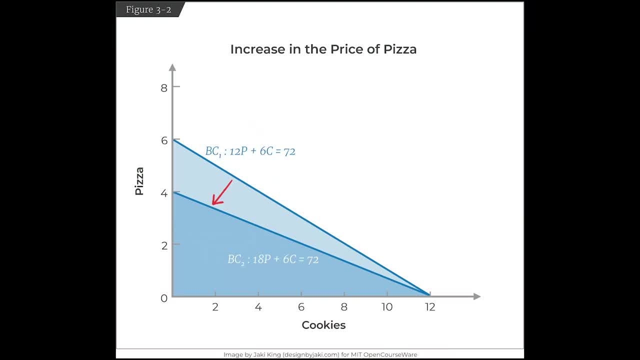 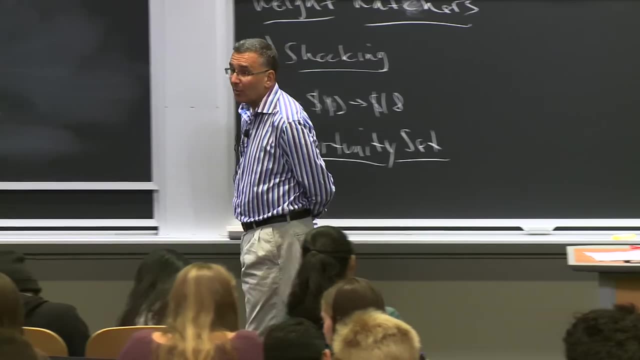 So your opportunity set initially was the black dots plus the red dots. Now your opportunity set has shrunk. Your opportunity set is now just the black dots. Given your income, you can now get less stuff, Same amount of cookies, but less pizza. 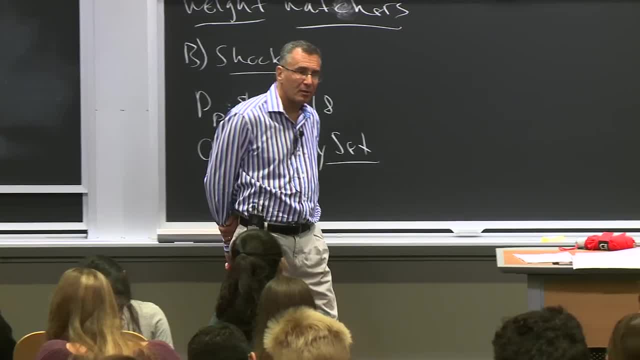 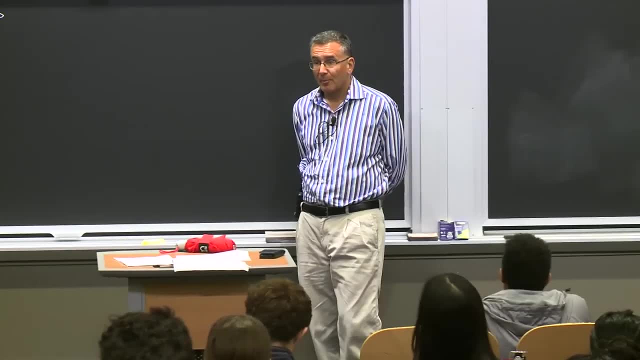 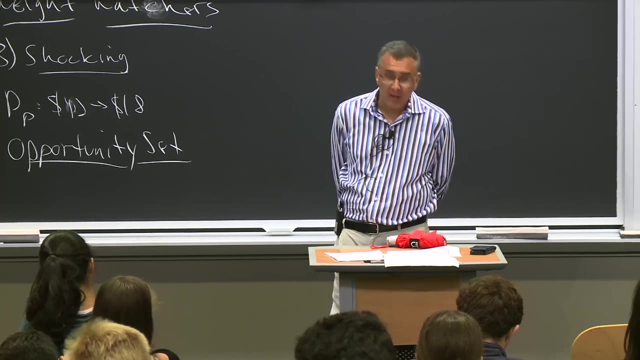 And you are worse off. Your opportunity set has shrunk, even though your parents still are sending you the same check. You are worse off because you can now buy less pizza with it. So that's what happens to the opportunity set when a price changes. 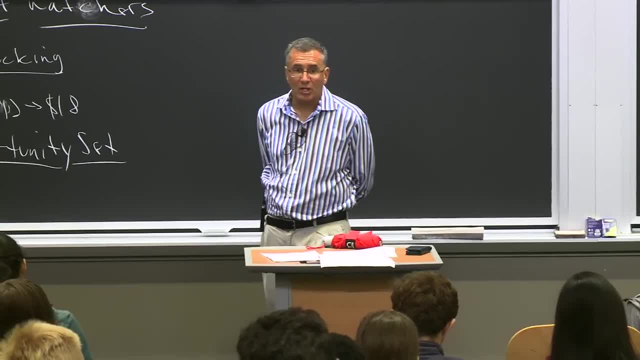 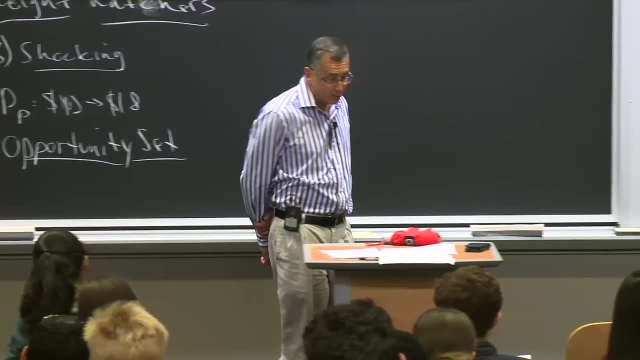 And likewise you should show yourself. the same thing will happen when the price of cookies change. In that case, you'll get an increase in the steepness of the budget constraint, But your opportunity set will still shrink. Now, what about? yeah? 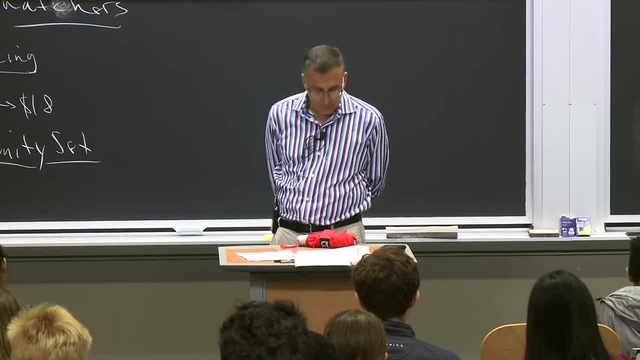 Don't we not care about all the dollars? Well, I'm not sure we're spending all their money. Well, that's a good point. We're going to come back to that. We haven't. We assume they're spending all their money. 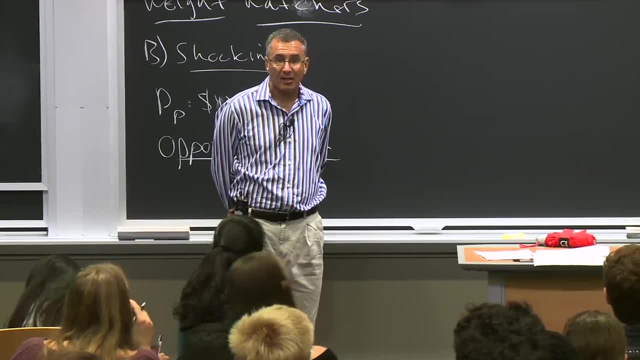 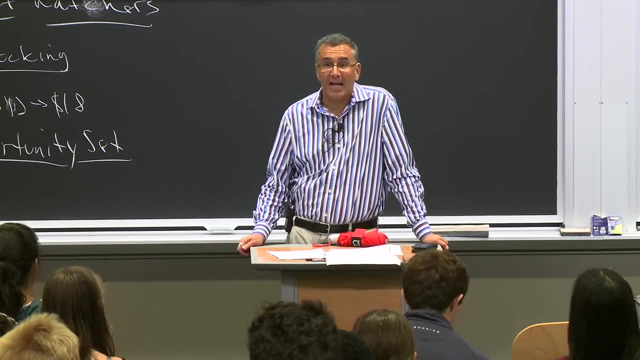 But it's just a way of representing. You can think of the line being lower as the same thing. So we just care about the area because it represents the set. But you're right, You could just focus on the line and say the line is everywhere lower. 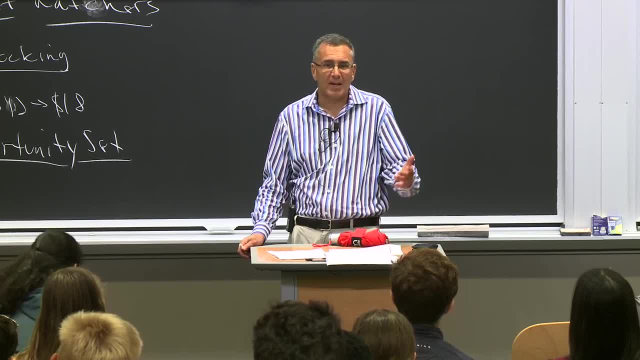 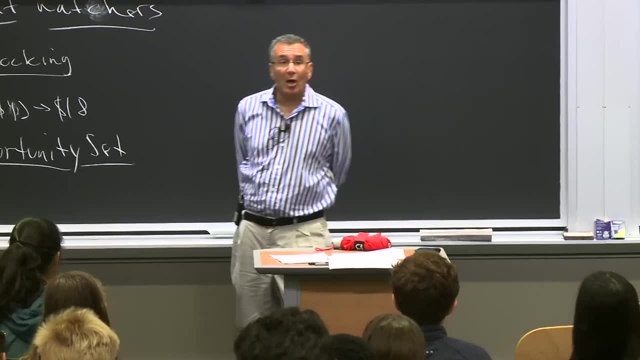 So they're worse off. That's another way to look at it, But we like to think about it as a set. It comes in handy later for various reasons. That's a good question. Now let's ask about a second thing: What if your income goes up? 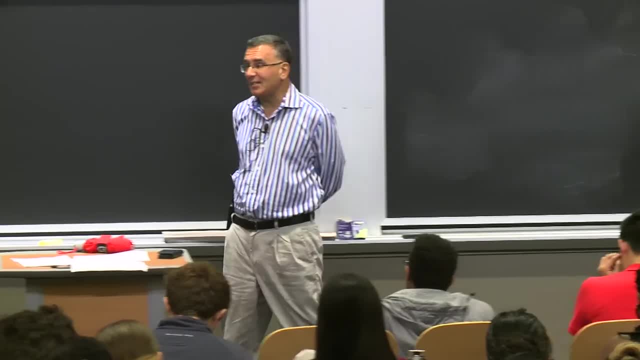 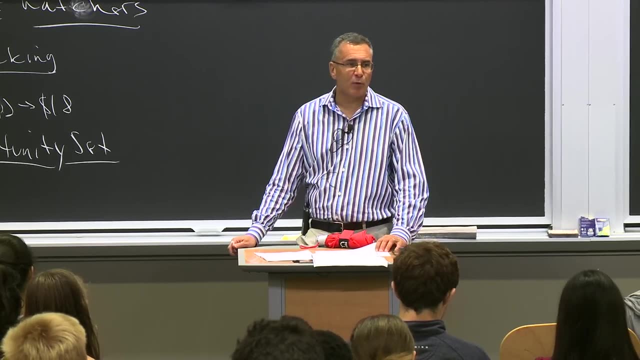 What if prices are back to 12 and 6, but your parents decide to send you more money? Suppose your parents are sending you less money. Turns out you haven't been paying enough attention to 1401.. Your parents are mad. They're monitoring you. 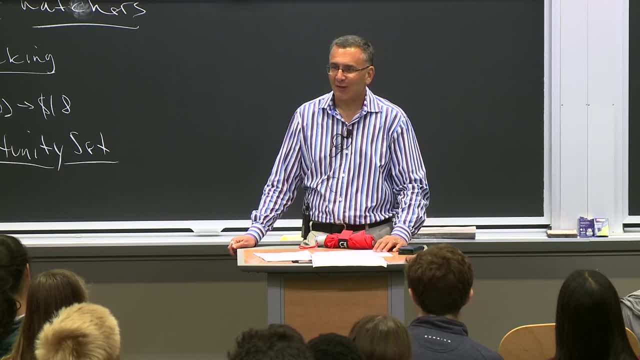 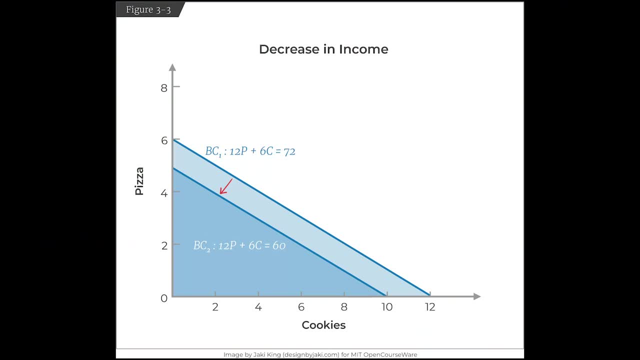 That's why we have the camera here. This goes directly to all your parents. OK, I'm sort of joking. And so let's say your parents cut your allowance to $60, OK. Well, What does that do? That's in figure 3-3, OK. 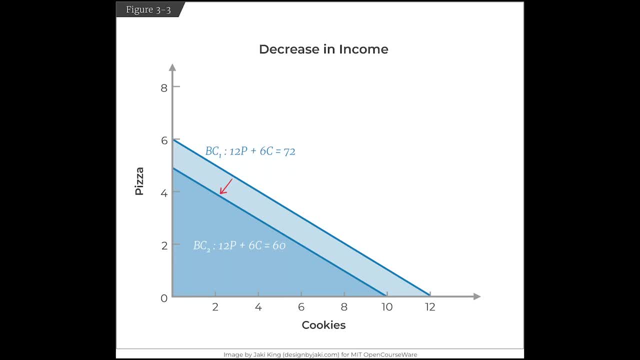 In figure 3-3,. the old budget constraint was that you get pizzas and cookies at a price of 6 and 12, and you get them until you spend $72.. Now you can only get them until you spend $60.. Now what we see is not a pivot in the budget constraint. 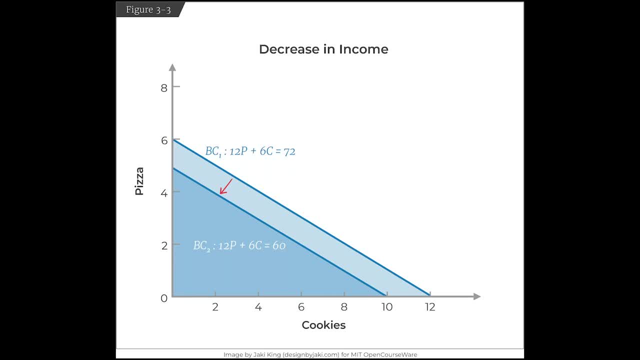 but an inward shift in the budget constraint, Because the relative price of pizza cookies has not changed. Therefore, the slope hasn't changed. The slope is dictated solely. You don't do anything to control the slope. The market controls the slope. OK. 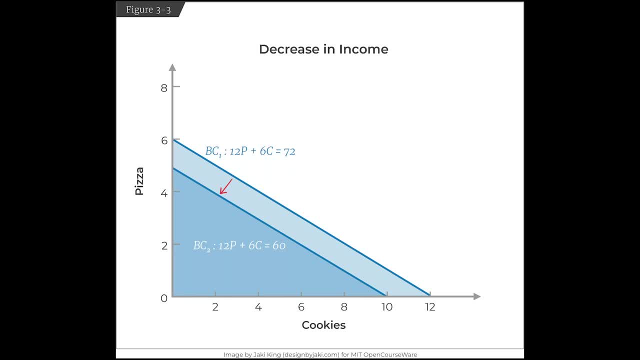 But you and your family control the level. OK, And the level has shrunk, So you're pivoting inwards. OK, And once again. now, instead of being able to buy, say, 12 cookies and 6 pizzas now, you can only buy, say, 10 cookies and 5 pizzas. 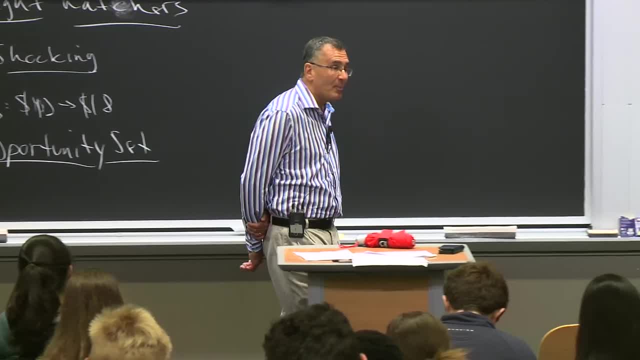 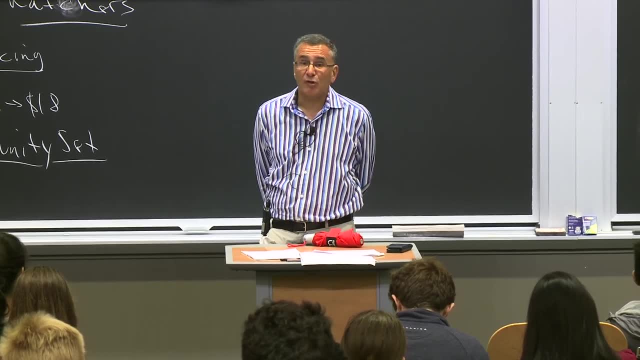 That's the most you can get, OK. So once again, your opportunity set has been restricted, but in a different kind of way, through this pivot inward. OK, So that's how we sort of manipulate these budget constraints, And we're going to come back to that next lecture. 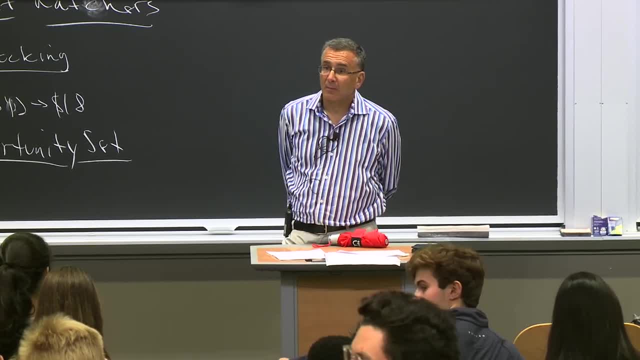 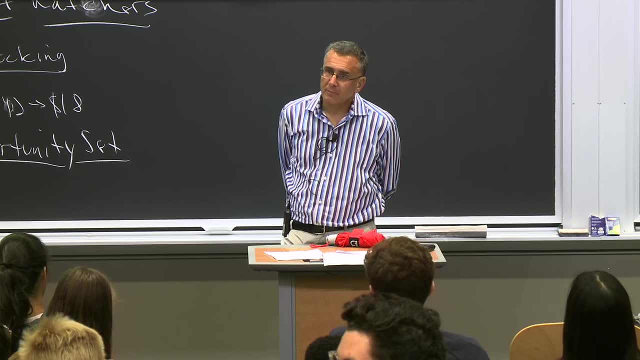 That will be important. Yeah, What are the differences between an increase in the price of pizza or a decrease in your budget? Is it more showing that the change in slopes doesn't really affect you if you're, say, buying more cookies and pizza, but in terms of if your budget as a whole? 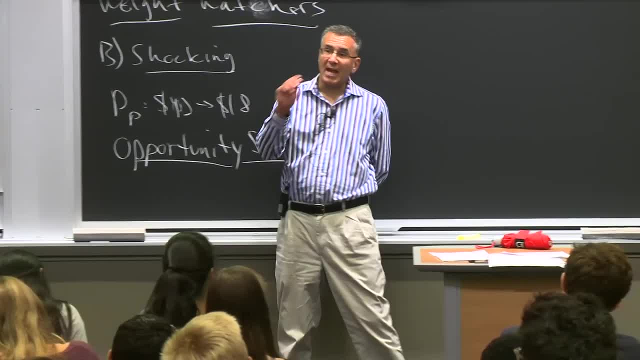 decreases, then it affects you overall. JONATHAN GRUBER- That's a great question And we're going to actually answer that question next lecture very explicitly. So hold on to that question and we'll talk about we're going. 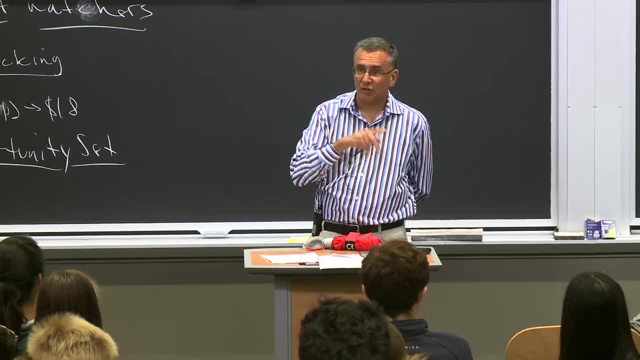 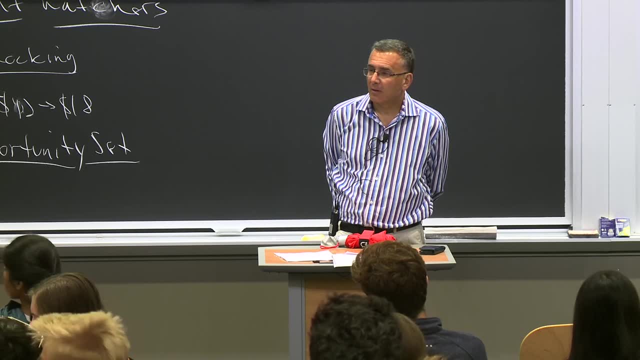 to compare explicitly. We're going to talk explicitly why income changes differ from price changes and what are the underlying mechanisms. Yeah, How do you determine your marginal rate of transformation? How do you determine your like say, it wasn't just pizza. 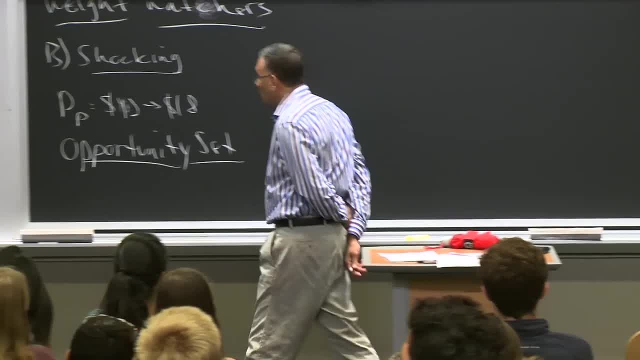 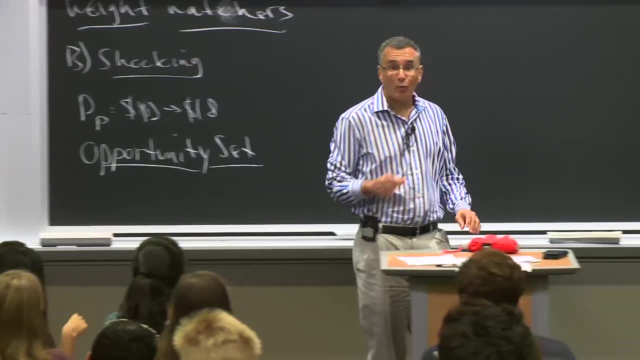 and cookies, but say it was more products. how would you determine that? JONATHAN GRUBER- Great, great question. So, as I said, we always are going to start with simplifying assumptions to make life easy. There's no reason that this couldn't be written. 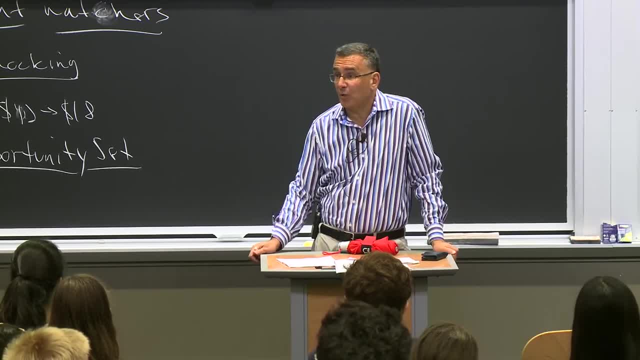 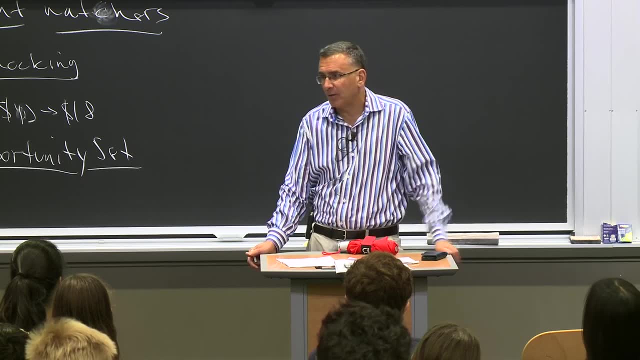 in three dimensions and you'd have relative marginal rates of transformation, rates at which you're willing to trade off various things. So you could just extend the math to more dimensions. It wouldn't add any richness, it would just make your head spin. 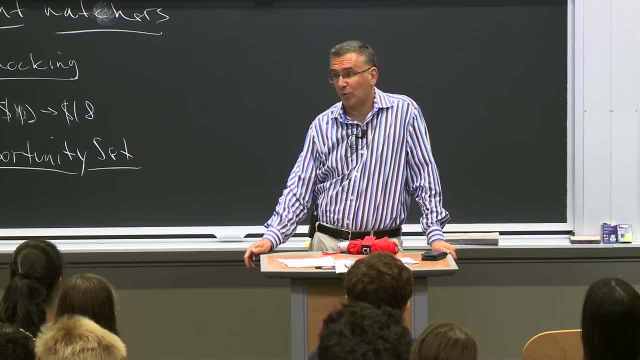 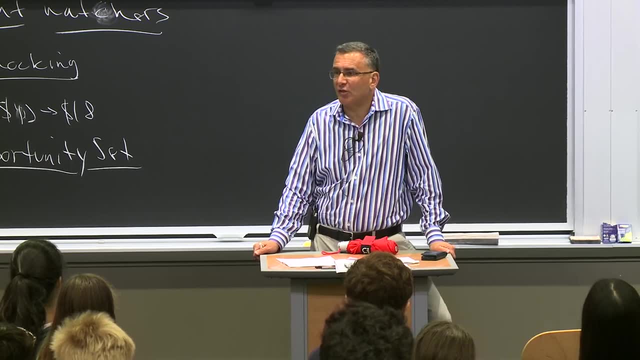 So all the basic ideas can come across with two goods, but it would be the same mechanics with more goods. You essentially, when we get to the constraint optimization, you essentially have more first order conditions in your constraint optimization. That's the way to think about it. 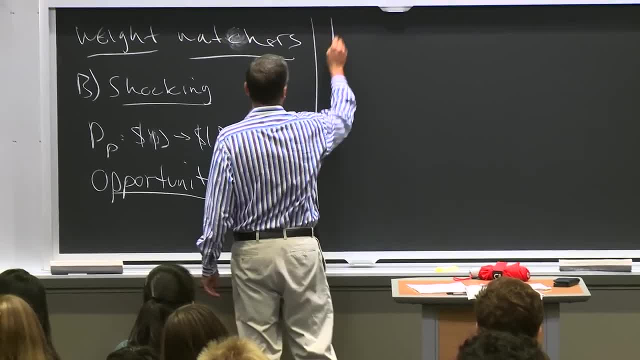 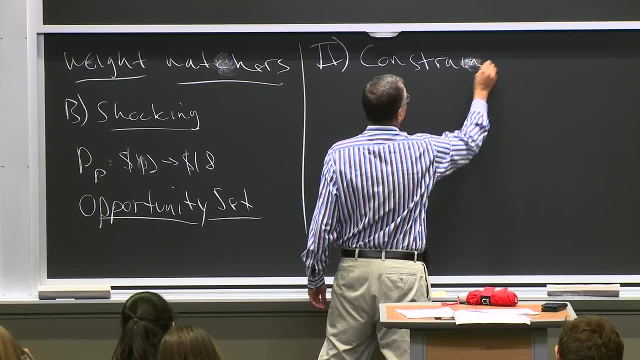 OK, so let's- actually- that's a great segue- Let's turn to the second part, which is how we use BUDGE constraints and the utility function we learned about last time to actually decide, describe how consumers make choices. So we're going to take utility. 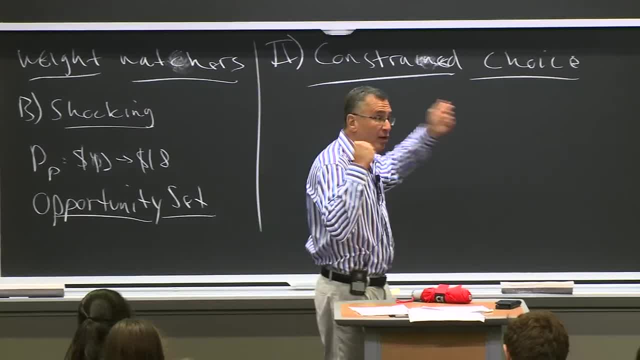 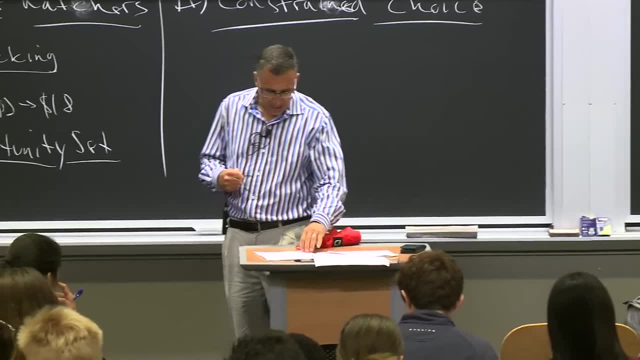 Remember I said last time, consumers are going to maximize the utility subject to a BUDGE constraint. Well, now we've taught you about utility. we've taught you about BUDGE constraints. let's put them together: How to consume, how do consumers put them together? 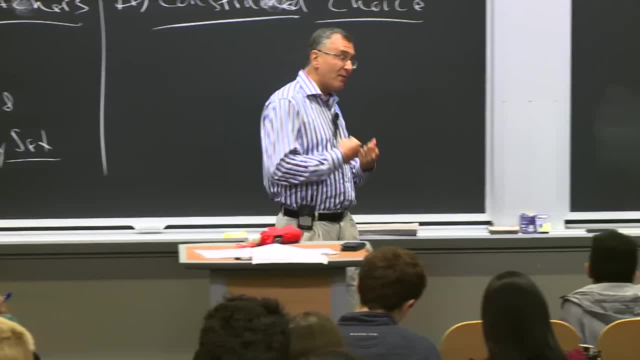 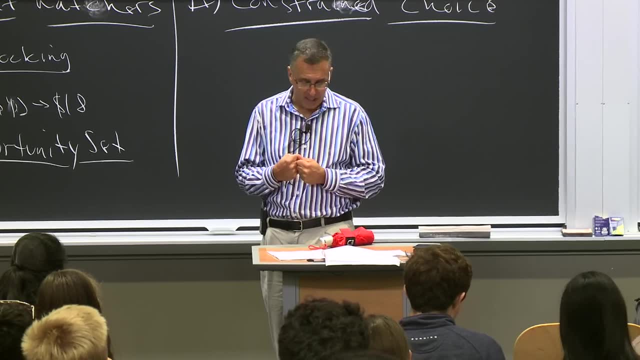 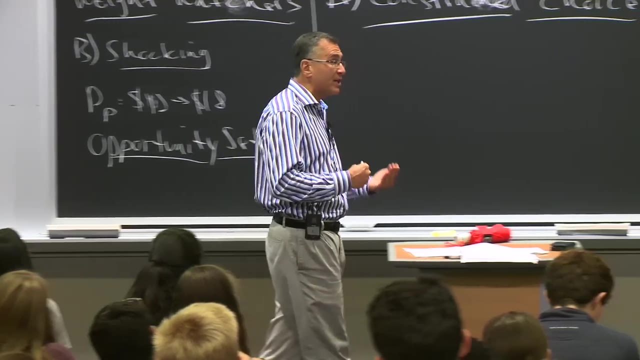 Well, graphically, the representation of preferences was our indifference curves. That represented people's indifference, with further out indifference curves made people happy. That was last time. So essentially what we're going to ask graphically is: what is the highest indifference curve you can achieve? 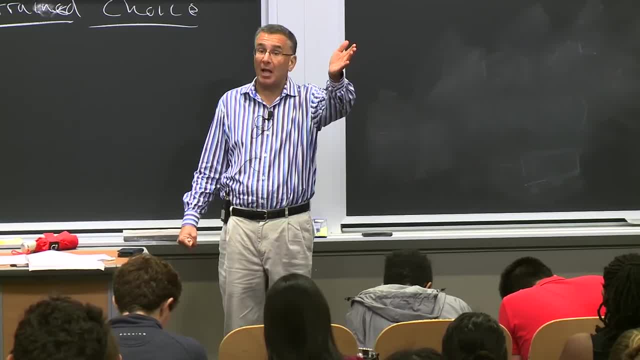 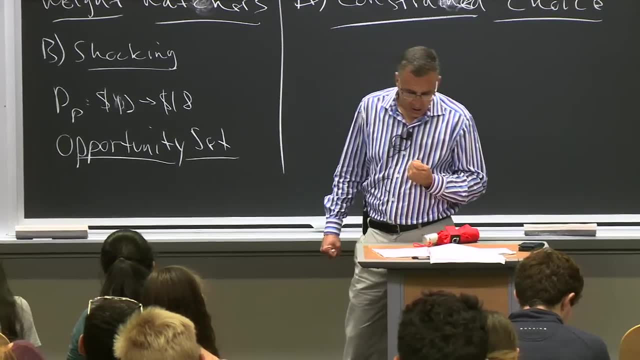 given your budget. We know you want to be the highest indifference curve possible by more is better, So we're simply going to ask: what is the highest indifference curve you can reach, given your budget? So let's consider the same utility from last time. 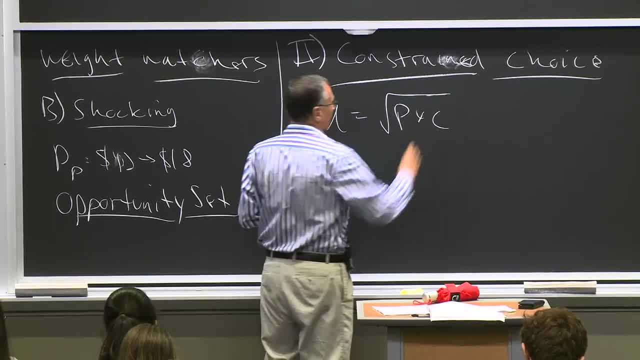 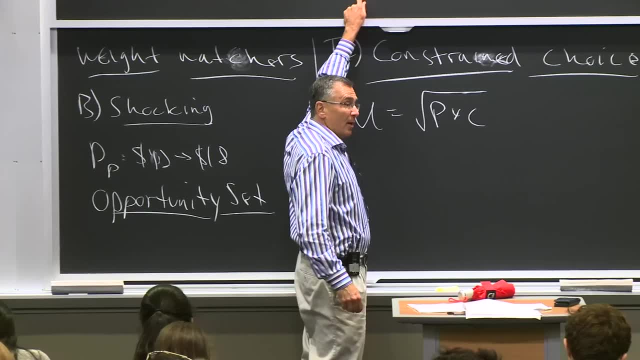 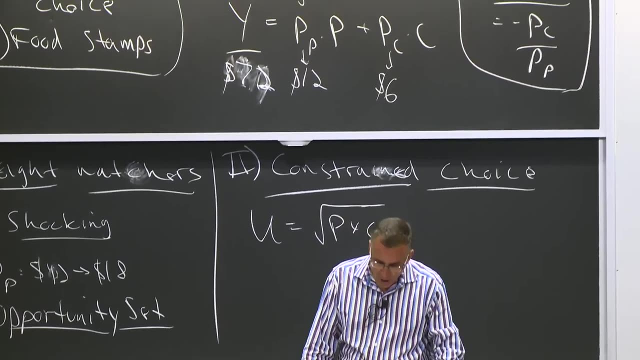 Utility is square root, It's the sum of P times C. And let's consider the same budget we wrote down up here: $72 income, $12 price of pizza, $6 price of cookies. And now let's ask: where can you go with that? 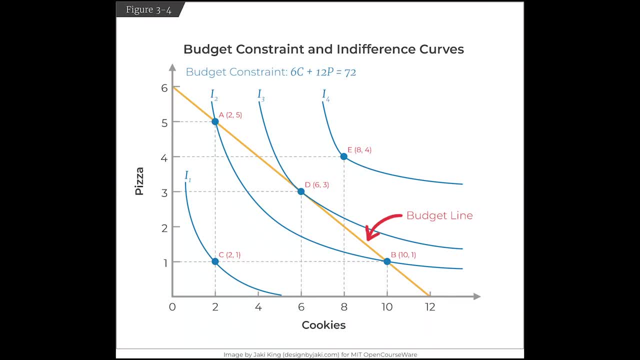 So let's turn to figure 3-4 and do it graphically. We'll do it mathematically in a minute. So in figure 3-4, you have our budget constraint, which runs from six pizzas to 12 cookies. 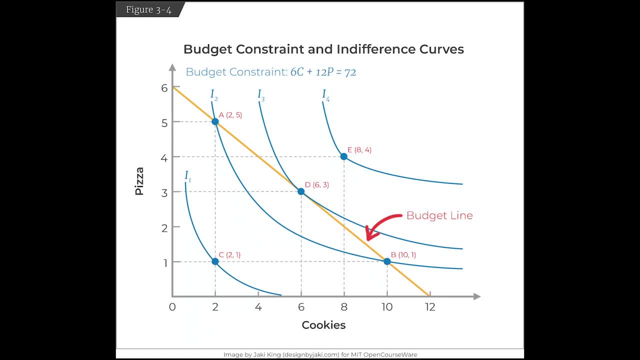 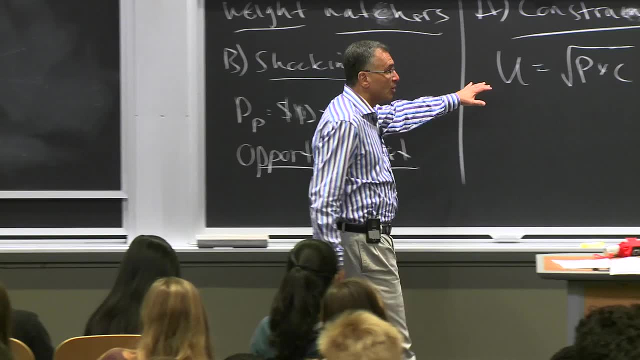 That's the original budget constraint And you have a series of indifference curves And these indifference curves- i1, i2, i3, i4, they all come directly from this utility function. So, simply, I've solved this utility function. 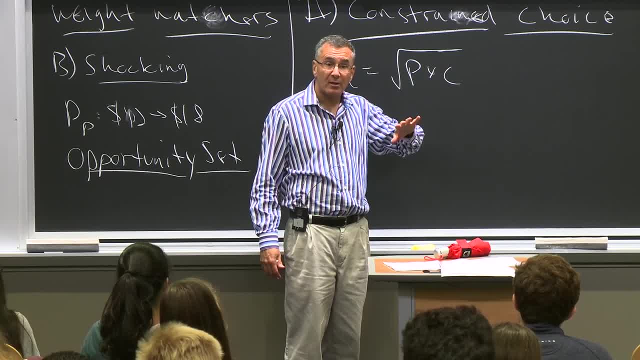 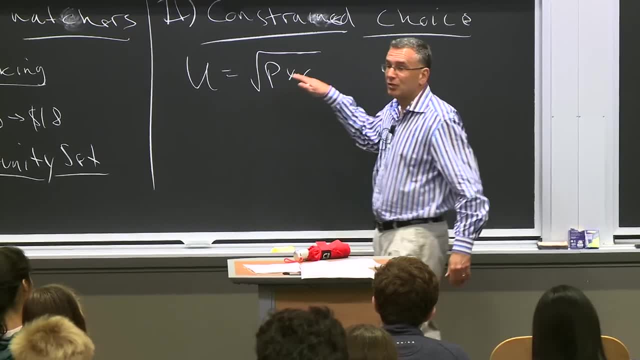 I'll talk about the math in a little bit. You'll do more math in section on Friday, But essentially we'll show you you'll derive on Friday how you take this utility function literally, can draw the indifference curves from it. But for now take my word that these indifference 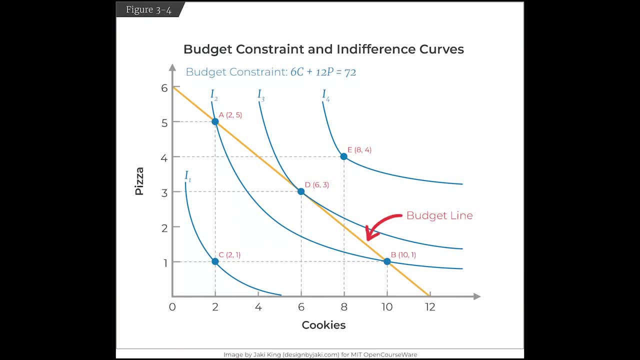 curves represent this utility function And what we see is that point D is the furthest out indifference curve you can achieve while still meeting your budget, while saving your budget constraint, And therefore we say that the optimum, graphically, is the tangency between your indifference curve. 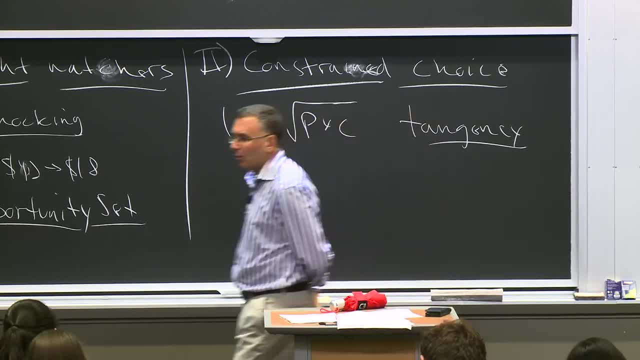 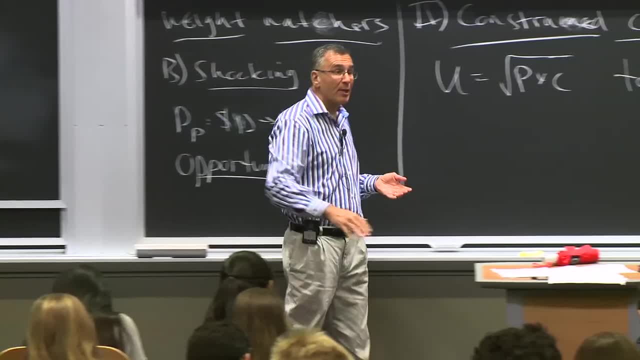 and your budget constraint is the optimal constrained bundle. You see how I brought. Last time we talked about further out indifference curves make you happier. Today we talked about the fact you're limited by your budget, So the furthest indifference curve you can get to. 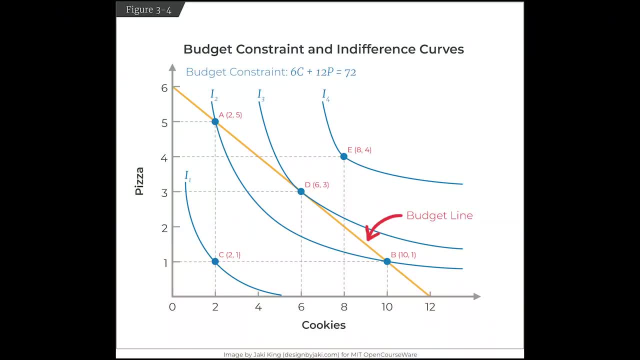 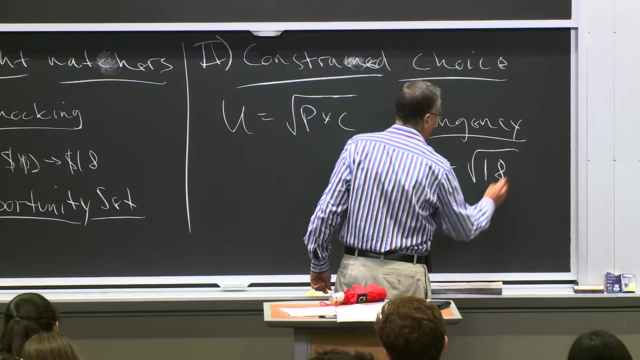 is going to be definitionally, at the tangent of the indifference curve and the budget constraint And once again that gives you- we don't want to measure utils, but just for mathematical purposes that gives you utility at that tangency of square root of 18.. 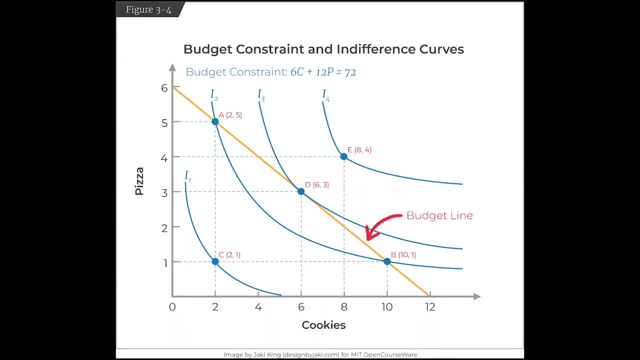 At that point you are choosing Six cookies and three pizzas. That is the choice you are making. That is the best off you can get given your budget. And to see this, let's talk about some other points and why they're not better. 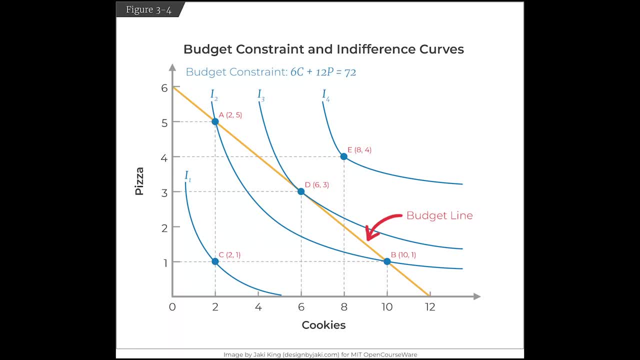 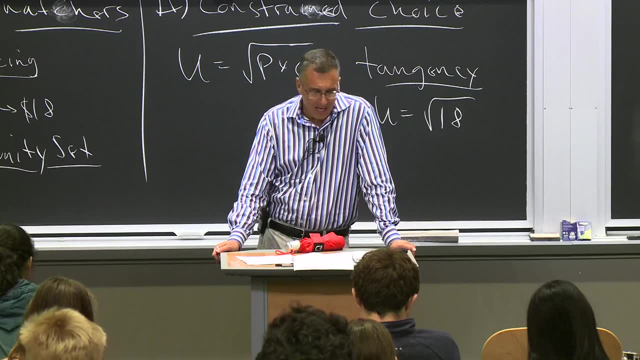 Let's talk about point A. Why isn't point A better? Why isn't it better to have two? Maybe you like cookies a lot and don't like pizza a lot and don't like cookies that much. How can we say that point D is better than point A? 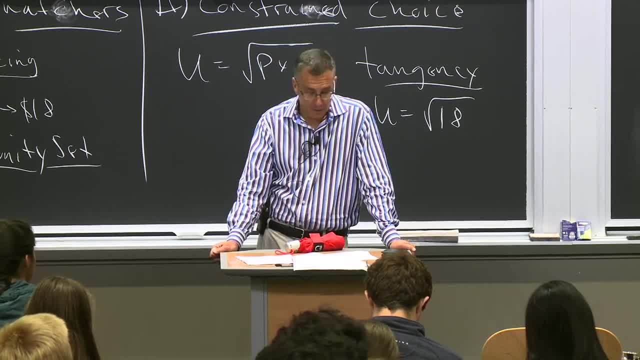 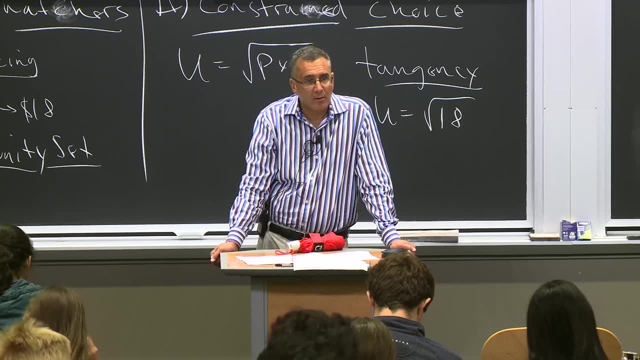 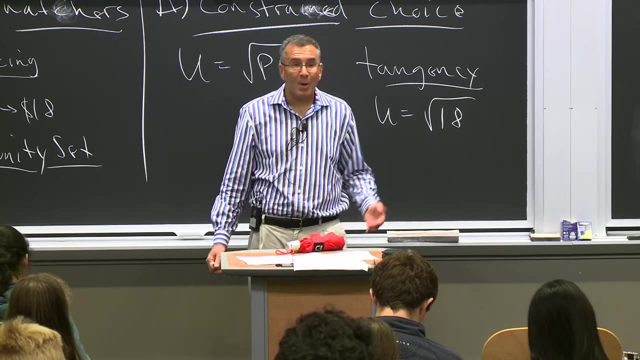 Yeah, It's on a higher indifference curve. So point D dominates point A because it's on a higher indifference curve. Well, fine, Same person. By that logic, why not choose point E? Yeah, you can't afford it. So the bottom line is: you can see graphically: 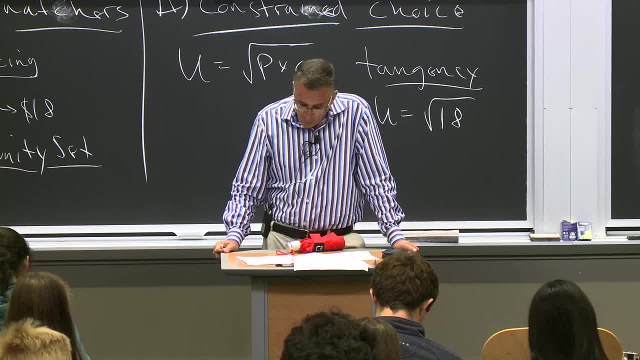 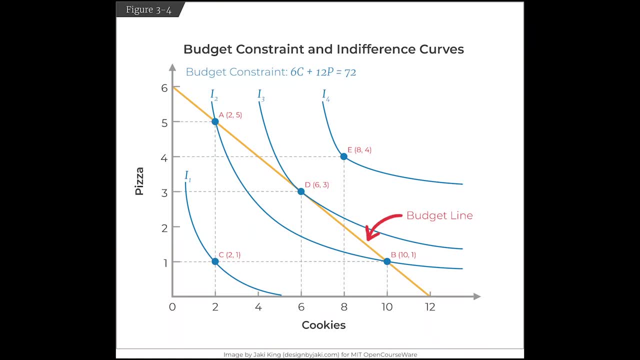 why the tangency is the best you're going to do. Likewise, point C you wouldn't choose. Point C has the same slope. It has the same slope. The slope has point D, In other words the slope's minus 1 half at point C. 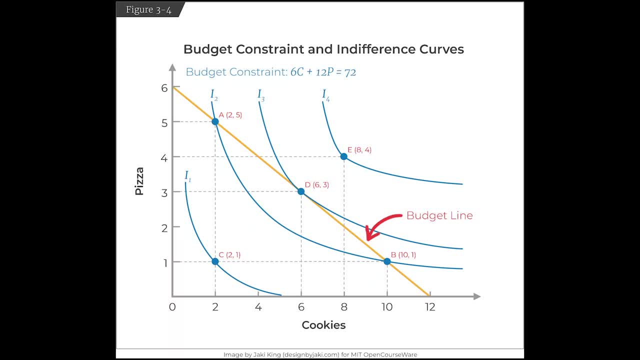 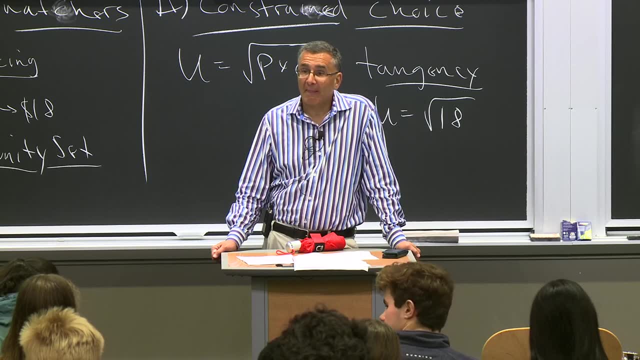 You drew a line tangent to point C. The slope will be minus 1 half, just like it is at point D, But you wouldn't be spending all your money, So you wouldn't choose that point either. Yeah, What if you have discrete indifference curves? 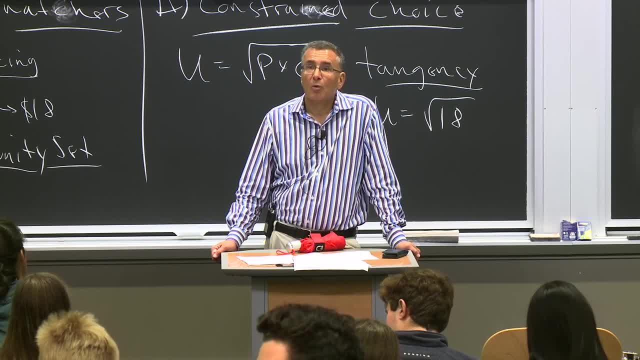 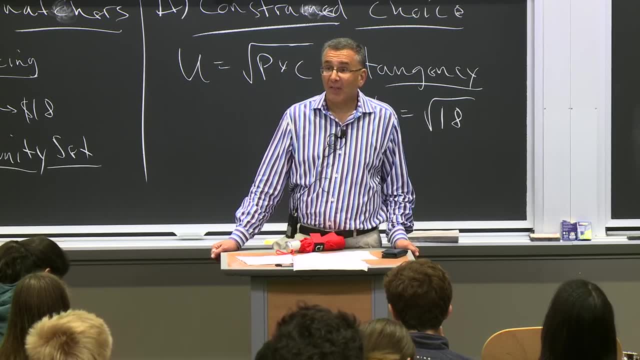 so there is none that hit the tangent. Do you just go for one? that's the most tangent? again, We're going to come to it. First of all, we're not going to have discrete indifference. Well, we could have lines And the lines could end up. 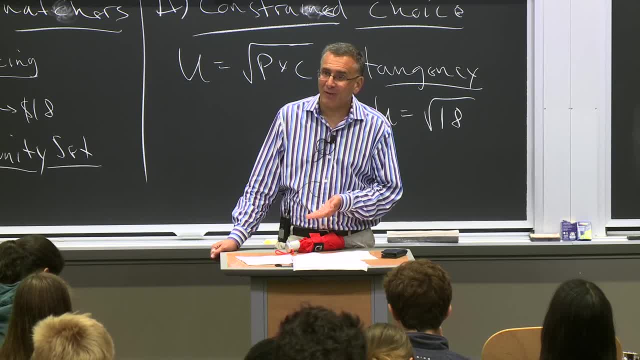 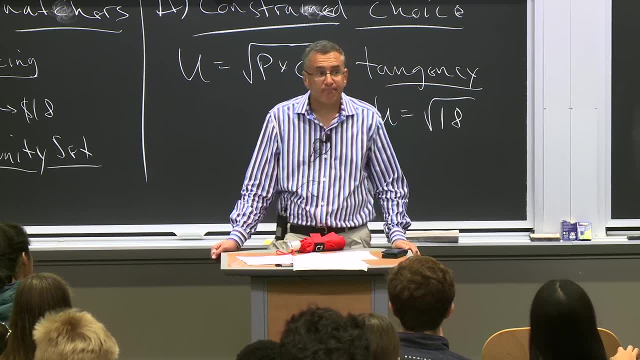 You could end up Lying along. And you could end up lying along a budget constraint, for example, Or you could even have utility functions which touch a budget constraint at one extreme or another, And we'll talk about those cases. Yeah. 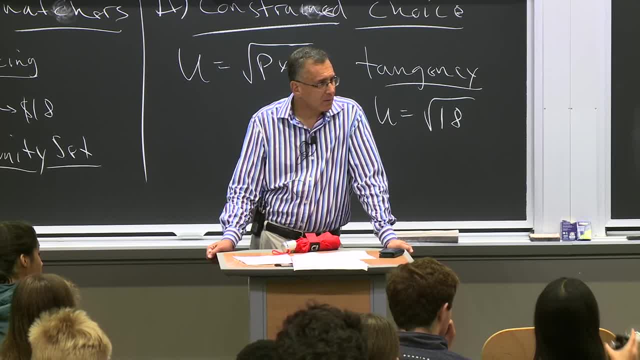 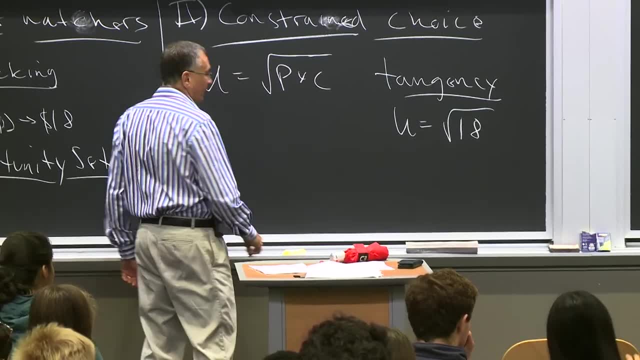 utility function to optimize as a budget constraint. right Yeah, Isn't this just a logger on? Well, let's come to the math. then Let's come to the mathematical derivation. So that's the graphics, Let's come to the math. 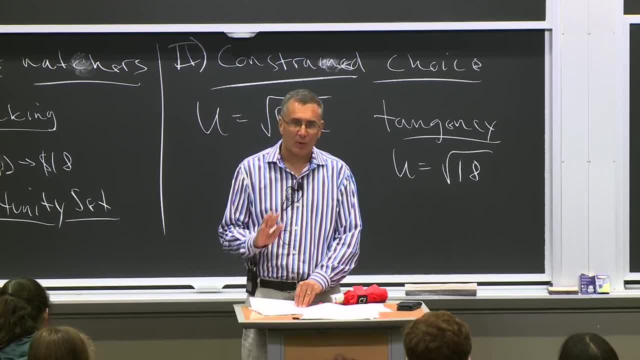 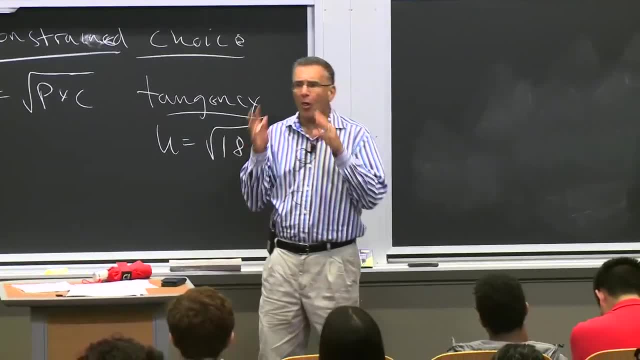 Now always a bit of a tightrope act when I'm doing math up here on the board, So bear with me, OK, But the key thing Is the math of constraint. optimization is all about the marginal decision. Remember, it's hard to say how many cookies you want. 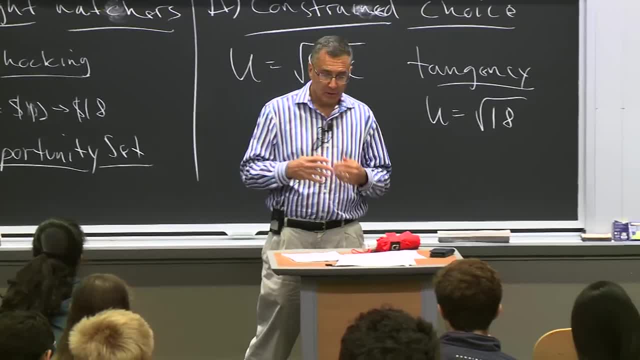 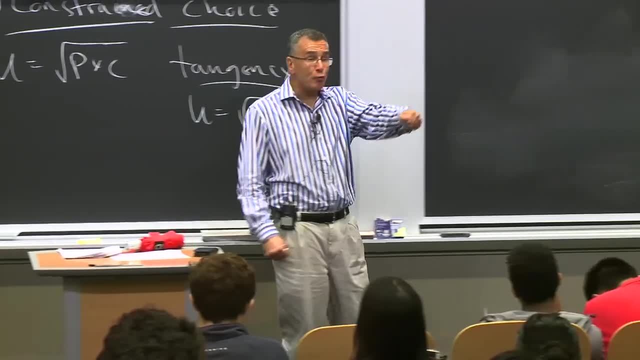 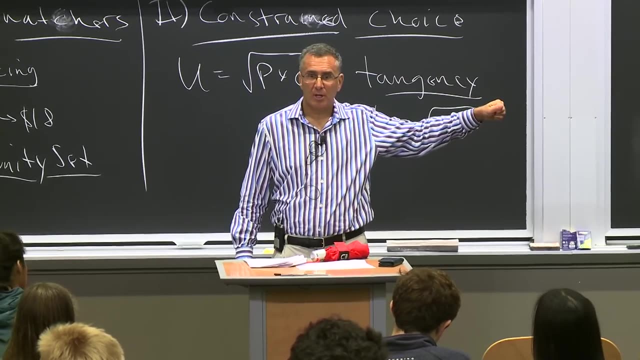 It's easier to say: should I have the next cookie? OK? It's about constraint, optimization, And what we want to ask is: we essentially want to compare. how do you feel about trading off pizzas versus cookies versus what? will the market let you do? 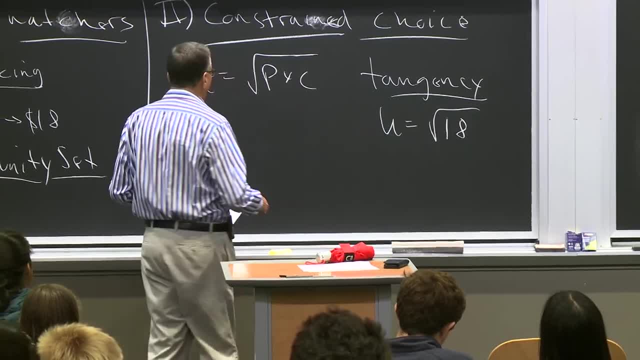 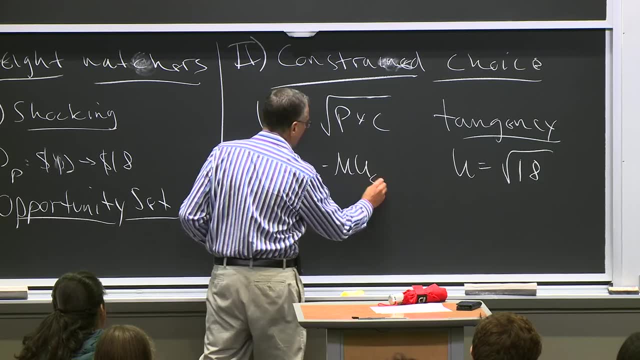 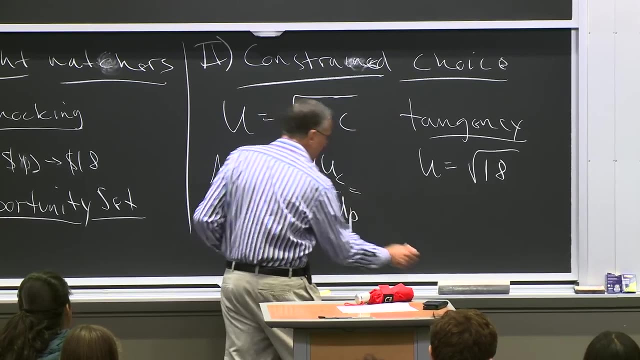 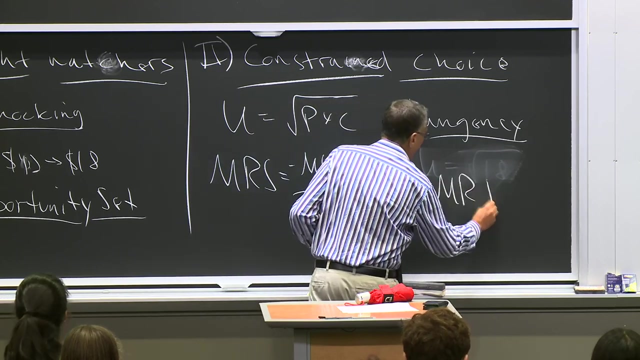 instead of trading off pizzas versus cookies. That is So. the optimum is going to occur when we set your marginal rate of substitution, which, remember, we defined as minus MUC over MUP, equal to your marginal rate of transformation, which we defined as minus PC over PEP. 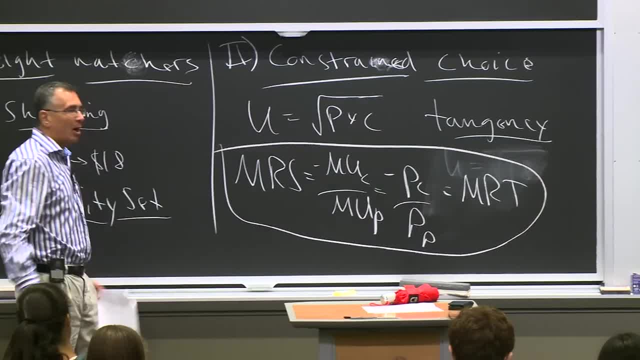 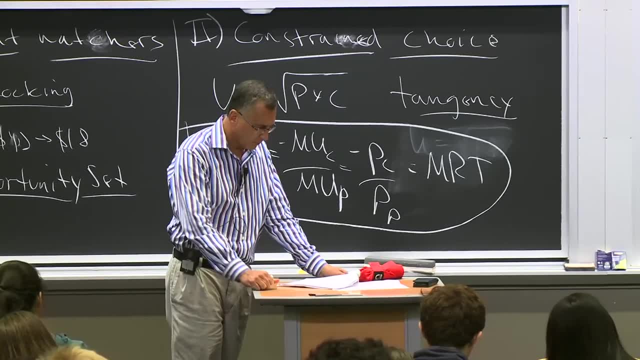 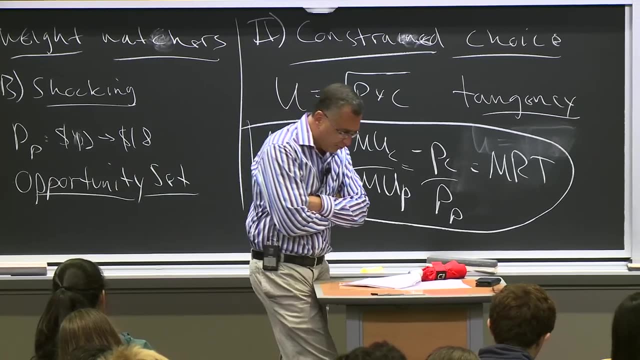 And this is the fundamental equation. It's going to give you the ratio of consumer choice. If you understand this equation, you can solve virtually every consumer choice problem. we'll give you That, basically, at the optimum, the ratio of marginal utilities equals the ratio of prices. 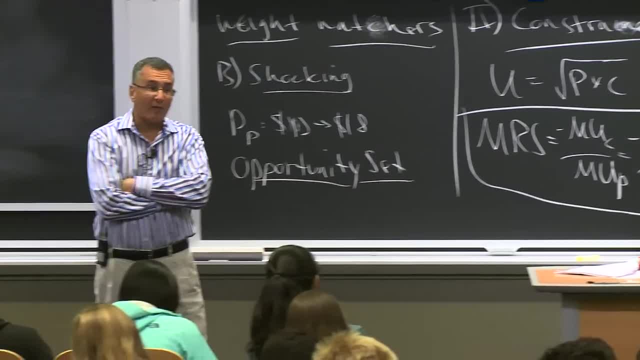 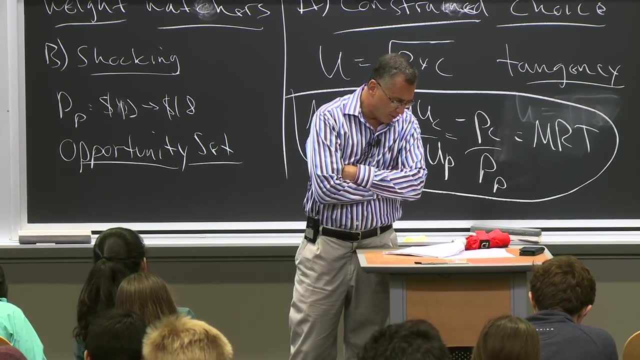 That is the rate at which you want to trade off pizza for cookies, is the rate at which the market will allow you to trade off pizza for cookies. OK, Basically, it's saying the ratio of the benefit of the market, the benefits. think of this as the benefits. 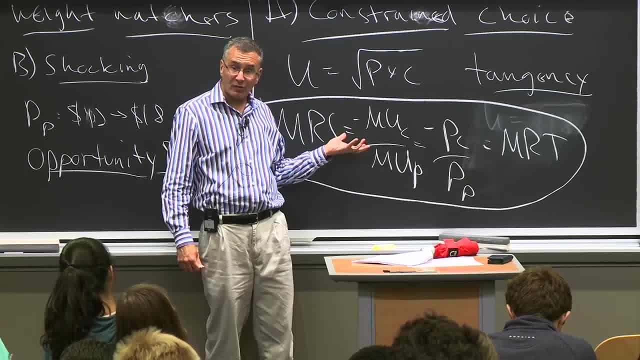 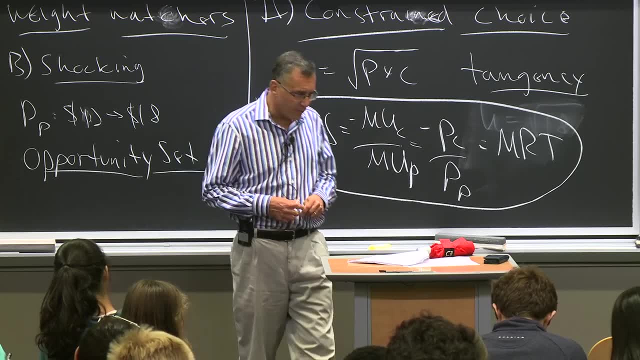 and this is the cost. Think of the MRS as the benefits. It's what you want. MRT is the cost. It's where you're constrained. You want to set the ratio of the benefits equal to the ratio of the costs. 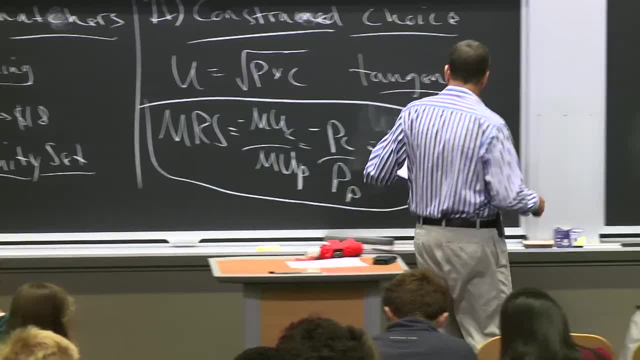 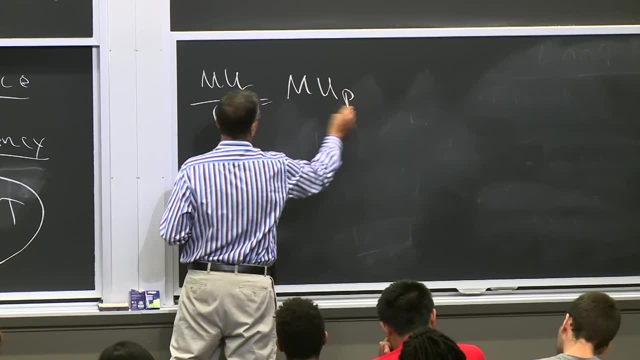 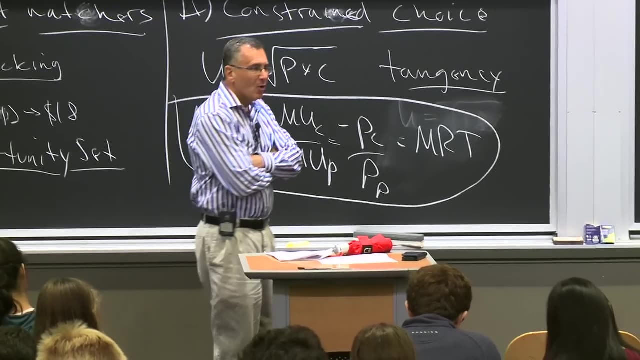 OK Now, I find it actually easier to think of it this way: If you just rearrange terms, you can write it as: MUC over PC equals MUP over P sub P. I like this way of writing it because I call this the bang for the buck equation. 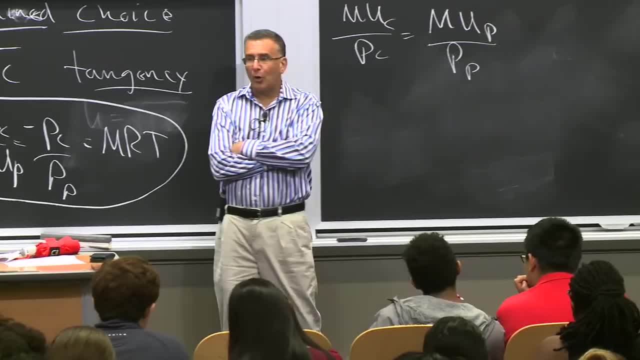 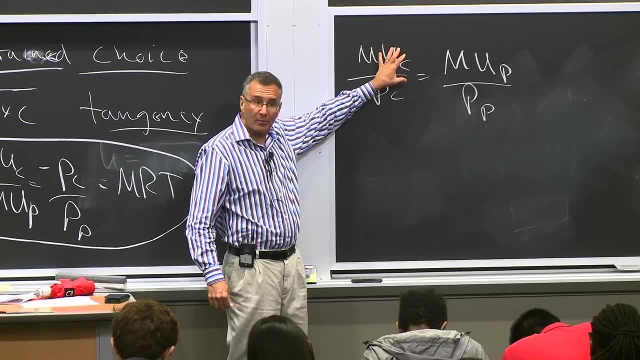 What this is saying: your marginal happiness per dollar should be equal. This is sort of the happiness per dollar spent on cookies. This is the happiness per dollar spent on pizza, And you want those to be equal. You want the bang for the buck. 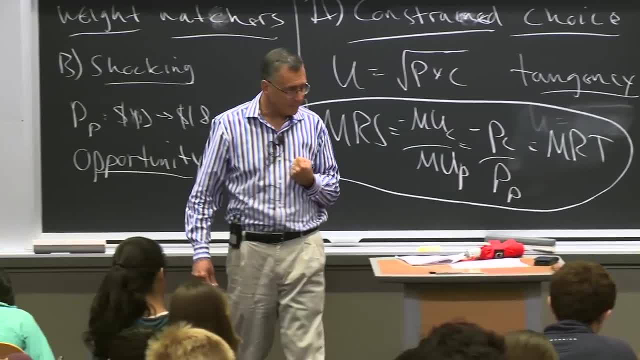 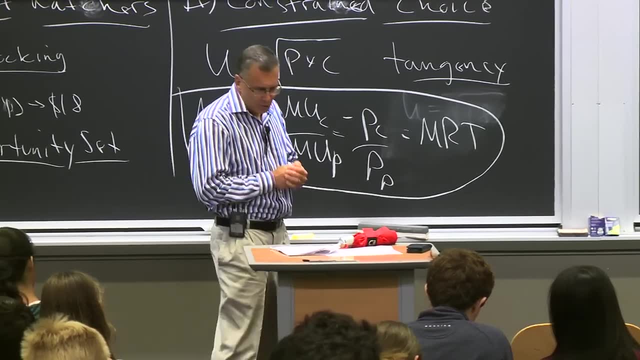 You want to put your next dollar where it's going to make you happiest, OK, And so basically think of that as your bang for your buck. OK, So, for example, suppose you were in a position where the MRS was greater than the MRT. 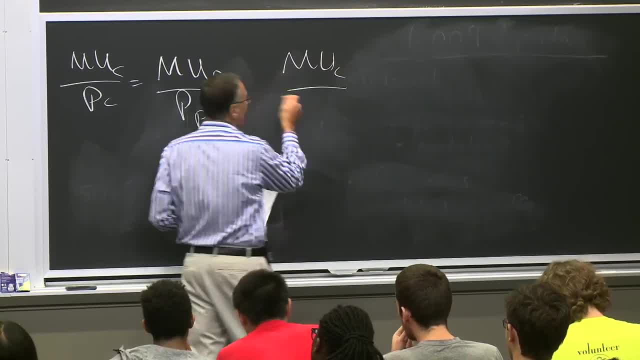 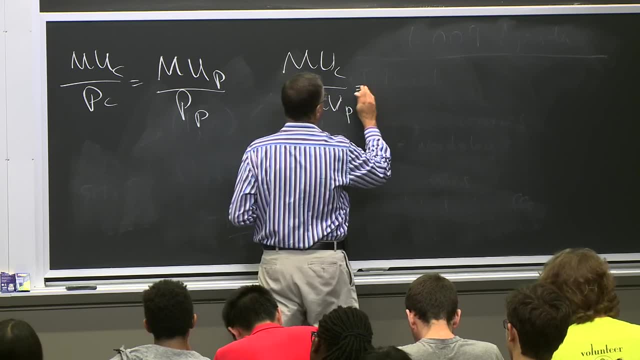 You're in a position where the marginal utility of cookies- and I'm getting rid of the negatives- There's negative on both sides. I'm just going to get rid of the negatives. OK, The marginal utility of cookies over the marginal utility of pizza was greater than the price of cookies. 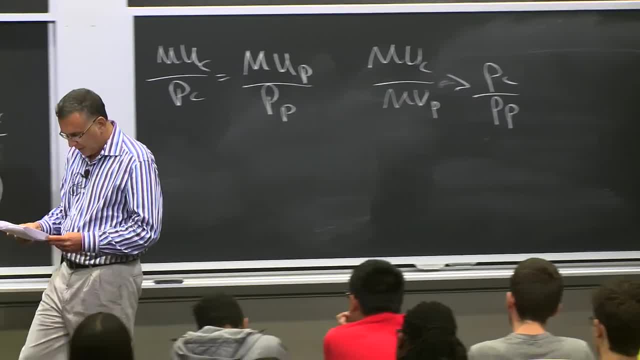 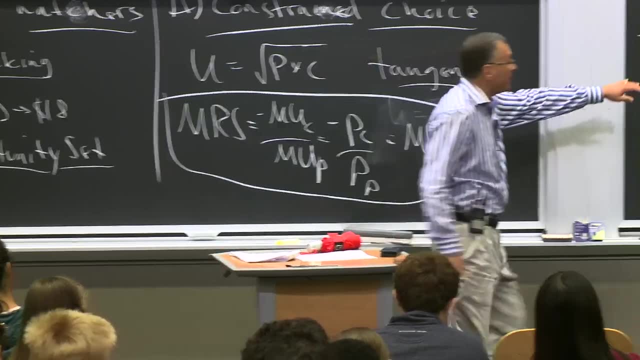 over the price of pizza- OK, That is the slope of the indifference curve- was greater than the slope of the budget constraint. This is the slope of the indifference curve. OK, The slope of the indifference curve. this is the slope of the budget constraint. 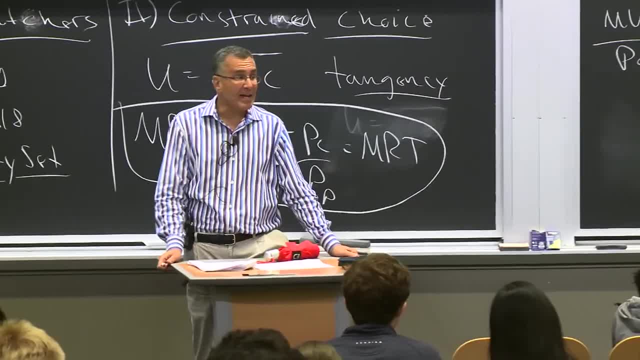 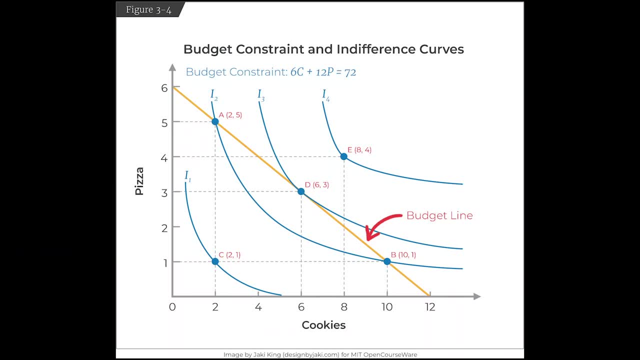 In absolute value. the slope of that difference curve is greater in absolute value than the slope of the budget constraint. OK, That would be true at points like point A, point A, where you intersect, where you basically intercept from above the budget constraint. 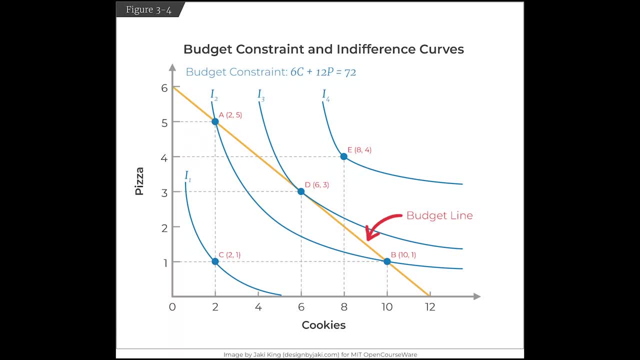 by the indifference curve. So a point like point A has a steeper slope of the indifference curve than it does the budget constraint. What that says is intuitively- and once again I want you to understand the intuition- the rate at which you are willing to give up. 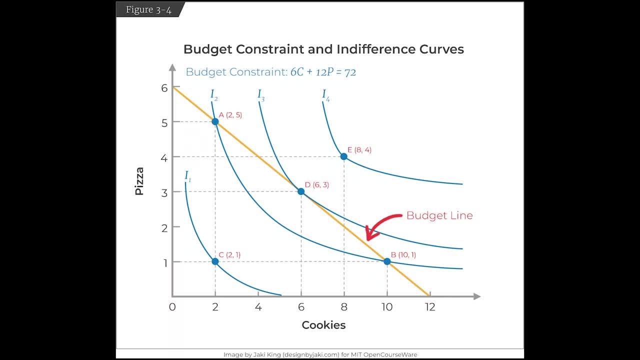 the rate at which you are willing to give up cookies for pizzas. I'm sorry, let me say it a better way: The marginal benefit to you of another cookie relative to another pizza is higher than what the market will charge you to turn pizza into cookies. 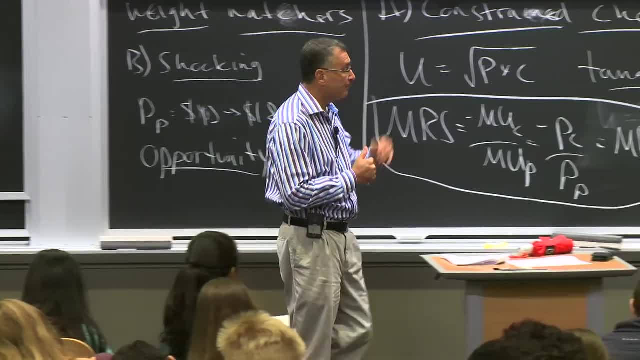 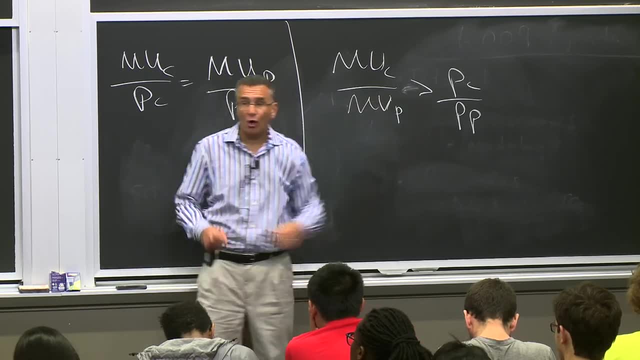 Let me say it again: The marginal benefit to you of another cookie, which is this: this is how much more you want the next cookie relative to how much more you want the next pizza- is greater than what the market is going to charge you to trade. 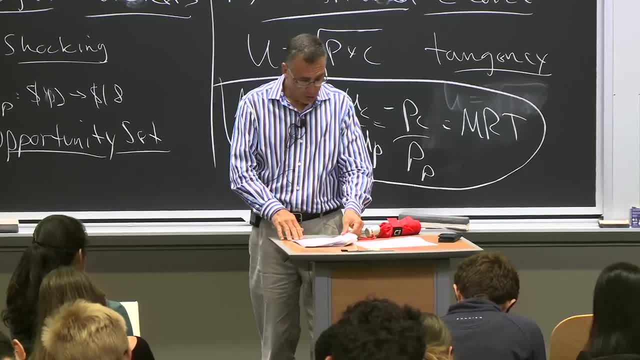 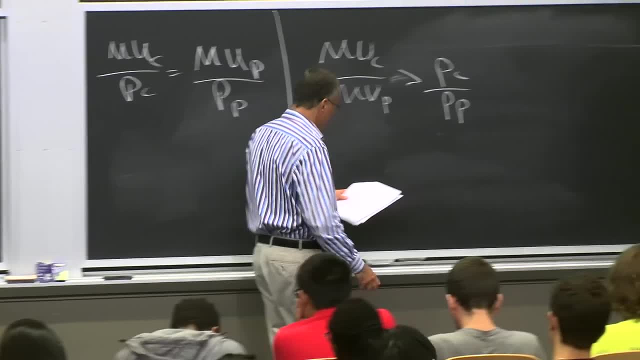 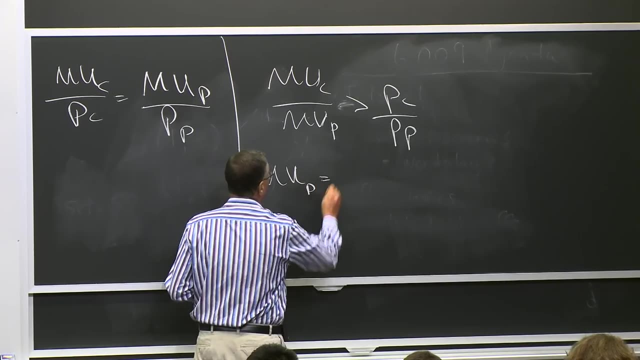 in your pizza for cookies. Therefore, you should trade in your pizza for cookies, Okay, So let's see this mathematically. At a point like A point A, okay, you have your marginal utility for pizza is the derivative of the utility function with respect to the number. 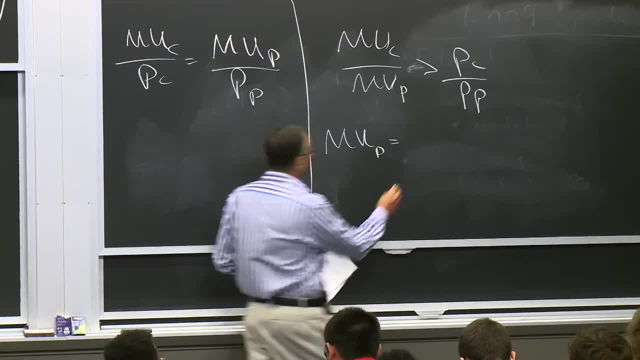 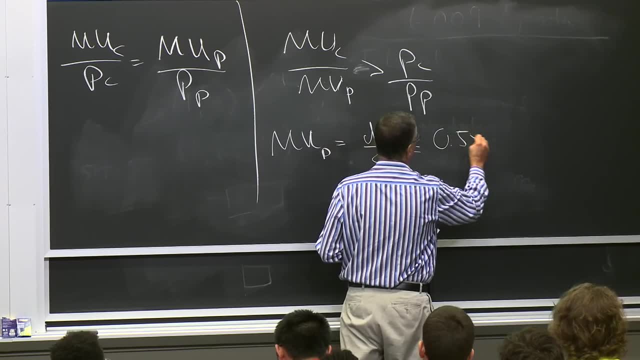 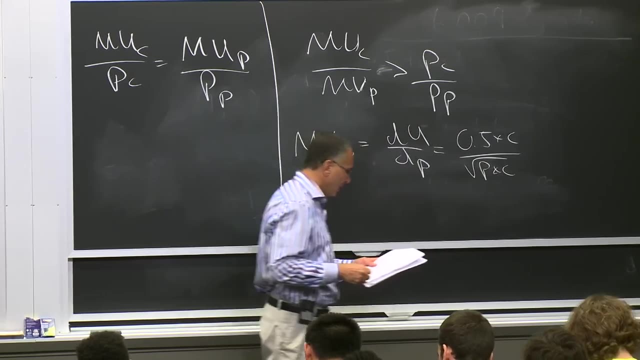 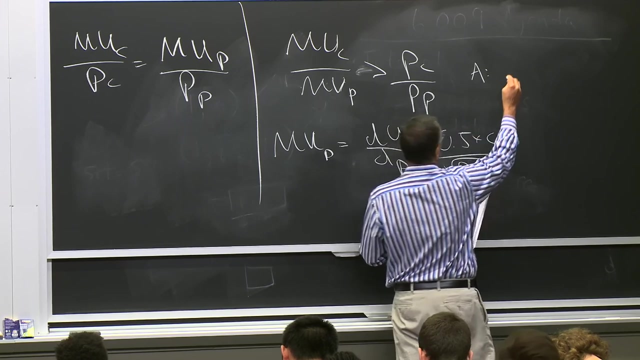 of slices of pizza, marginal utilities derivative of the utility function. So it's du dp, okay, which is equal to 0.5 times c over square root of p times c, Okay, So, and at point A? at point A, we had two cookies and five pizzas. 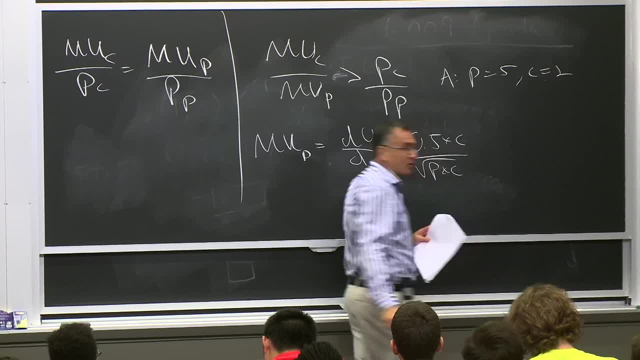 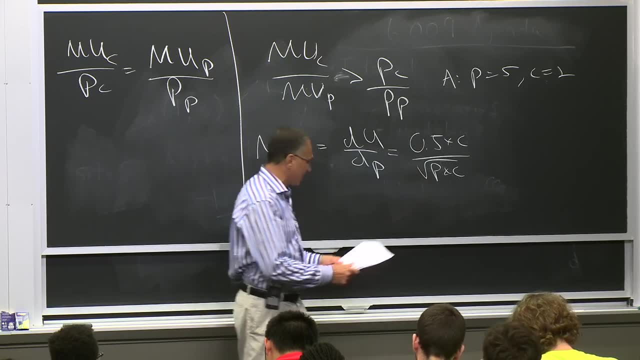 At point A, p was five, c was two. Okay, that's true at point A. So we can evaluate this marginal utility: du dp, which is equal to 0.5 times c over square root of p times c, So that's 1 over the square root of 10.. 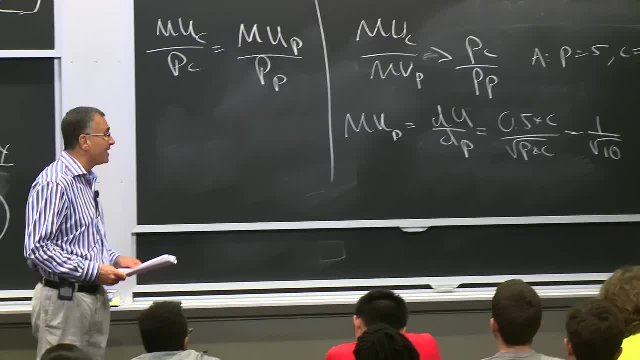 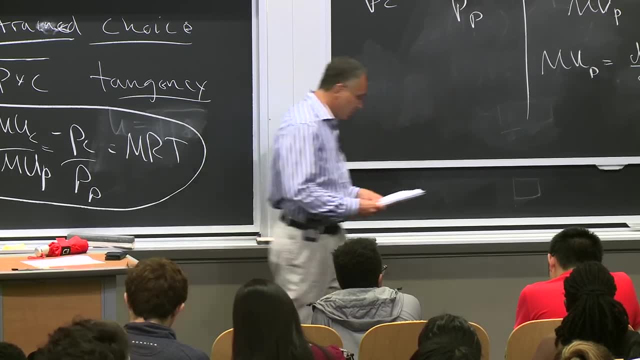 Okay, That's the marginal utility of the next slice of pizza. The next slice of pizza makes you 1 over square root of 10 happy Once again. that number is meaningless. We only care about it in ratio. So we need the ratio. 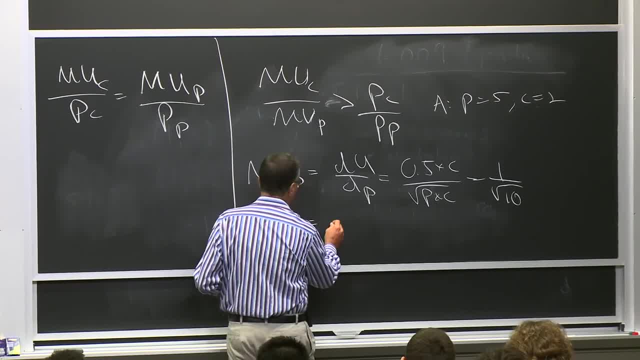 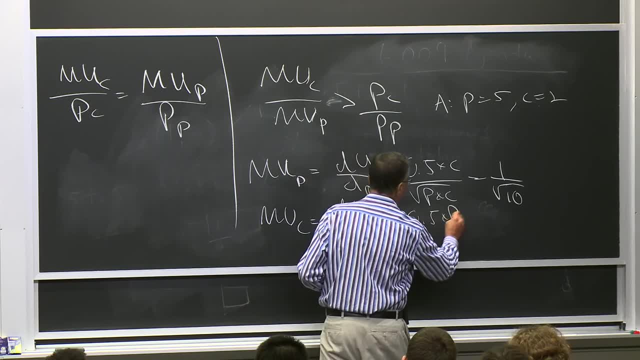 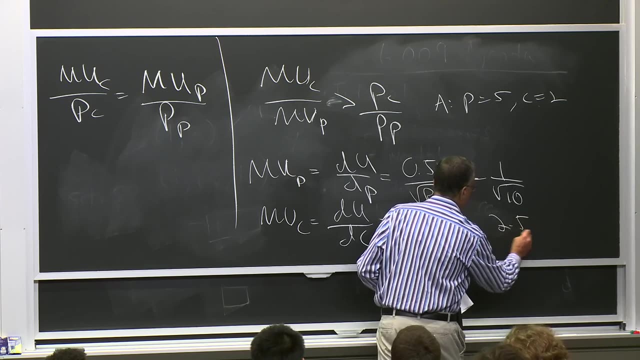 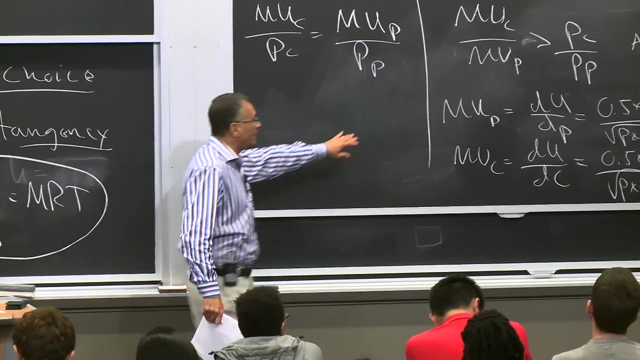 So let's do the marginal utility of cookies, That's du dc, which is 0.5 times p over square root of p times c, which is 2.5 over the square root of 10.. Okay, So the marginal utility of pizza is 1 over square root. 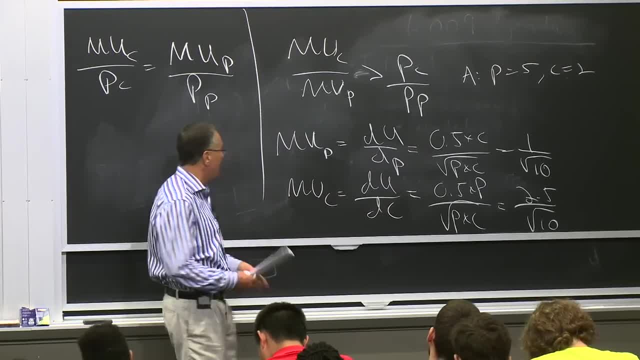 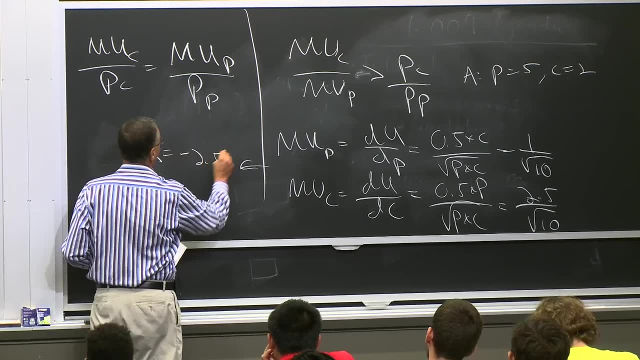 of 10,. marginal utility of cookies is 2.5 of the square root of 10, okay, 2.5 of the square root of 10.. Therefore, your marginal rate of substitution is minus 2.5.. Remember, marginal rate of substitution is MUC over MUP. 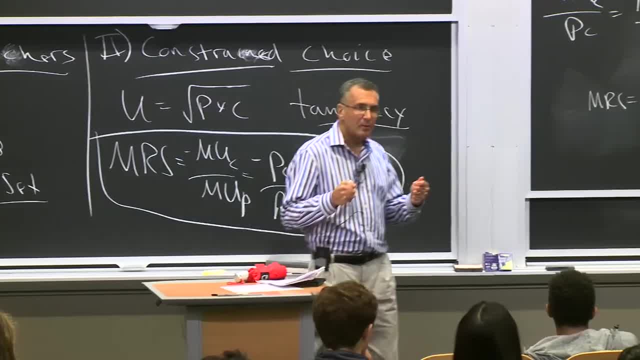 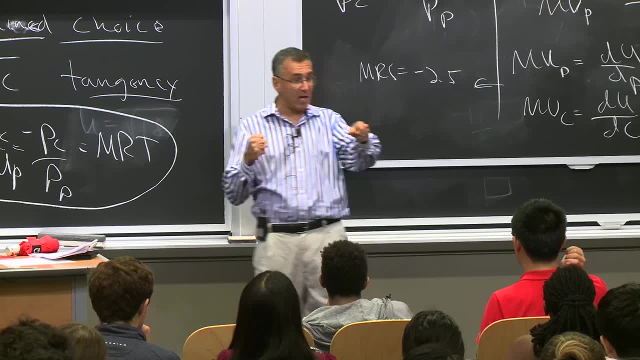 So your marginal rate of substitution is minus 2.5.. What does that mean? Can anyone tell me what that means? Your marginal rate of substitution is 2.5.. What does that mean? That is a meaningful concept. Utils are not, but that is. 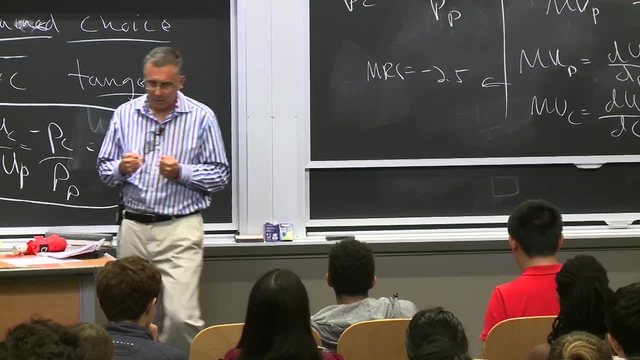 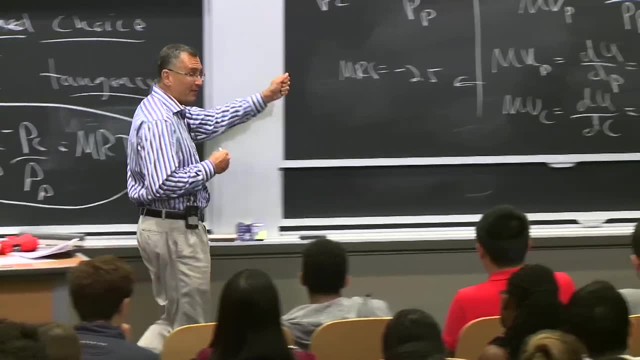 Yeah, Say it loudly so we can hear it. If you're willing to trade two pizzas for one cookie, You're willing to trade exactly. You're willing to give up 2.5 slices of pizza for one cookie. That's what that number means. 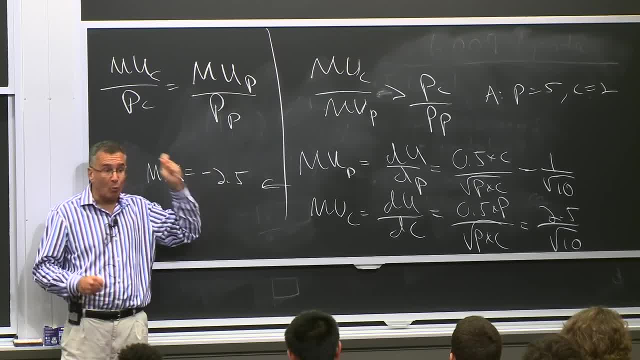 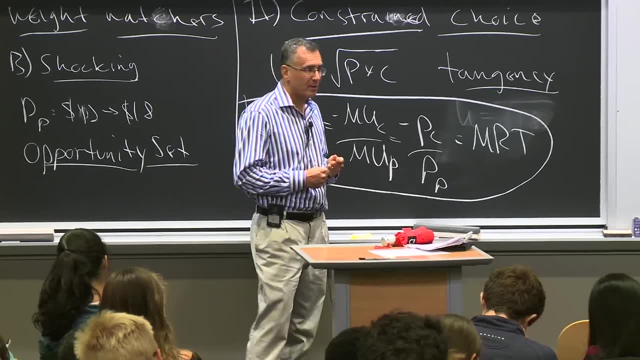 And that is a meaningful number. That's not an order, That's cardinal. We can use that. You're willing to give up 2.5 slices of pizza to get one cookie. What is the market asking you to give up? How much pizza do you have to give up to get one cookie? 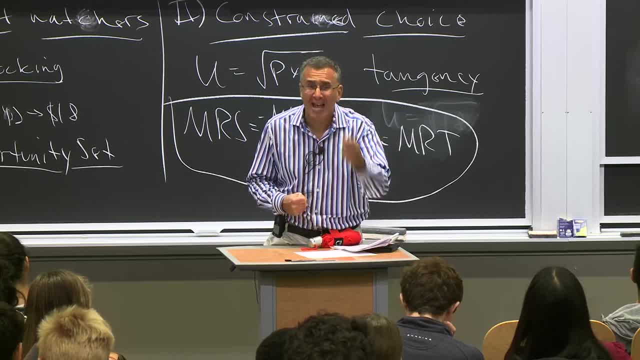 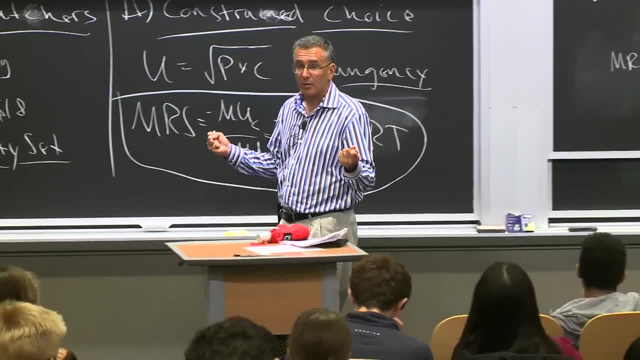 Half a slice, Half a slice. You are happy to give up 2.5 slices of pizza to get a cookie, But the market's saying, well, let's have a cookie for half a slice of pizza. So what should you do? 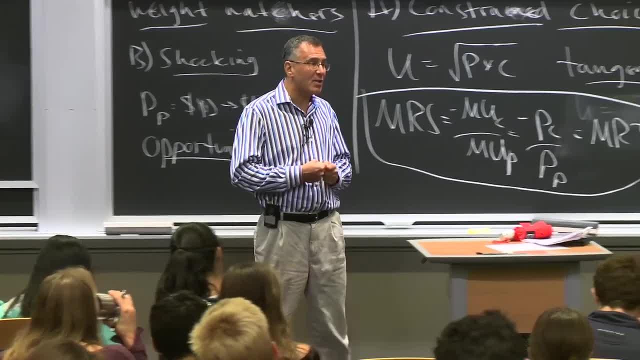 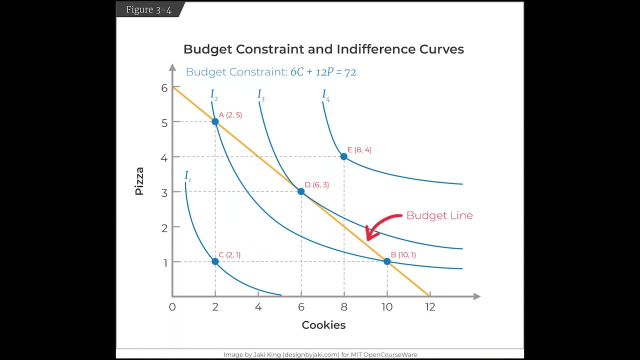 Eat less pizza, eat more cookies. That will unambiguously make you happier, And that's why you should move from point A towards point D. That's the intuition. You basically want to trade pizza for cookies until these things are equal. 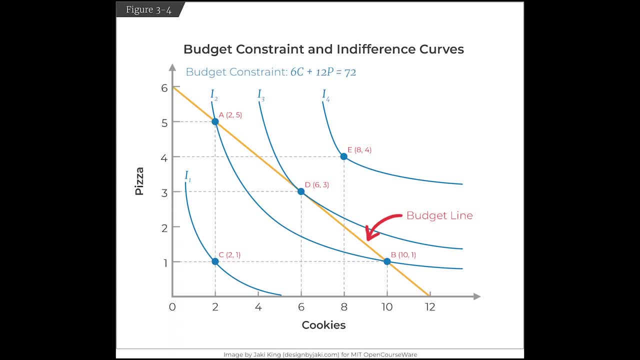 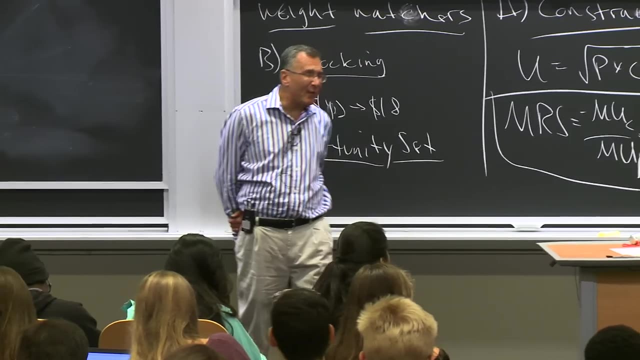 Indeed, I'd like you to go home and do the same math starting at point B. If you do the same math starting at point B, you'll find the MRS is much below a half. That is at that point you are happy to give up. 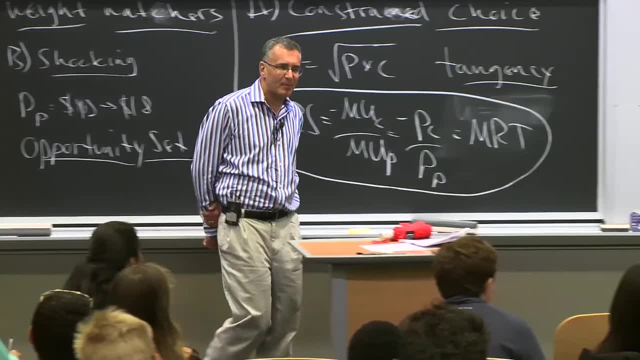 tons of cookies to get pizza Because, jeez, you've got 10 cookies and one slice of pizza. You give up tons of cookies to get pizza, But the market says you only have to give up two cookies to get pizza. 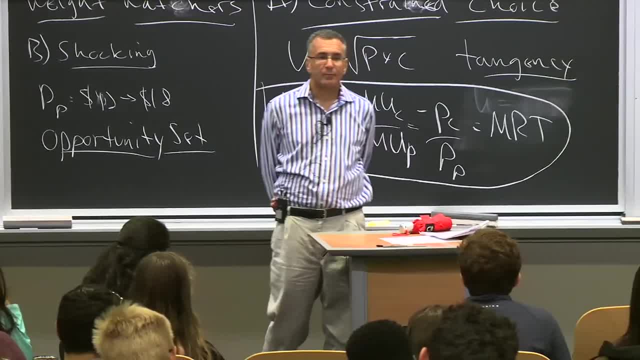 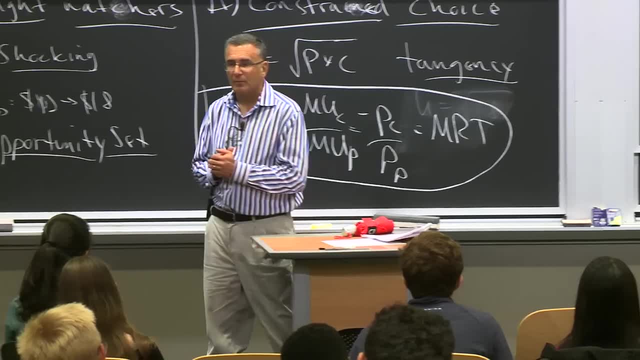 So you'll happily do it And you move back towards point D And that's the sort of in a bundle, sort of the intuition and math and graphics of how we do constrained optimization. That is hard and very important Questions about that. 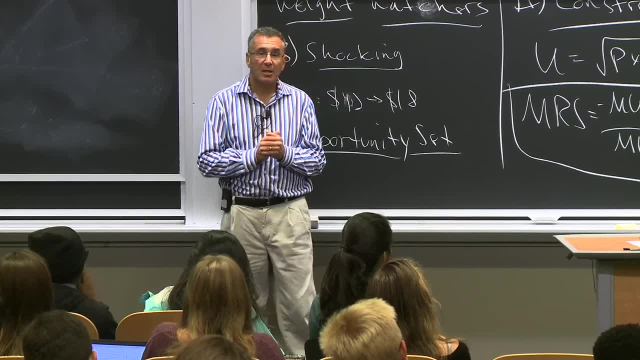 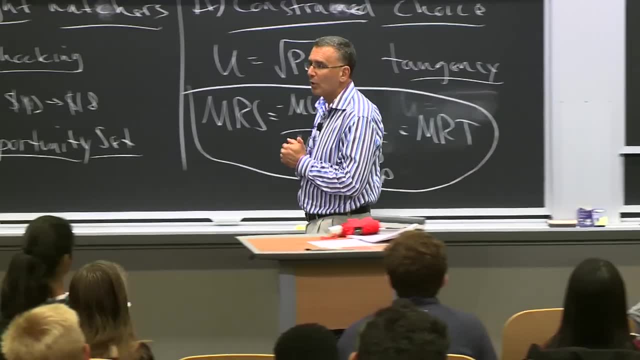 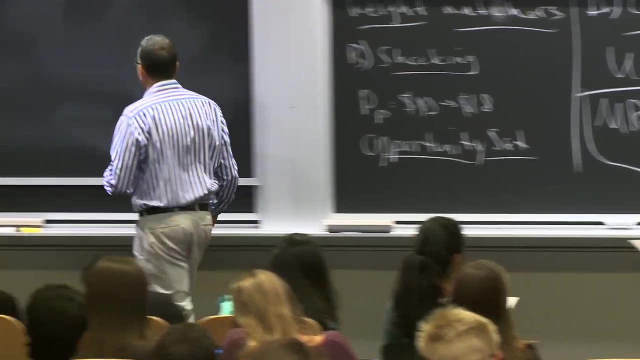 Don't hesitate to ask. That is hard and very important. If you understand this, you're sort of done with consumer theory. This is sort of the core of what consumer theory is all about. It's all about this balancing act. The whole course is fundamentally 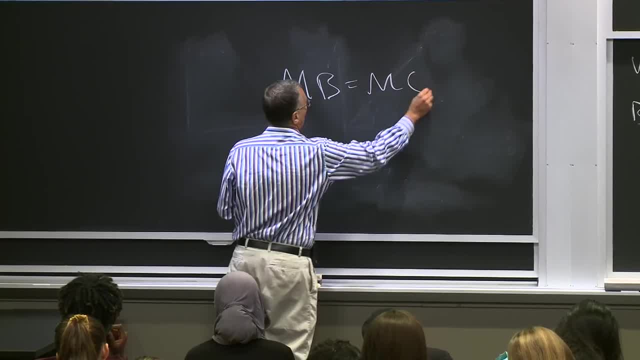 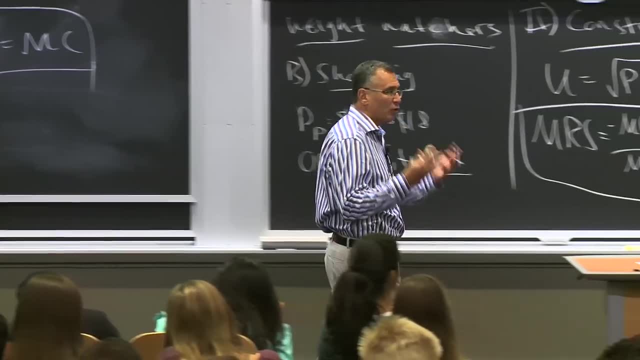 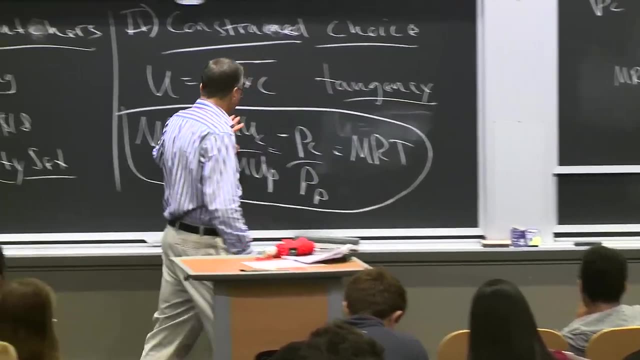 all about one equation, Which is: marginal benefits equals marginal costs. Everything we do is about weighing the marginal benefit of an activity against its marginal costs. If we take the next step, what's the benefit, What's the cost? Well, here the marginal benefit is the MRS. 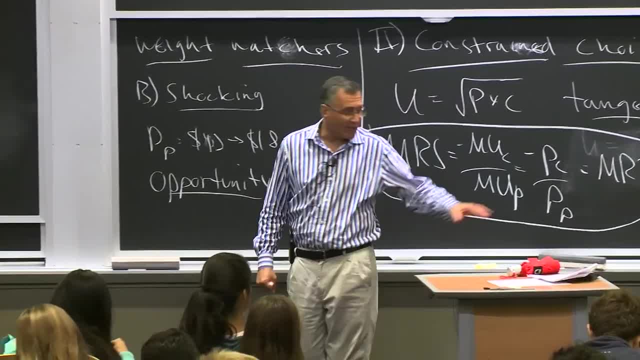 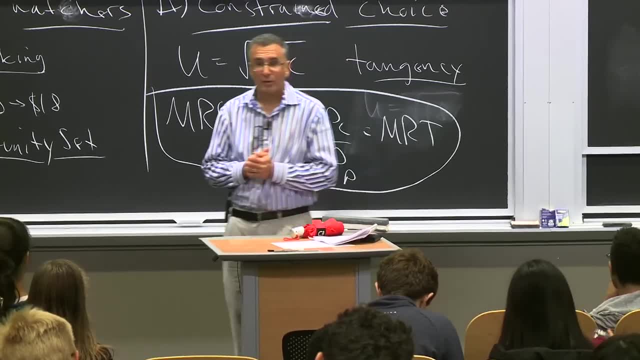 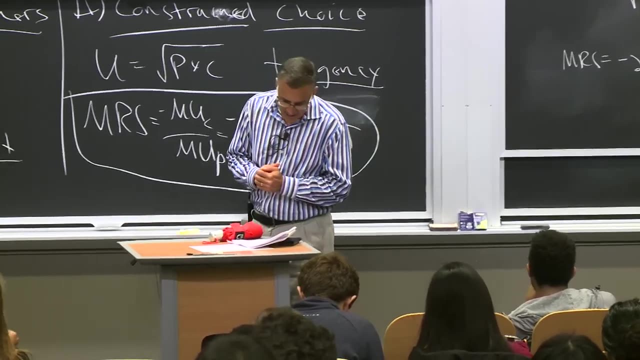 The marginal cost is the MRT. We want to set them equal, And this sort of example, I hope, explains why. So that is how we think about constrained choice. Now I want to apply it, I want to apply it. I want to apply it by looking at the example of food stamps. 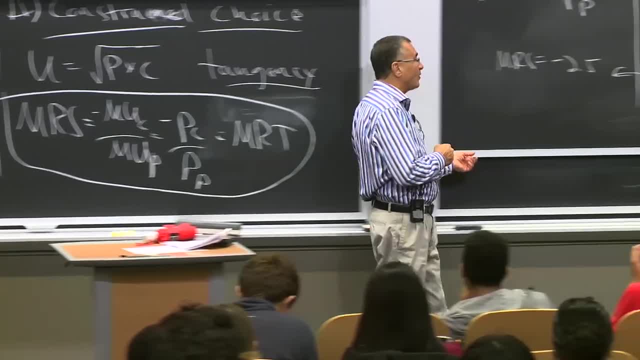 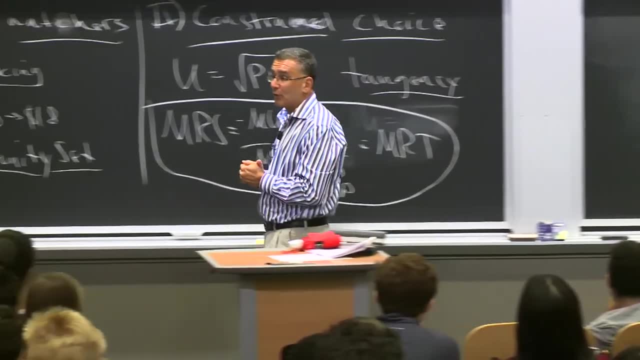 Now food stamps are not actually called food stamps anymore. When I was a kid they were called food stamps. It's basically a program the government has that provides money for individuals to buy food if they're low income. Essentially, we have in the US what's called the poverty line. 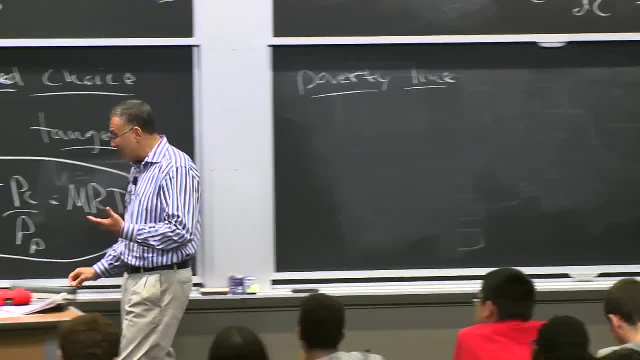 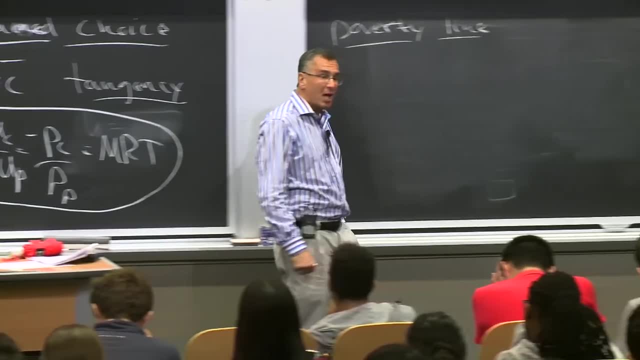 And I'll talk a lot more about this at the end of the class, But the poverty line is essentially a measure of what's a minimum level of resources you need to live. In America, the poverty line for an individual is about $14,000.. For a family of four it's about $28,000.. I feel that number obviously can depend on where you're from. If you're in Boston, you'll say that's insane. If you're from some rural part of the country, you think yeah. 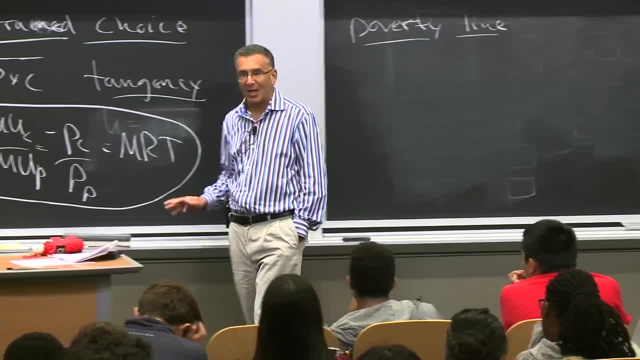 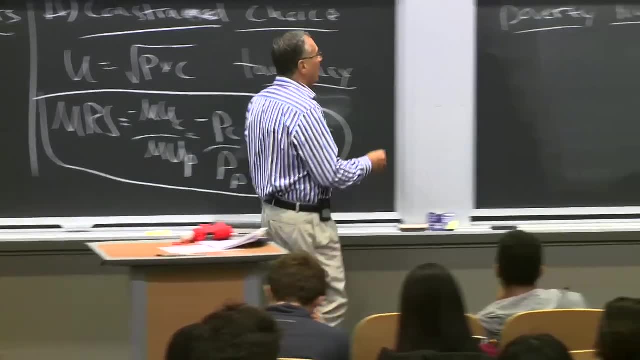 that's poor but manageable. We'll talk later about the poverty line, what's good and bad about it, But in any case, if you're below the poverty line in America, roughly speaking, you get help with buying food, And that comes through a program we now call SNAP. 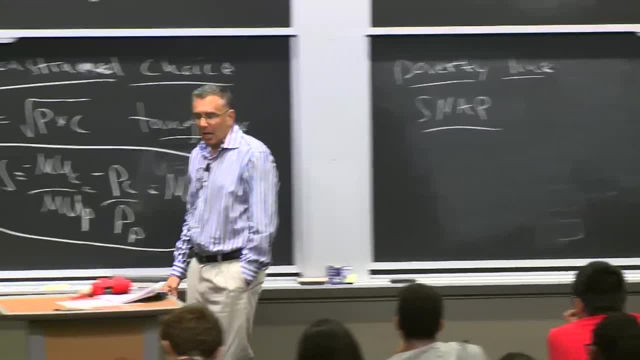 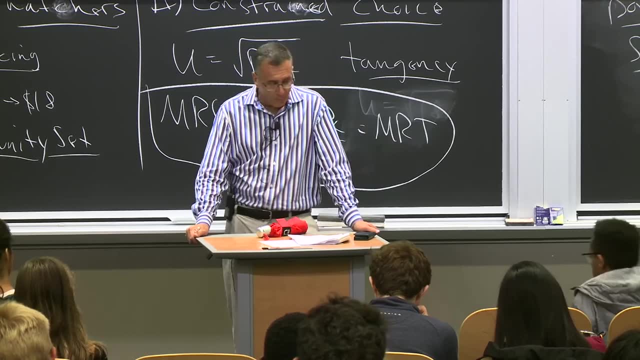 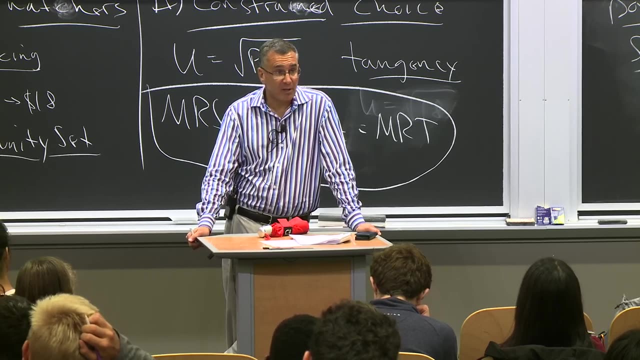 Used to be called food stamps. I got to update my notes. Supplemental nutrition? I don't know. I know the N's for nutrition. So basically what the SNAP program does is it gives you a debit card. If you qualify in income grounds, you get a debit card. 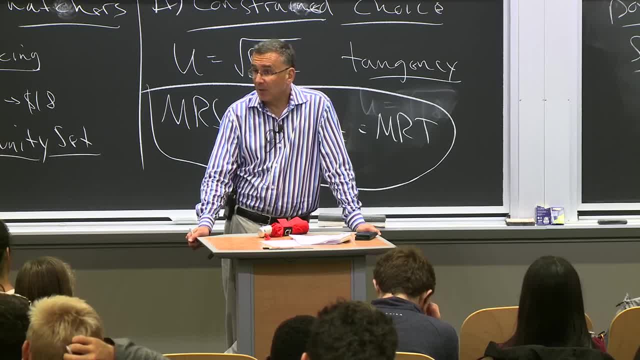 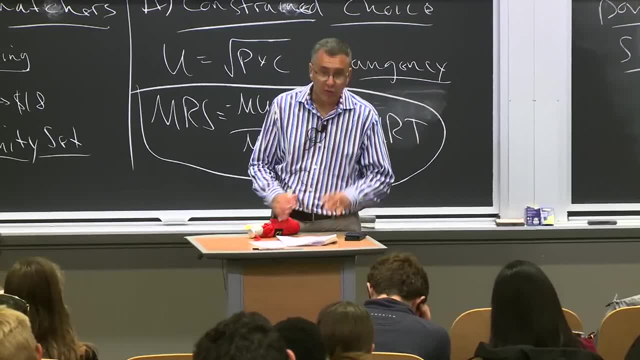 And that debit card can be used to buy food and food only. So you essentially get a debit card from the government that you can use to buy food if you're poor enough, And they give you sort of a fixed amount every month And that month can be used to purchase food. 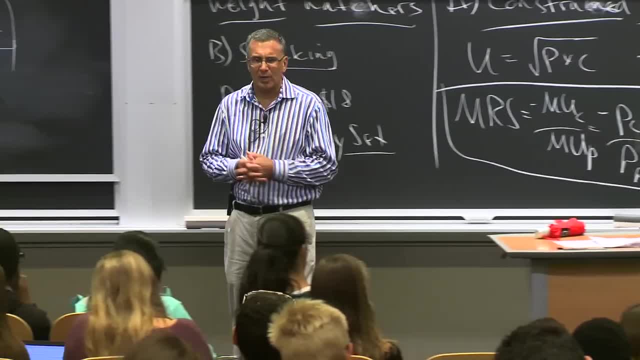 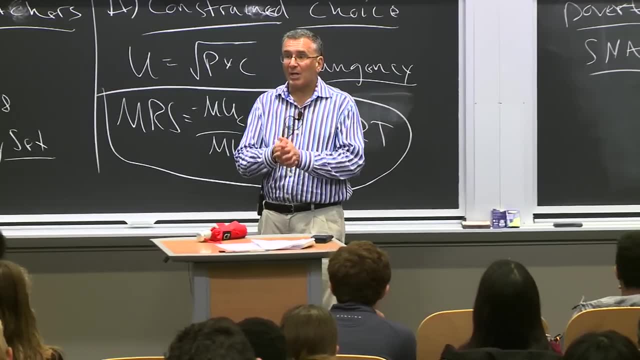 So here's the question: Why go through this rigmarole? Why not just give people cash? It's a fancy thing. If we want to give poor people money, why not just give them money? And I don't want the answer yet. 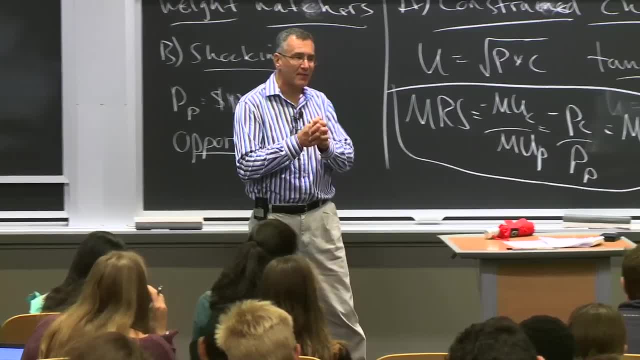 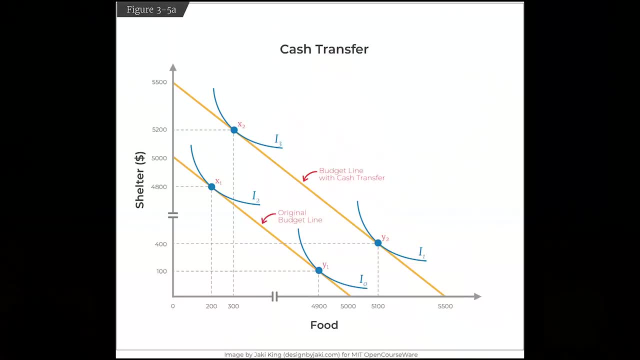 OK, What I want to do is show you graphically how we think about the trade-off, And then we'll come to the answer. So hold your thoughts. So let's actually graph how we think about food stamps. Let's go to figure 3-5-A And let's start with a cash transfer. 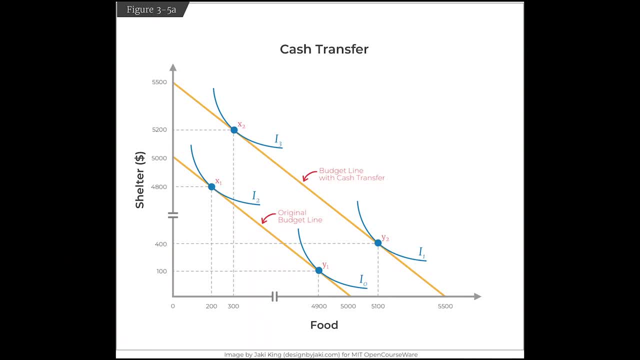 So here's the setup. Imagine people start with an income of $5,000.. That's super poor. OK, $5,000 is their whole family income for the year And let's say all they can spend it on is food or shelter. 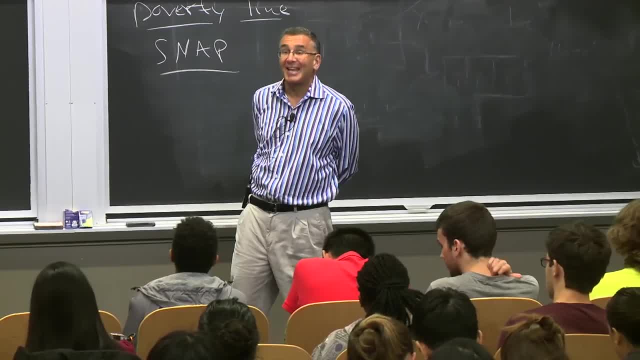 Remember, as this gentleman pointed out, in life there's more than two goods, But it makes it a lot easier to have two goods. So imagine, in this case, your two goods are food and shelter And actually, quite frankly, if you're that poor, 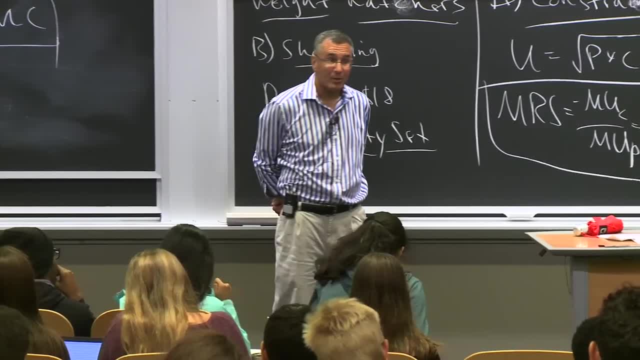 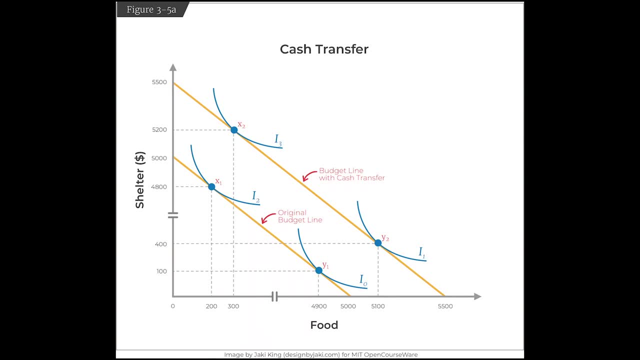 that probably isn't only two goods you can worry about at that level of income. OK, It's food and shelter. So you have $5,000 to devote to food and shelter. So you have some original income. The original budget line, which is labeled there: 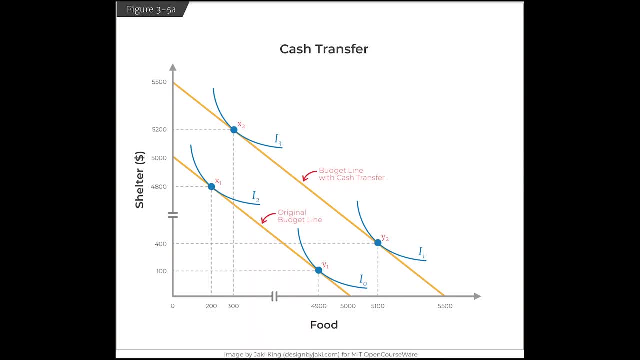 original budget line that runs from $5,000 of food to $5,000 of shelter, And then you could have some along the way. Now let's say we give someone $500 in cash. Obviously this graph is not to scale. 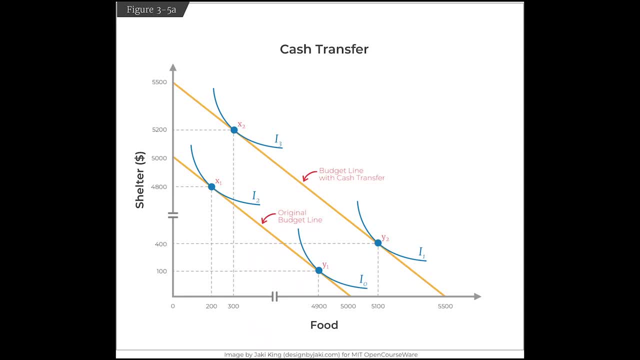 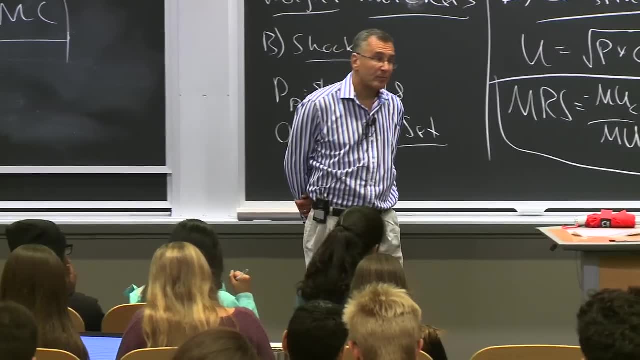 It looks like you're doubling his income. It's only $500.. This just sort of makes it easier not to scale graph. Let's say we give someone, We say to them: look, you're poor, We're going to give you $500 in cash. 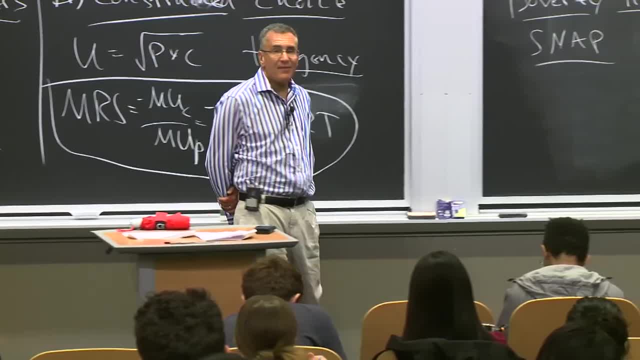 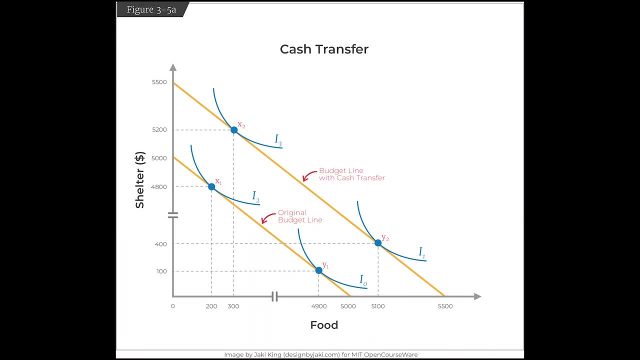 Well, now, all we've done is shift out your budget constraint from $5,000 to $5,500.. We've shifted out your budget constraint from $5,000 to $5,500.. What does that do to your choices? Well, consider two different types of people. 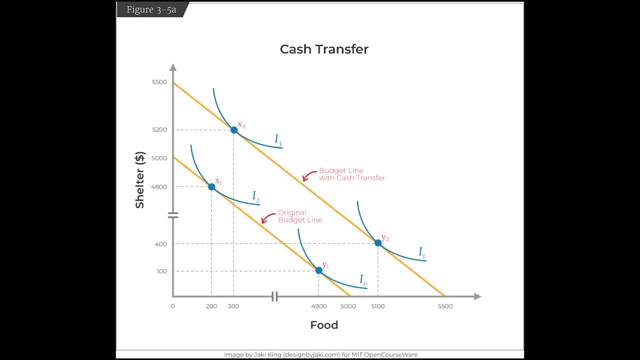 Person Y. they used to be on difference curve I0. They used to spend almost all their income on food and not a lot on shelter. They're probably homeless, So they spent all their money on food and were basically homeless. Now what do they do? 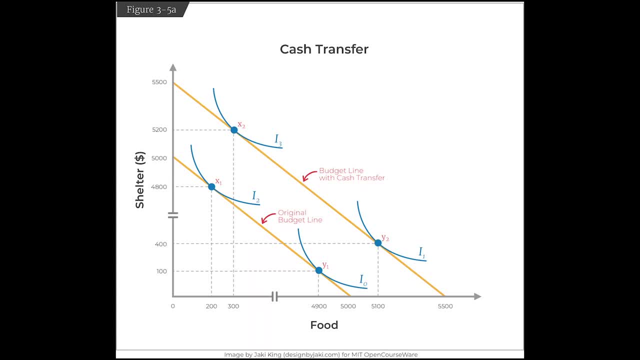 Well, they spend a little more on food and a lot more on shelter. Maybe now they get $400, still doesn't buy you much shelter. They spend a little more. Maybe a night a week they can get shelter. So basically that's what they do. 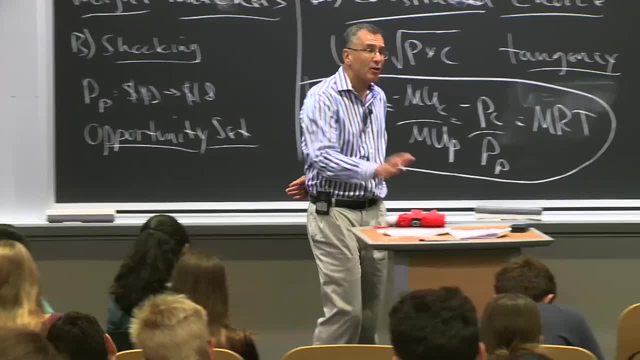 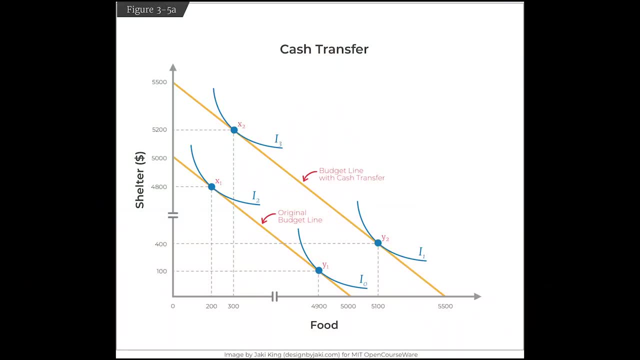 That's their constrained optimization. We're not saying it's right or wrong. This is not normative economics, It's positive. The positive thing is, given their utility function, they move from point Y1 to Y2.. Now imagine someone like individual X. They're different. 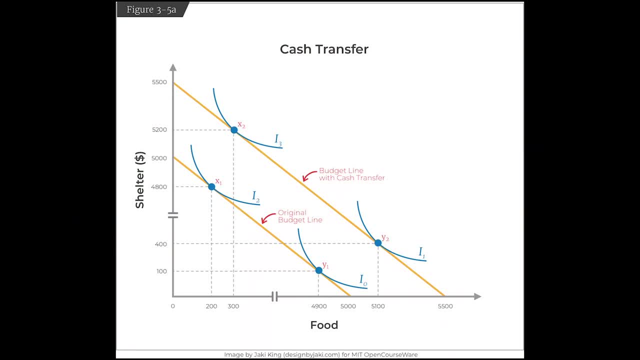 They're tastey. Their tastes are such that they don't need to eat, They just want to have shelter. So they're up at point X1 initially, And you give them that $500, and they spend just a little bit more of it on food and even more of it on shelter. 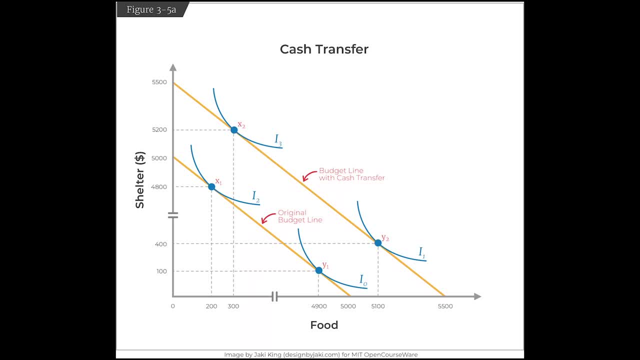 They just love their shelter And they're just super Weight Watchers. They don't eat, So basically they move from X1 to X2.. Once again, not normative right or wrong, It's just: these are feasible choices people could make given the opportunity set with which. 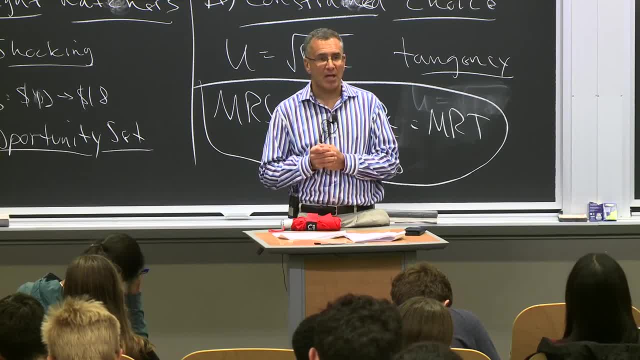 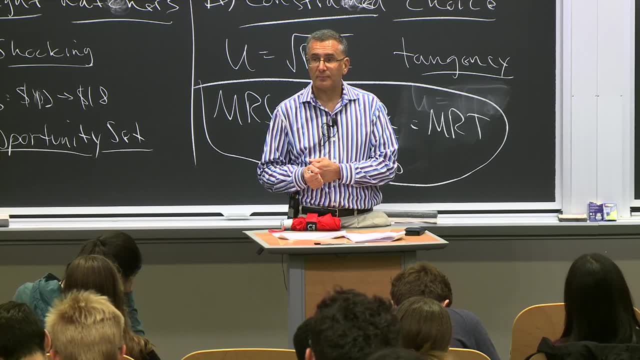 they're faced, And that's what I was looking at, And that's why I was looking at the $500 in cash Question about what I did here on this graph alone. Yeah, Even if you gave them money specifically for food, couldn't they then just reallocate their other money? 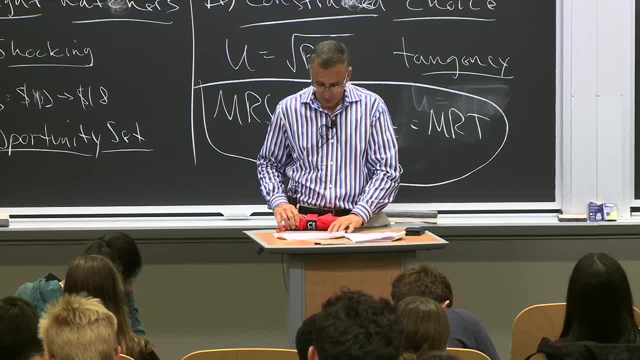 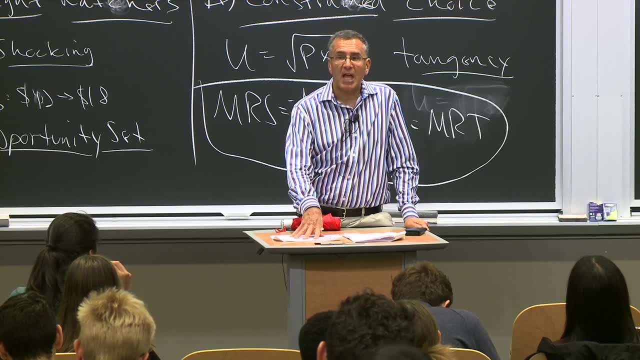 OK, that's a good point. We'll come back to that. That's time out. if you're not a sports fan, OK, so we will come back to that And in fact, OK, but do people understand what the cash transfer is, how it works? 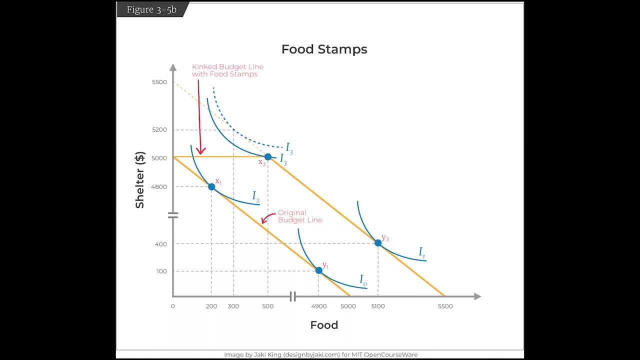 OK, now let's go to SNAP And let's say with SNAP, instead of giving them $500, we give them a debit card. Instead of handing them a $500 check, we give them a debit card with $500 on it that can only be used on food. 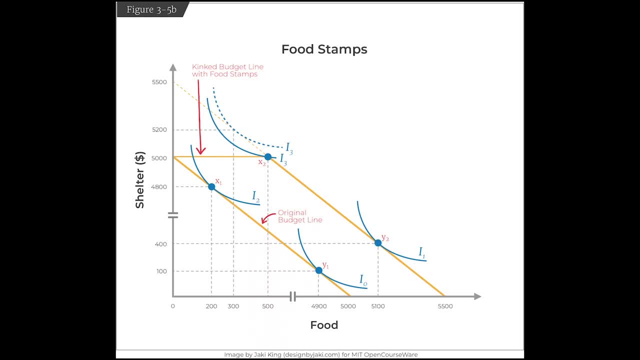 How does this affect their budget constraint? Now we see where budget constraints start to get interesting and fun and the kind of challenges you're going to face in this course in drawing budget constraints. The original budget constraint continues to be the original budget line, running from $5,000 to $5,000. 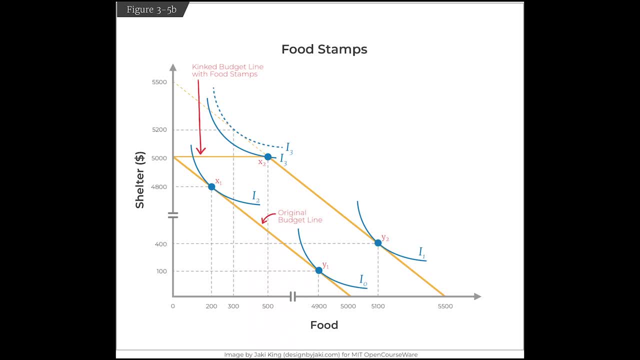 The new budget constraint is this kinked line that runs from $5,000 on the y-axis to the point X2.. OK, at $5,000 on the y-axis. So it starts at $5,000 on the y-axis, $0 on the x-axis. 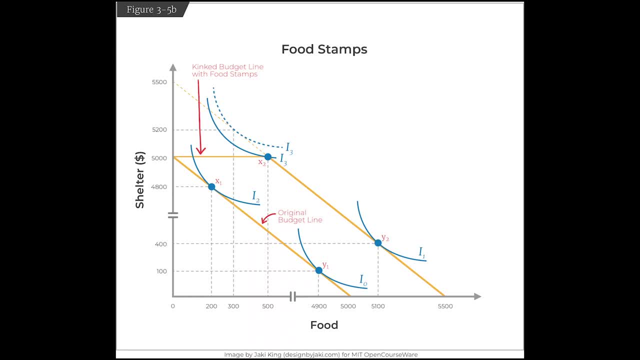 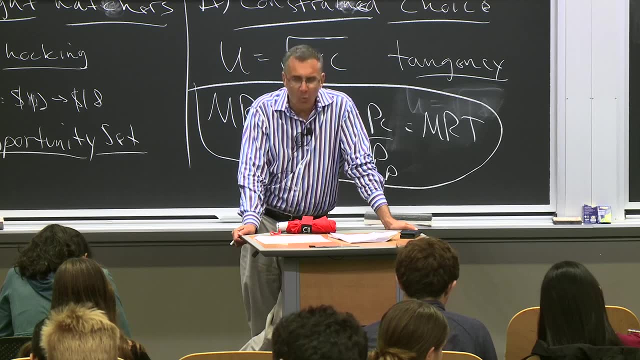 There's a flat line that goes to $5,000 on the y-axis, $500 on the x-axis, And then it slopes down parallel to the original budget constraint to $5,500.. Can someone explain to me why that's the new budget? 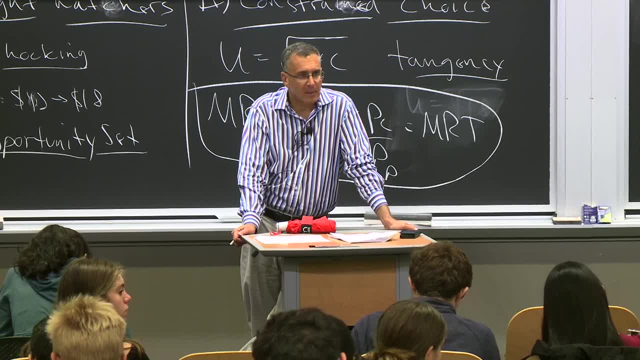 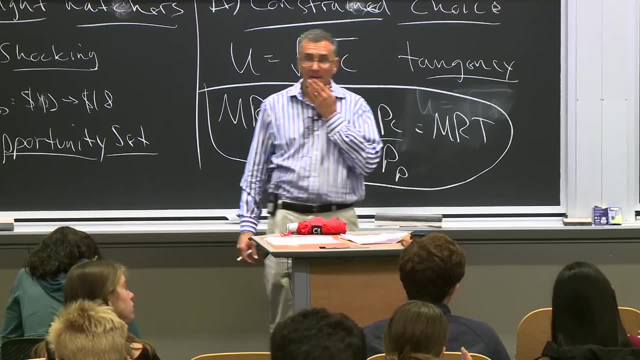 constraint. Yeah, You can't spend negative amounts of up-rated. You can't spend negative amounts if you're not Exactly. We are forcing you to spend At least $500.. Compared to cash, we can do whatever the hell you want. 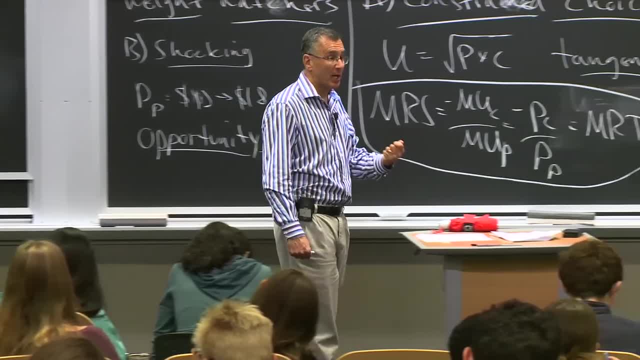 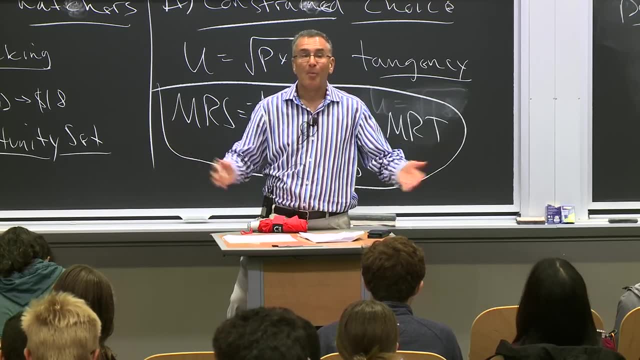 We are forcing you to spend $500 of your money on food. Coming to the question back there, it doesn't have to be a specifically labeled $500. It could be any $500. But we're forcing you to spend at least $500 on food. 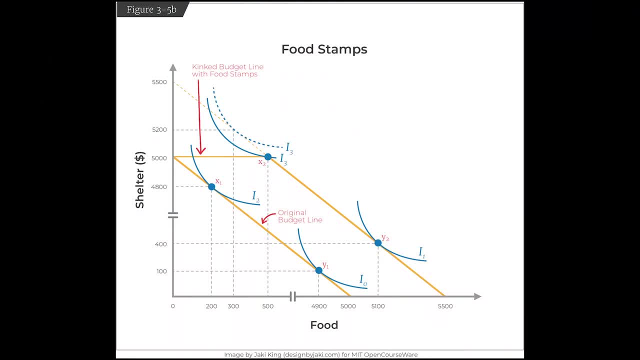 Well, what does that do to your choices? Well, for person Y, it makes no difference whether they get cash or whether they get food stamps. Now, Even light blue shirt, turquoise shirt- asked that question. Why does it make no difference? 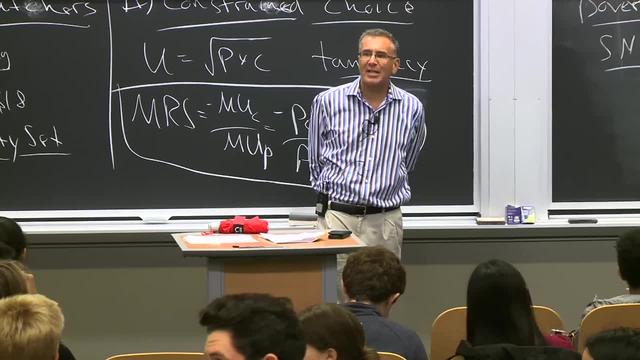 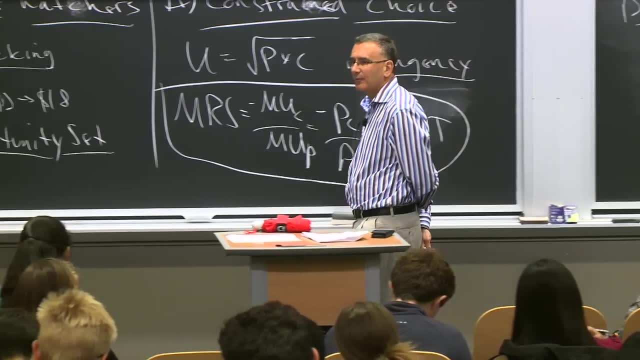 Yeah, Why does it? whatever greenish, I don't know you. Why does it make no difference for person Y if they give him food stamps or cash? He's already spending a lot of his money on food, So any money he gets he can just reallocate differently. 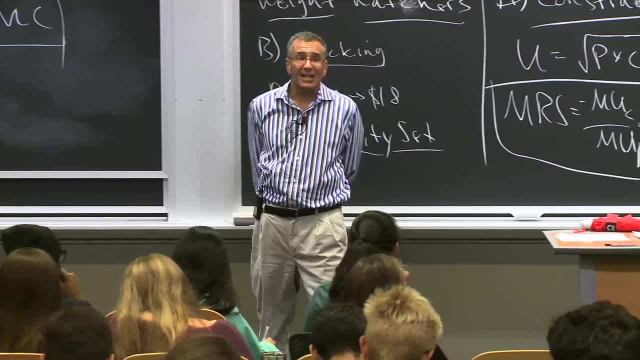 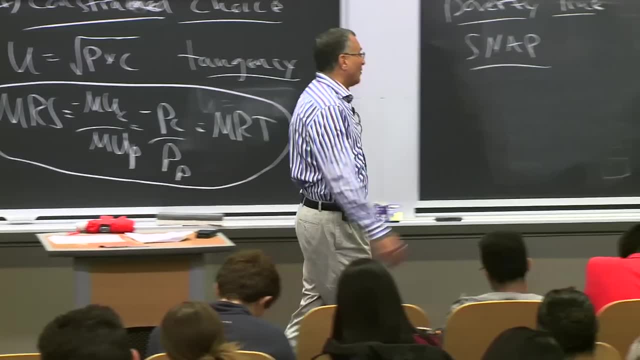 So he can spend some of the money he would have used on food on himself Exactly. He can just reallocate his money. That's exactly right. So for person Y there's no difference. Look, they're already spending what? $4,900 on food. 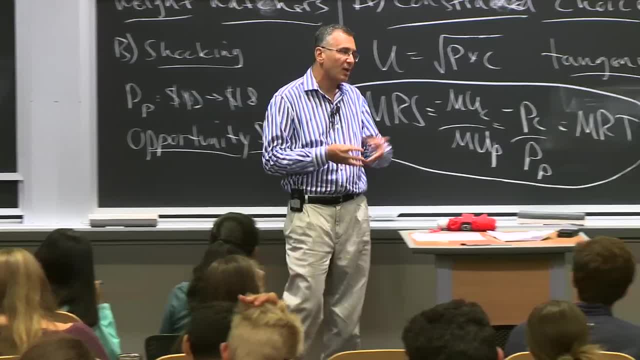 You give them a thing labeled $500.. $500 for food. it's not going to affect their life. They'll just take $500, they'll just spend. they'll just treat it as $500 more in cash. They're indifferent. 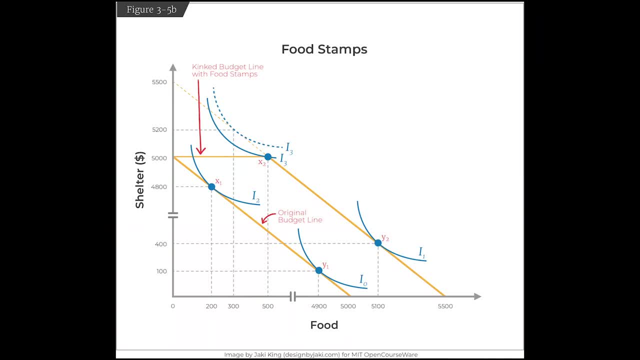 So nothing affects them. But what about person X? Well, person X, remember the dashed portion of this budget constraint is from the old cash example, And the dotted indifference curve is what they would have chosen with cash. Remember, person X with cash would 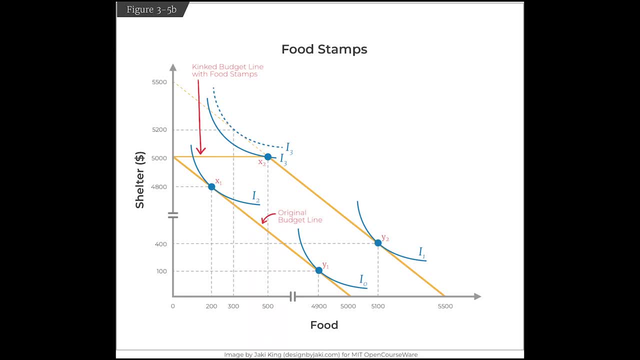 have chosen to still spend less than $500 on food, even when you gave them $500. They still only spent $300 on food. So we are forcing them to not be on their preferred budget constraint. Rather, we're forcing them down to point. 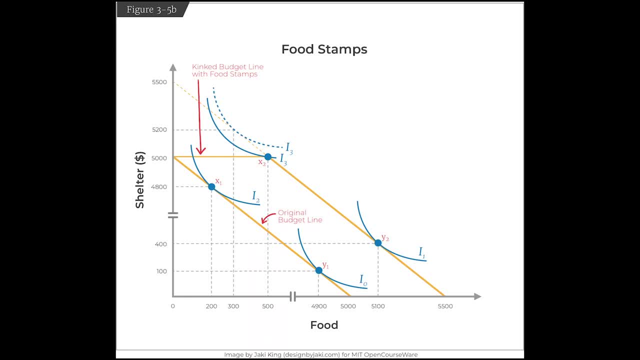 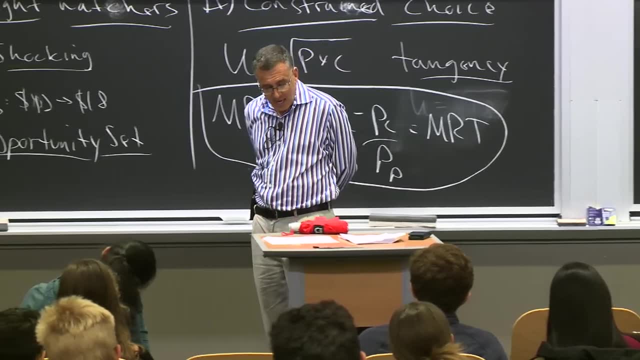 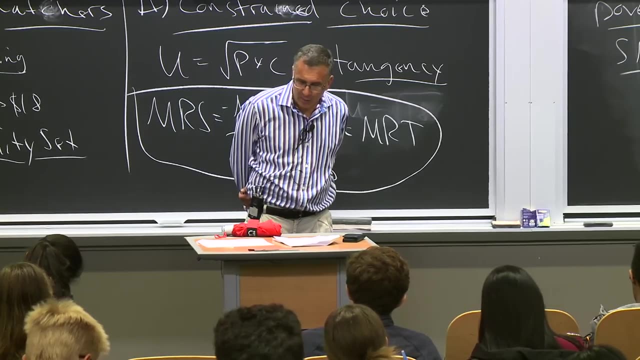 X2, which is they'll spend the minimum they can on food, but the minimum is $500.. We are forcing them down to point X2.. Now, why do I say forcing them? Why do I know for sure they are being forced, that they're? 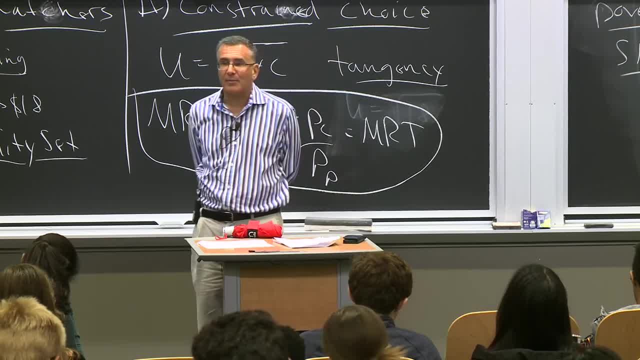 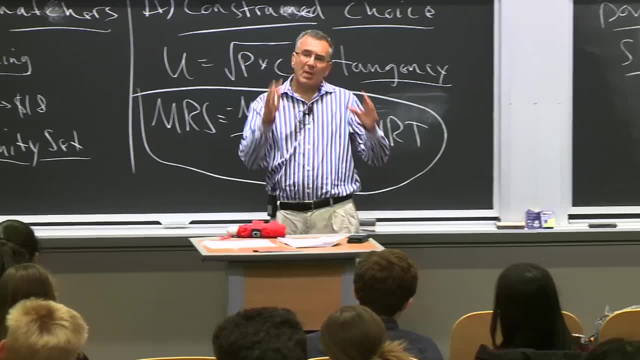 less happy at X2 than they would have been when they gave them the cash. How do I know for sure? Yeah, They're at a lower indifference, Exactly. Think of it this way: One of the important things is people always get to the point that makes them happiest. 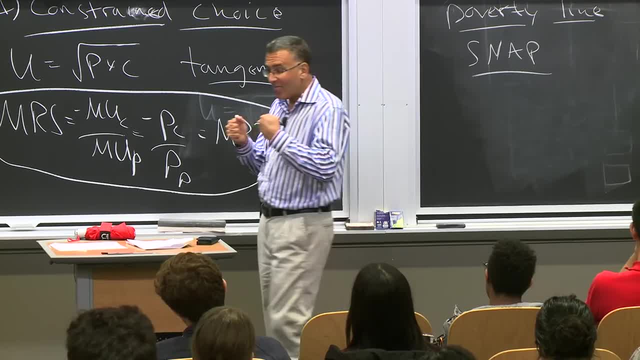 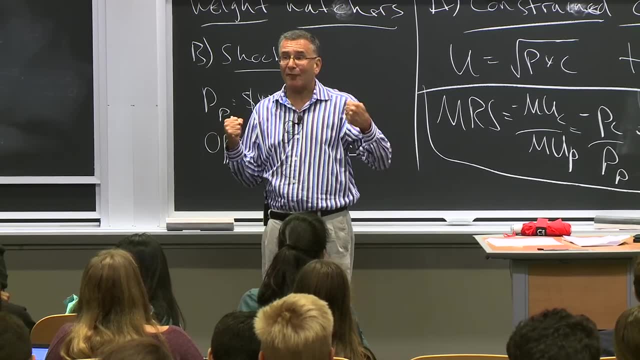 We call it the robustness of economic equilibrium. People get to the point that makes them happiest. They always before had the choice of spending $500 on food and they chose not to. Therefore, if you force them to spend $500 on food, 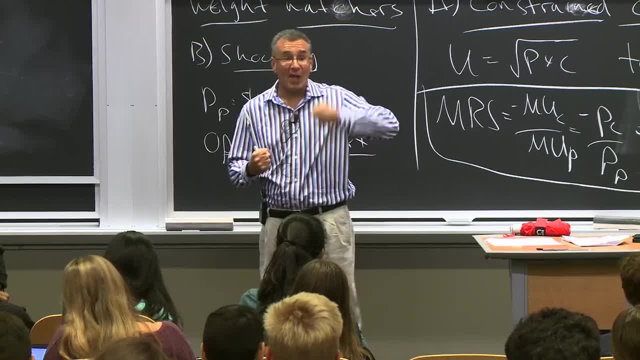 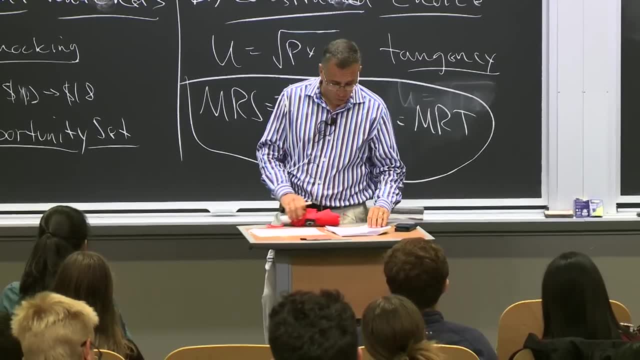 they must be less happy. Think of it that way: They always could have spent $500 on food. They didn't. Therefore, by forcing them, you're making them less happy. So they are worse off. They are forced to spend. 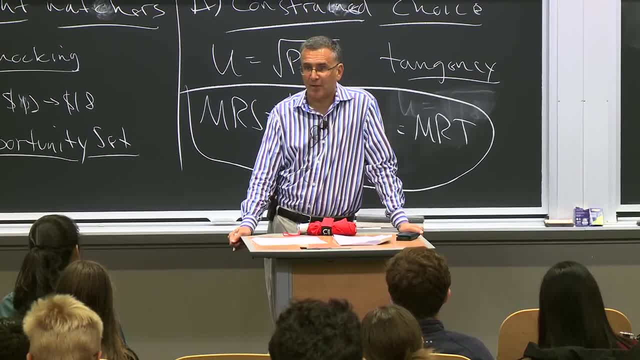 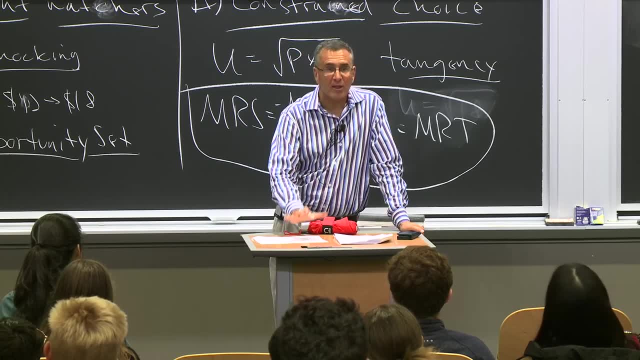 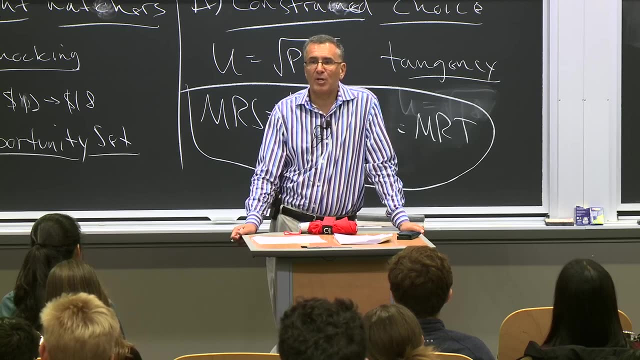 They'd rather spend some of that money to find a nicer place to live, but we're not letting them. We're making them buy food. I just want you to understand the graphics here and the conclusions I drew. Now why? Why are we doing this? 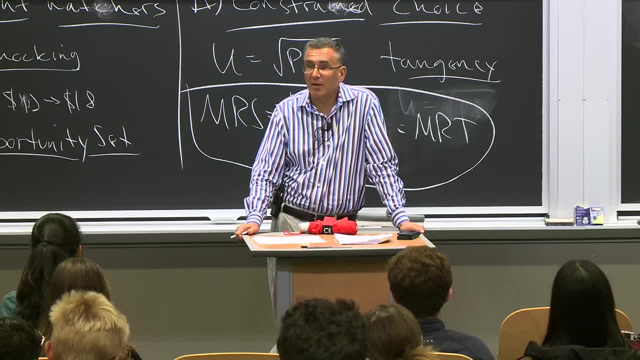 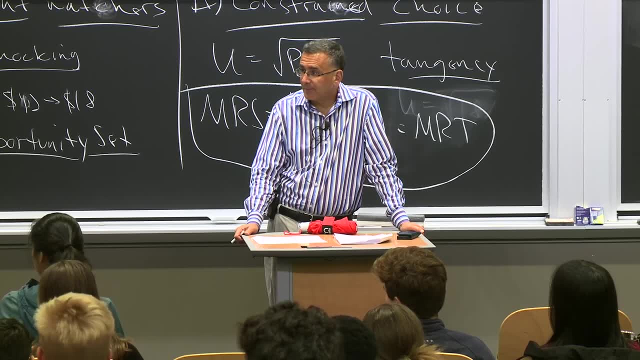 Why would you? They're better off with cash. Why would we force them to have food? Yeah, I'm saying because what makes people on the highest indifference curve is just what makes them happiest, but not necessarily what makes them live the longest or have the best health. 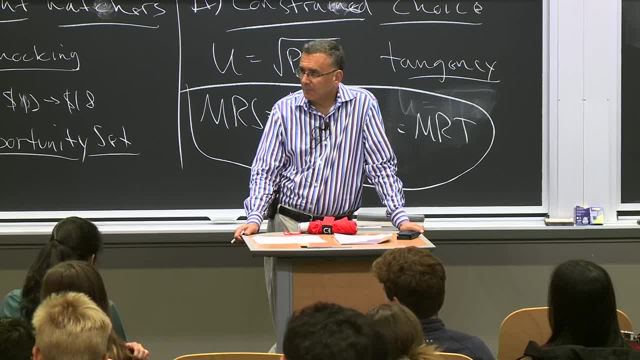 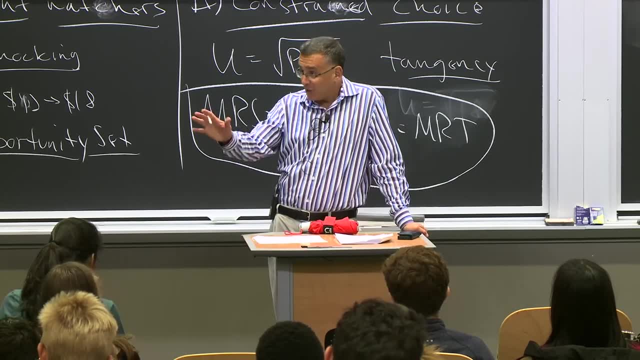 So perhaps if you never spend money on food and you die, that would be really bad, OK, But basically what you're saying is: you know better than the guy. Let me say I'm not accusing you, I'm just saying: look. 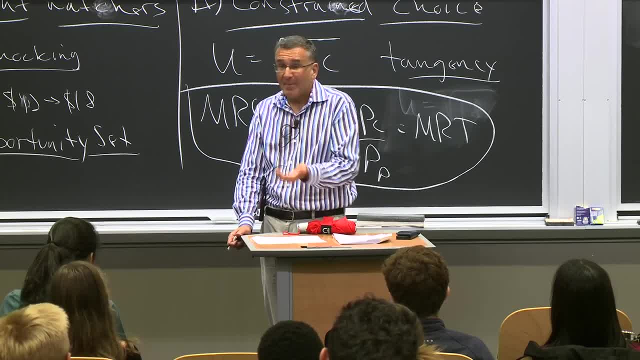 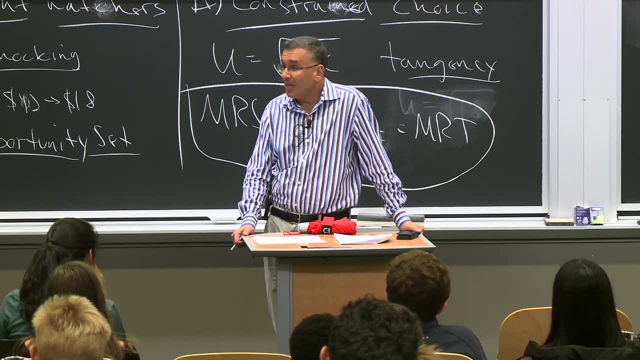 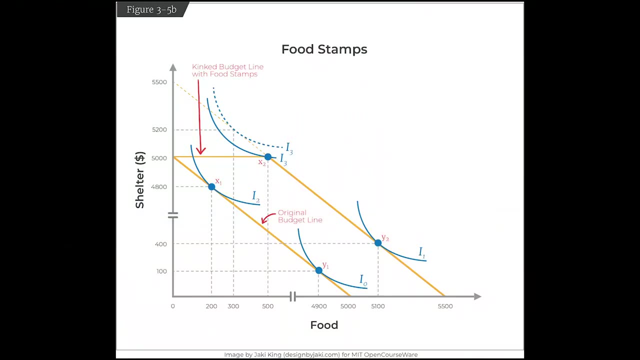 If people knew best, maybe they'd like to just have a nice house and die. If people knew best, then there'd be no reason to do this. The reason to do this is because we think they don't know best. So, for example, let's change the label on the y-axis. 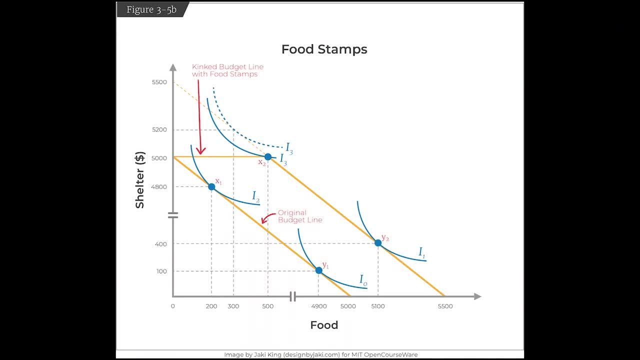 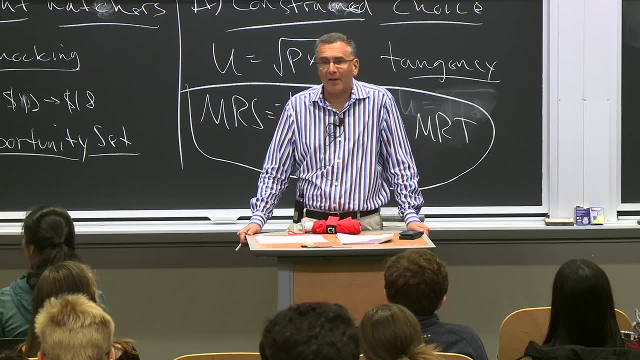 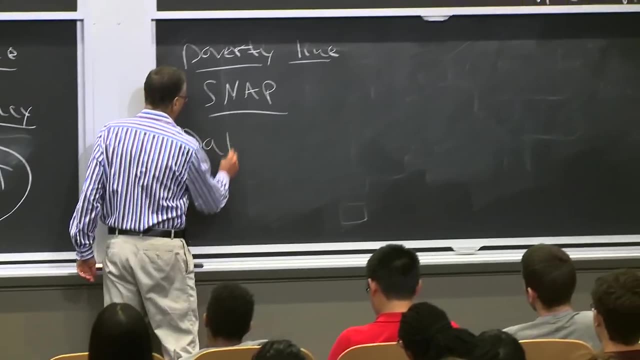 Just a small change. Let's cross out shelter and write cocaine, OK. Well, in that case maybe we don't feel so bad about forcing the guy to buy food instead of cocaine. OK, In other words, this is a program which might make sense if we are paternalistic. 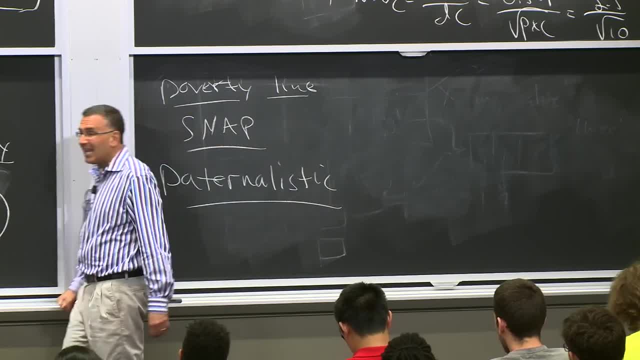 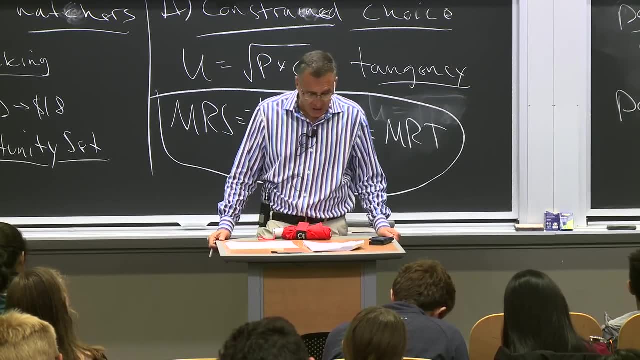 Now we're getting into norm of economics, Paternalistic. If we think that people won't necessarily make the right decisions for themselves, then it may be worth actually making them worse off, Because they're not worse off, Their perceived benefits are worse. 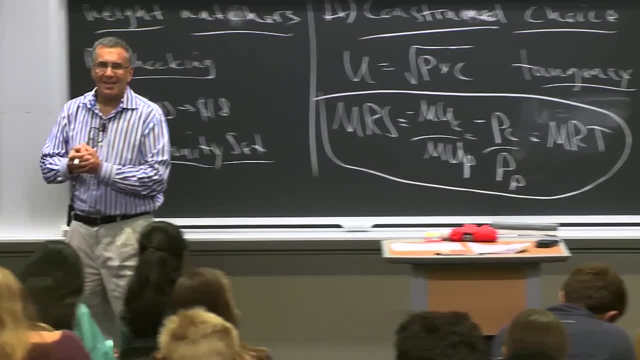 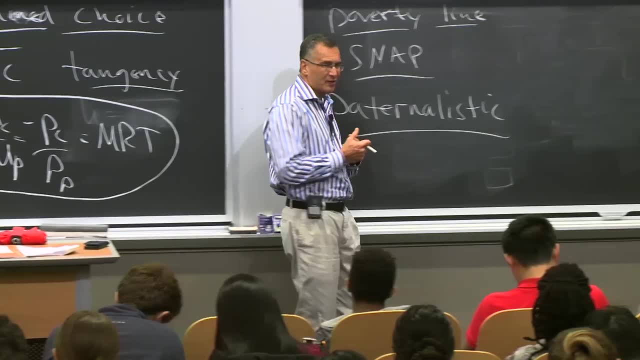 but they don't know what they're doing. OK, Now You can see why. I hope you can sort of immediately see why this concept makes economists a little nervous, Because why do we know what they want better than they do? OK, 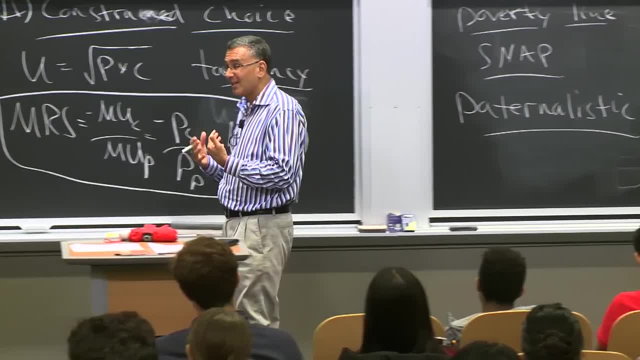 So it makes people a little bit nervous, economists a little bit nervous and a lot of people a little bit nervous to say, gee, maybe they're just happier doing cocaine. And how do we know that that's the wrong way for them? 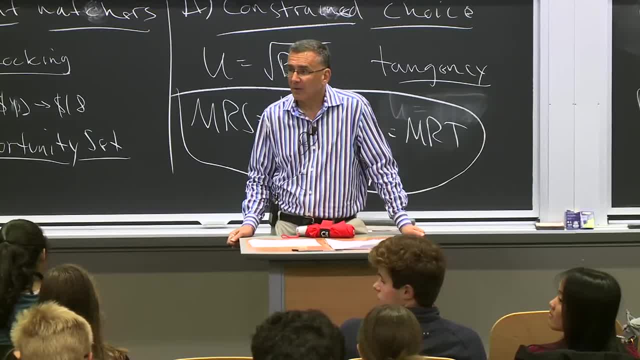 to spend their resources. Yeah Well, like, can't you put it from the perspective of like: this is taxpayer money, right? So then aren't you also just factoring in how the taxpayer wants to spend their money, and then? 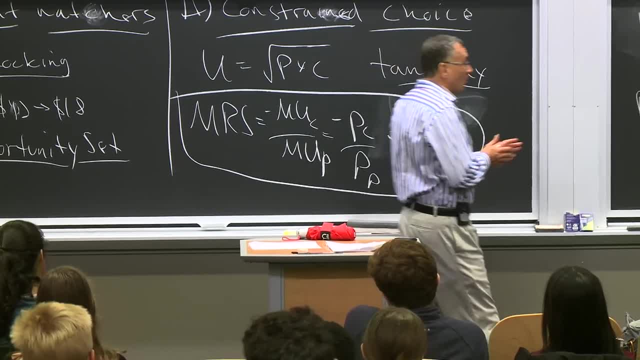 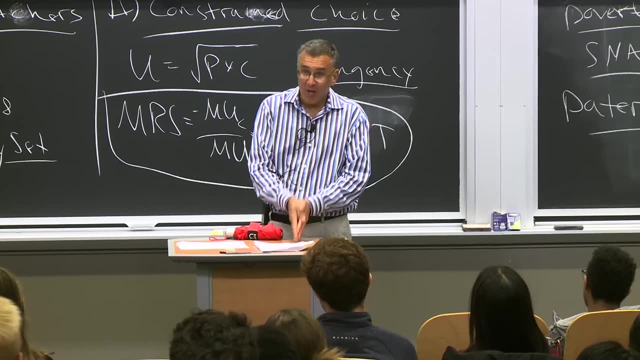 they're in the first group and they're all there. That's a very good point Now, but there's sort of two points there. First of all, if the taxpayer's goal is to help poor people, then why shouldn't you make them as happy as possible? 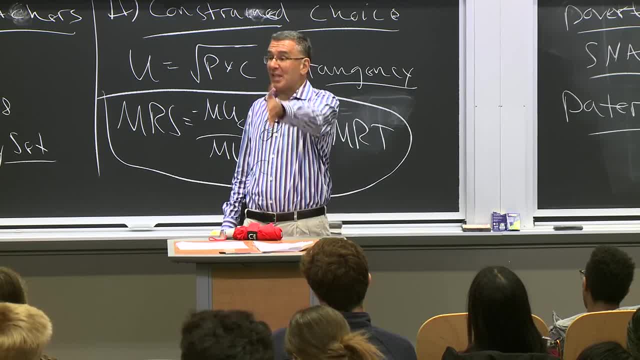 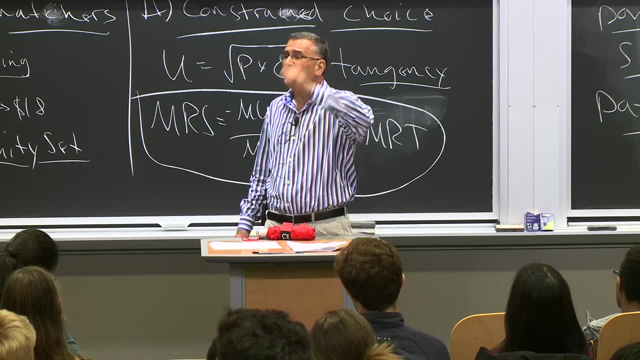 Right. Why am I giving money to this poor guy? Because I'm sad he's poor. But what you're saying, I'm not actually that sad he's poor. I'm sad he's not eating. If you're really just sad he's poor. 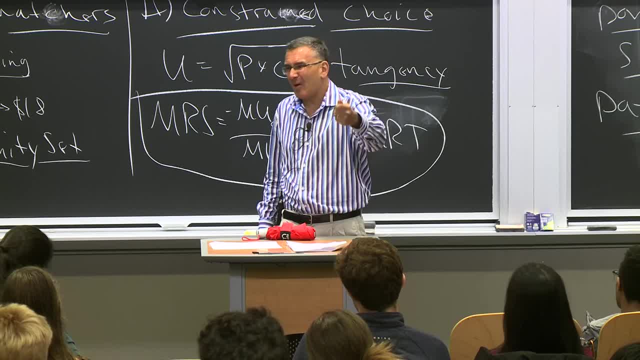 then you should give him money. If what you're sad about is: gee, I don't like how he's living, I don't like his. I'm sad he can't have better food to eat, sad he has a place to live. 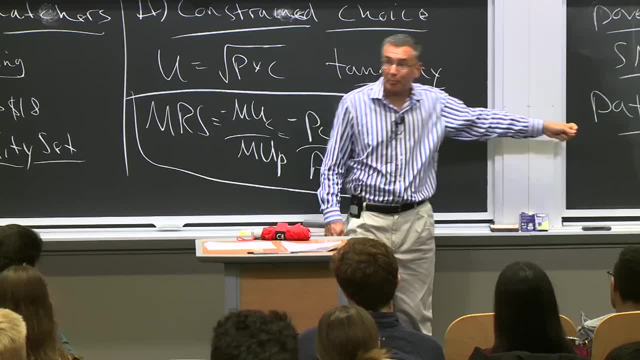 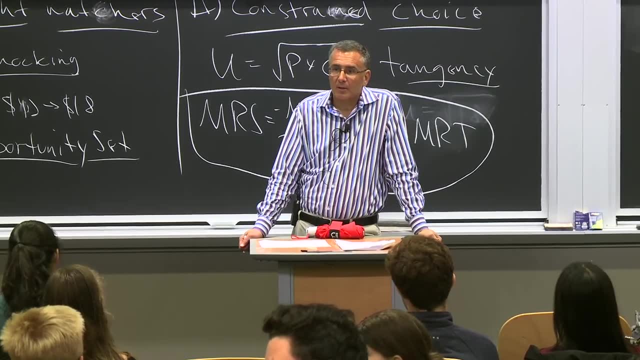 Then you're starting to impose your preferences. But let's be important, That's imposing your preferences. Yeah, I feel like the difference here really goes for happiness or contentedness. But really the point of SNAP isn't really with contentedness or happiness, but rather 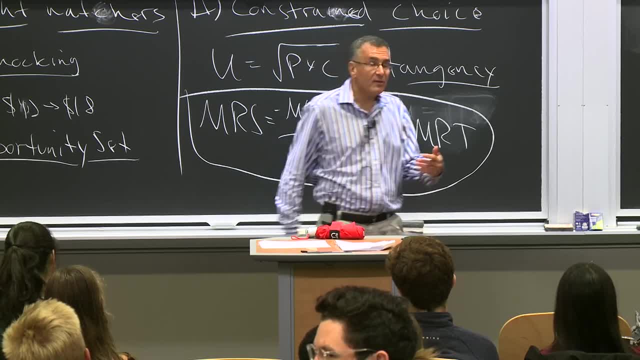 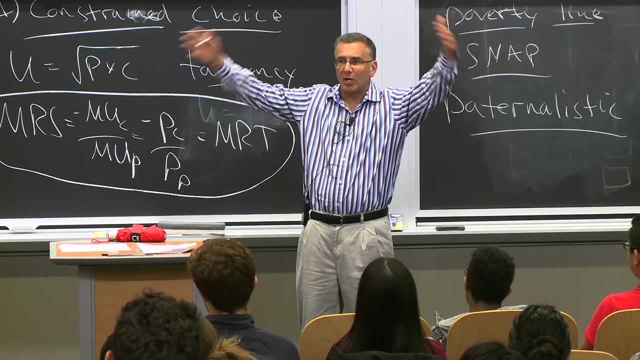 like what would lead to a more sustainable life. JONATHAN GRUBER- Well, that's a related point of the taxpayer, If the taxpayer cares about. look, we want a healthy populace that's going to live a long time and be productive and pay taxes. 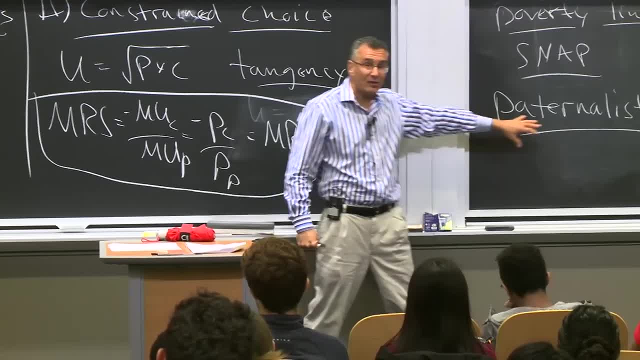 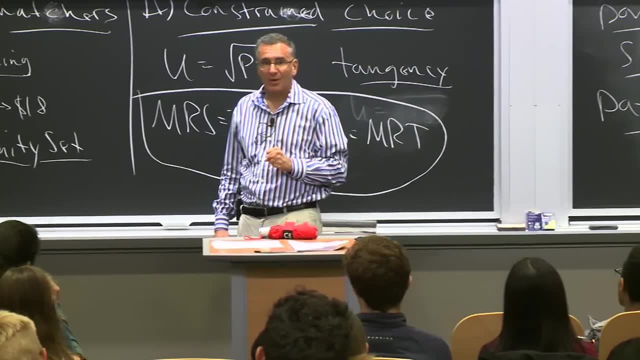 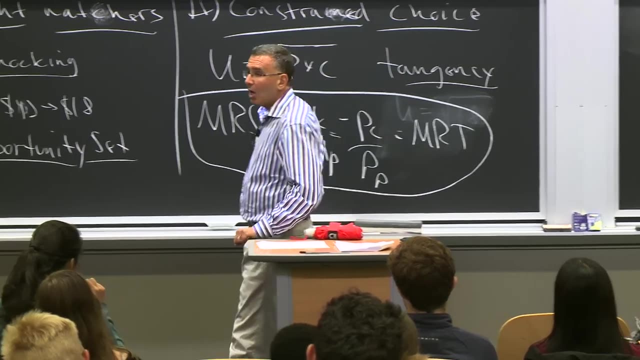 then that would be a reason to do this. But once again I want to emphasize: this is paternalism. If you really just care what makes people happiest, you should give them cash. So that raises two questions, First of all. first question: 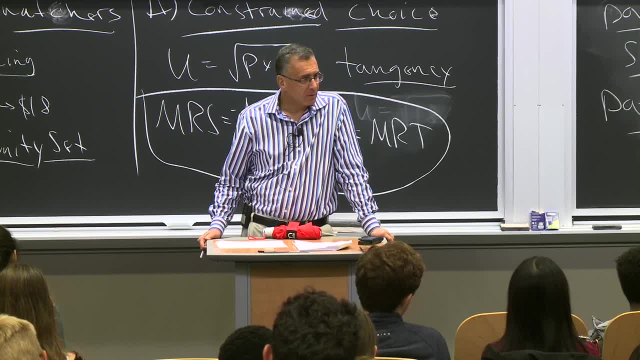 Yeah, So how does the negative negative turn out? This is, for example, if we bump a lot of money, If we allow people to spend a lot on shelter, that's not really going to help people, It'll just make the. 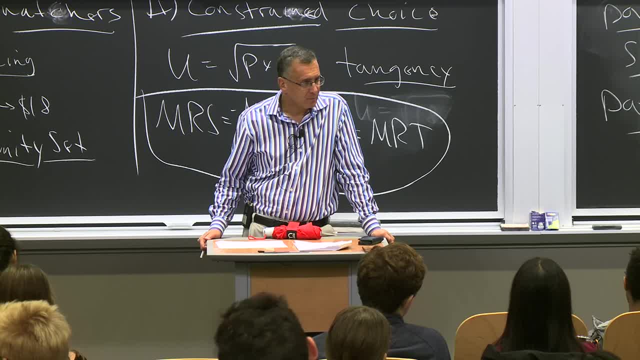 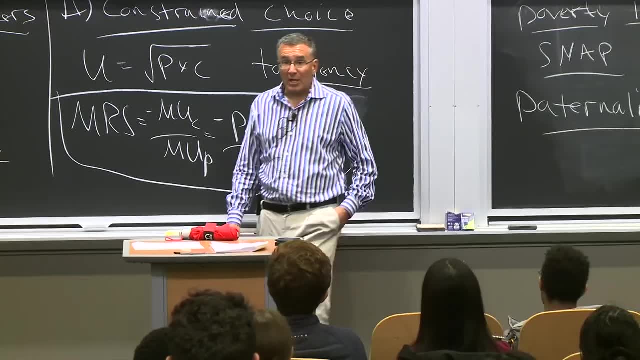 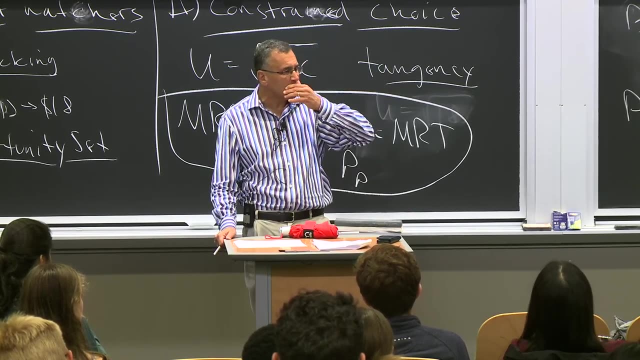 JONATHAN GRUBER- Yeah, yeah. so basically it's a great question. In general, I'm going to answer a lot of those questions with the same cheat this semester, which is we're going to assume the markets are perfectly. 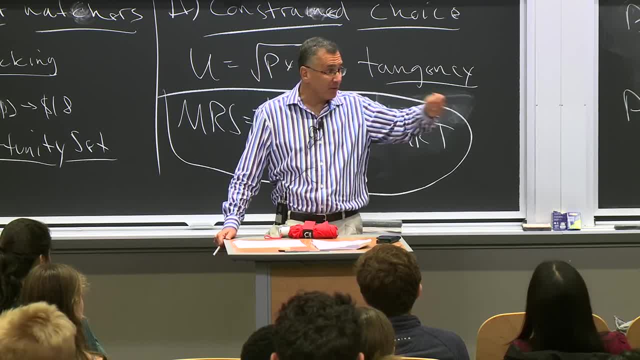 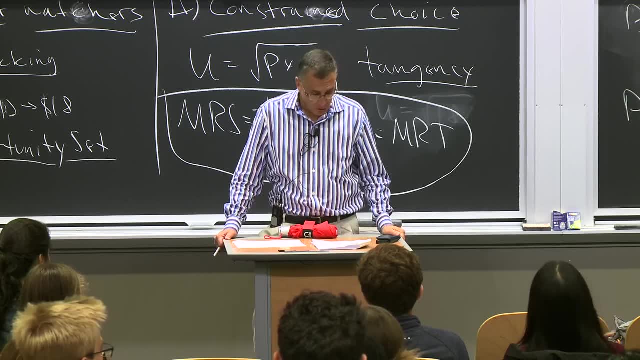 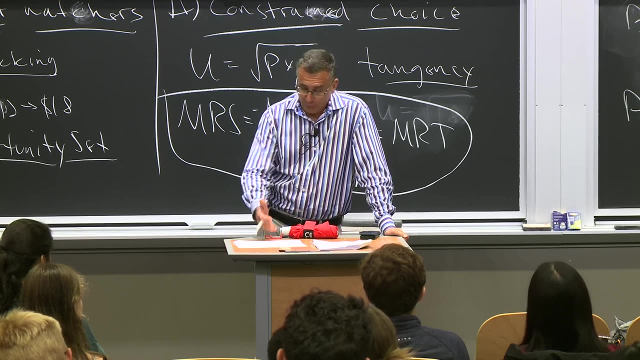 functioning, So you're imposing sort of a market failure. Once there's market failures, all bets are off. With no market failure and no paternalism, you'd want to give them cash. So this raises an important question: Do food stamps actually increase food purchases? 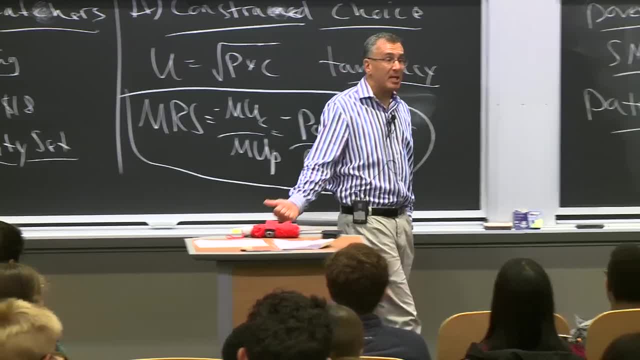 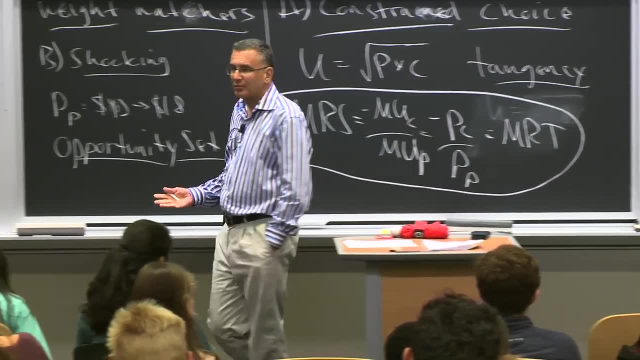 First of all, there's two reasons why they might not. Reason one is: everybody can be like why? X is sort of a silly case. right, You're going to die if you eat that little And food stamps aren't that much. They're maybe like $3,000 a year. Everybody's going to spend $3,000 on food. So the first issue is the first reason why food stamps may not matter is that, in fact, everybody's spending at least that amount. 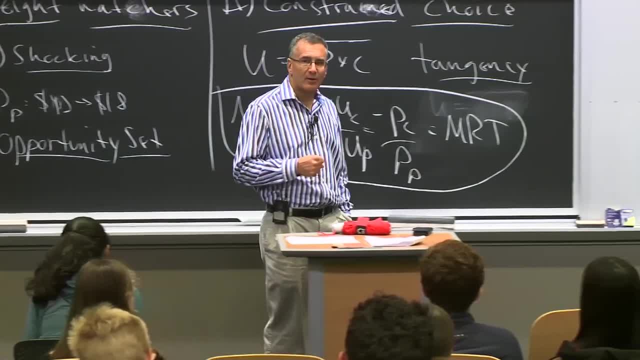 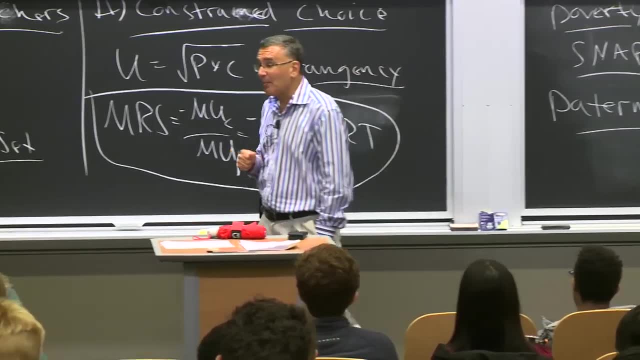 Everybody's like. why Nobody's like X? What's another reason why it might not matter? What's a way people could get around food stamps? Yeah, Buy food at $3,000.. Yeah, They could set up a black market where they essentially say: 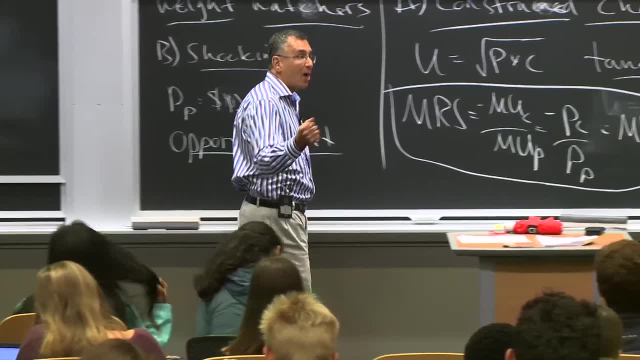 look, I only want $2,000 of food. The garbage is making it worth $3,000.. I'll buy my extra $1,000 of food, I'll sell it to people who do want it And I'll end up still eating $2,000 worth of food. 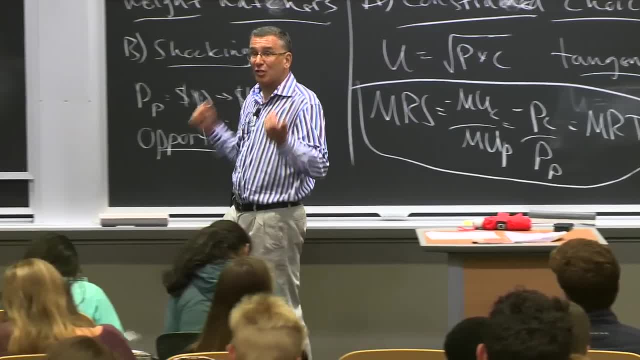 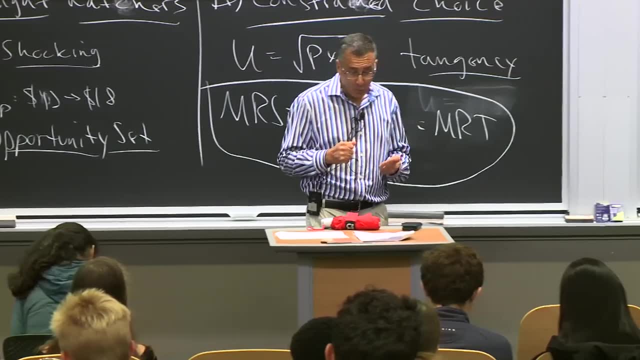 So we actually want to know: do food stamps actually increase food consumption in practice? Are they making a difference? Well, actually we've run an experiment on this. OK, We're going to talk in this class a lot about empirical results in economics. 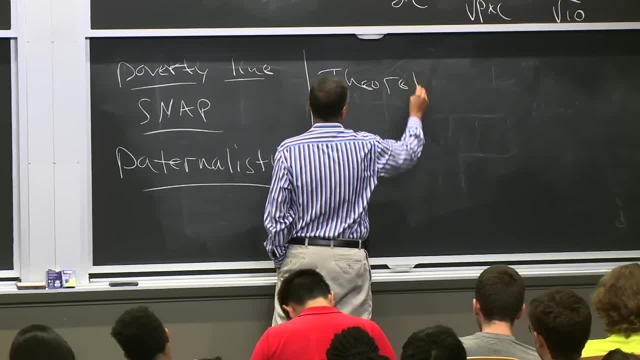 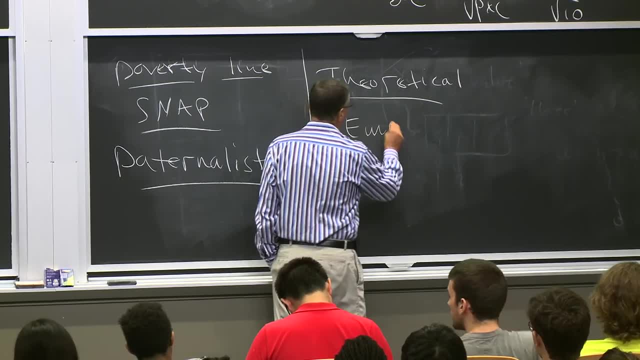 This class is mostly going to be a theoretical class, That is, we'll talk about models and ideas, But we're also- since basically I'm an empirical economist- we're going to talk about empirical economics, which is results and testing the theories we develop. 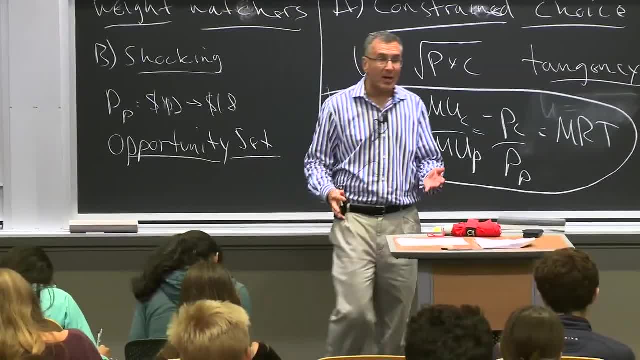 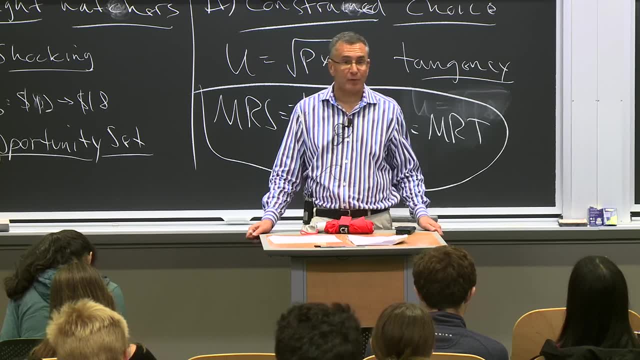 Empirically. here's a great example of empirical economics: is we set up a theoretical model? You always want to start with a theory, but the theory sometimes has predictions which are uncertain. Here we have an uncertain prediction from theory about whether food stamps will affect food purchase or not. 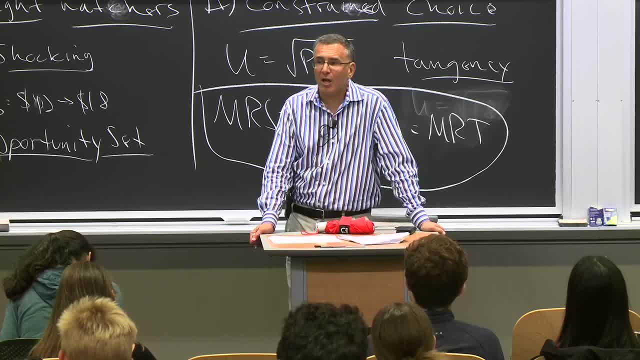 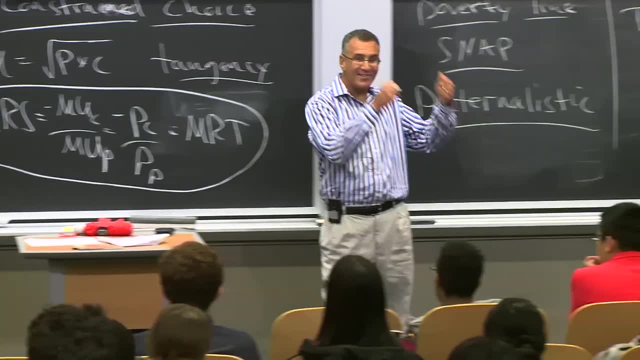 So let's test it. And the way we test it is: we actually have run food stamps, cash-out experiments, where we literally take guys on food stamps and give them cash instead and watch what happens to their consumption before and after. It's a real randomized trial. 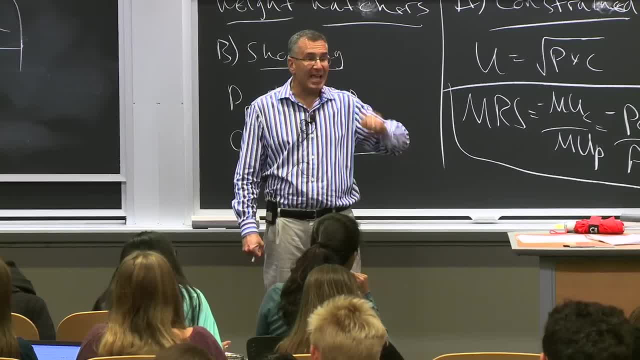 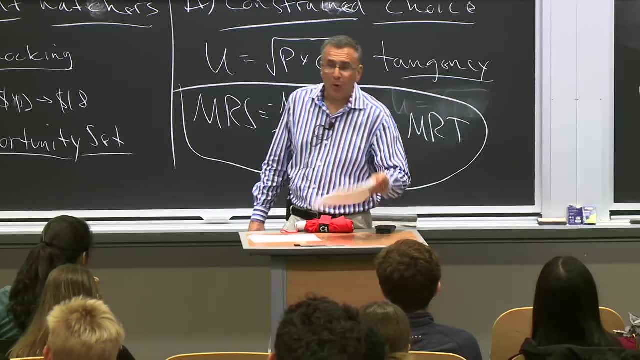 We literally flip a coin Heads. you keep your food stamped Tails. we replace those food stamps with an equal amount of cash. Then watch what happens. What happens is that we're going to test it. What happens is that people spend about 15% less on food. 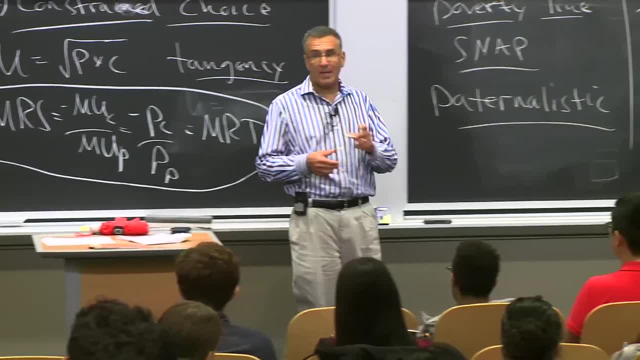 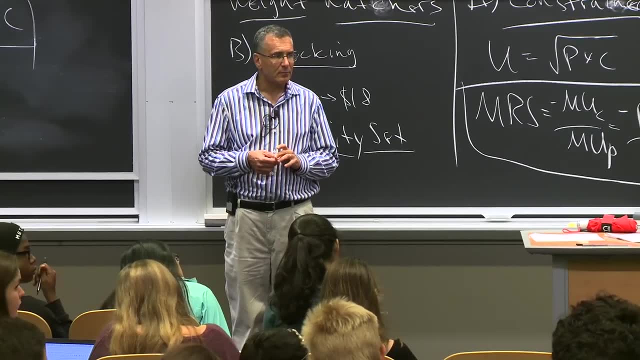 when you give them cash instead of food stamps- That is, food stamps- is forcing people to spend about 15% more on food than they would like to, unconstrained by the cash. Yeah, Yeah, This is going to give you the behavior of. 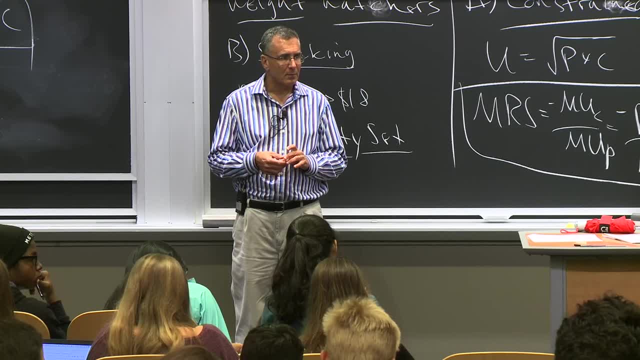 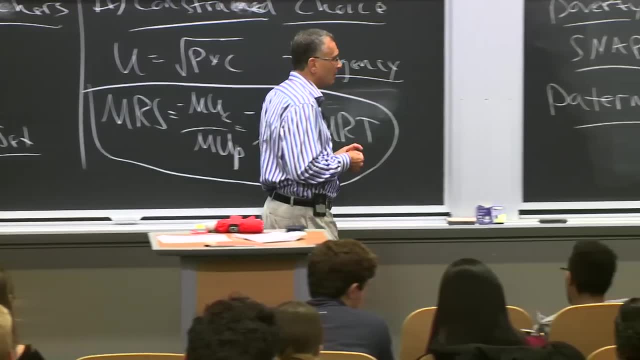 I remember doing an experiment, Like if you have a price of gas going down, you actually use the amount of money to tend to have gas constant, which- and this might be related to food stamps- We did food stamps. Yeah, You know, it's a great question. 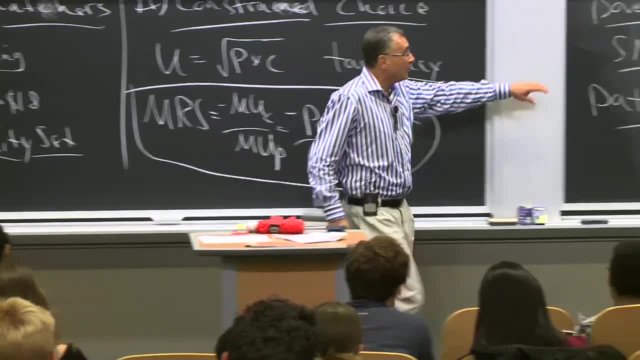 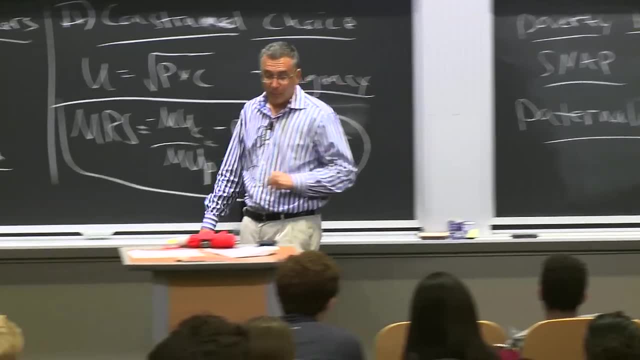 And you're asking about richer theory, richer theory, And I'm telling you that I'm going to give you the empirical evidence. Whatever the theory is, the empirical evidence tells you what happens. There's different explanations for why. So empirical evidence is that basically. 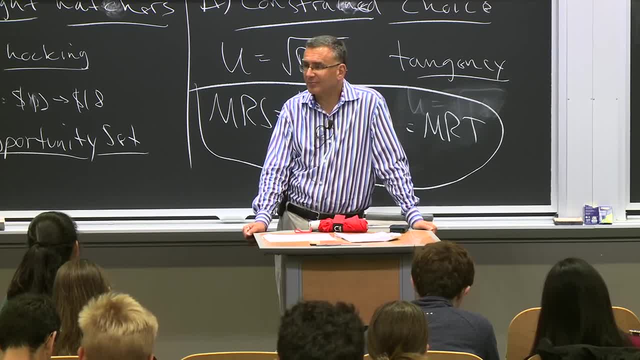 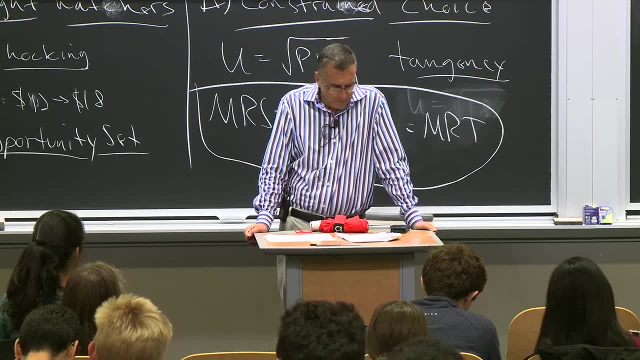 the price of our paternalism is 15%. We are making people effectively 15% worse off, making them spend 15% more on food than they want to. So is it worth it? Well, actually, the evidence is starting to pour in that it. 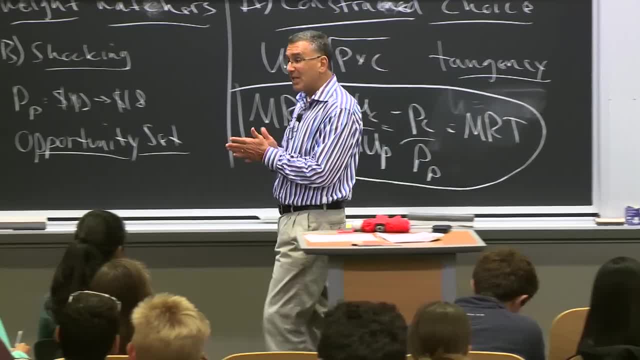 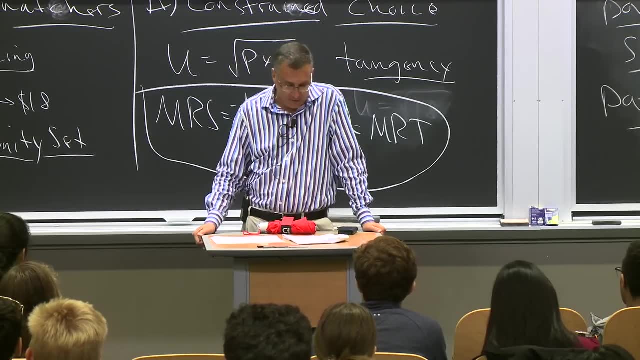 might not be worth it, Because there's starting to be a lot of experiments where giving people just cash- especially developing countries And developing countries- the answer seems to be just giving people cash- makes them better off. That actually especially in developing countries. 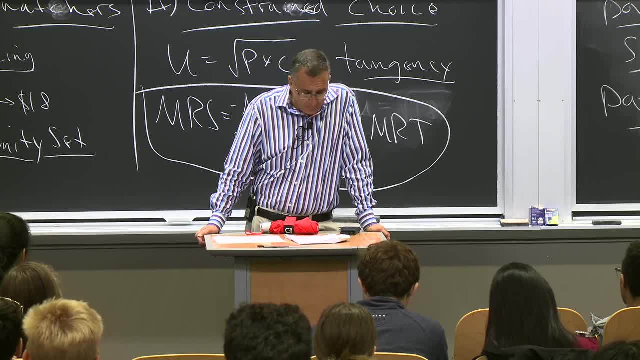 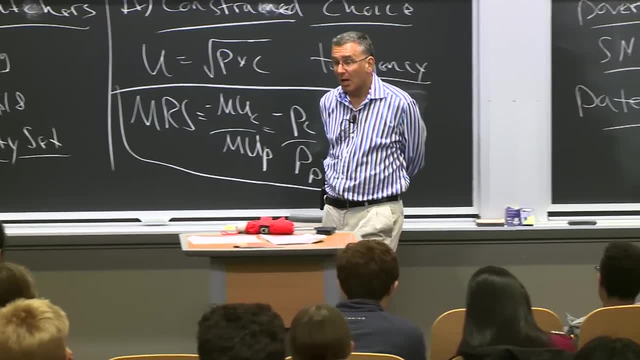 people use the cash in productive ways. So, for example, they have a series of valuation programs where they've given people cash, mostly in developing countries, in Africa in particular, some in the US, And they find that people spend relatively little of that. 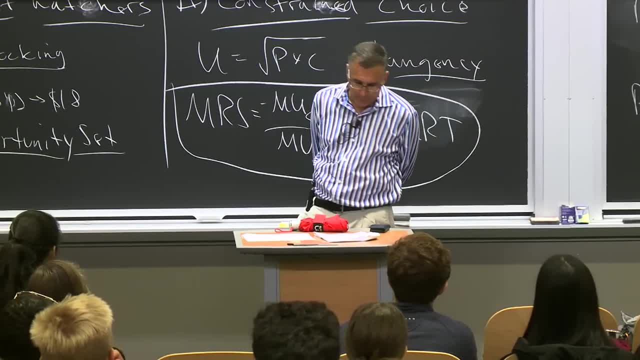 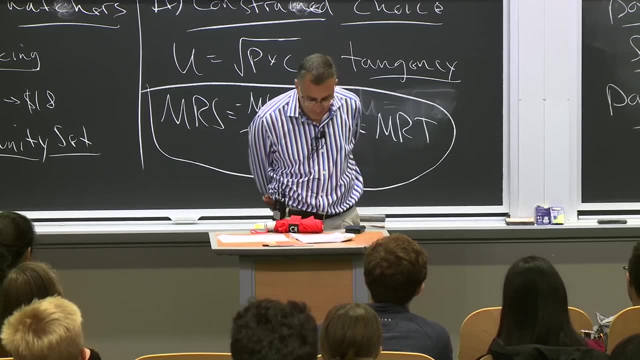 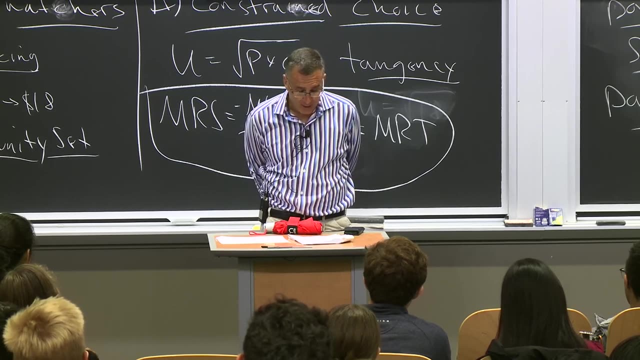 on drugs and alcohol, But they actually tend to spend it productively And in fact, they found developing countries. this all provides valuable resources for individuals to start businesses. So they ran an experiment in Uganda where a nonprofit company randomly offered a group of women $150, which is huge relative to their income. 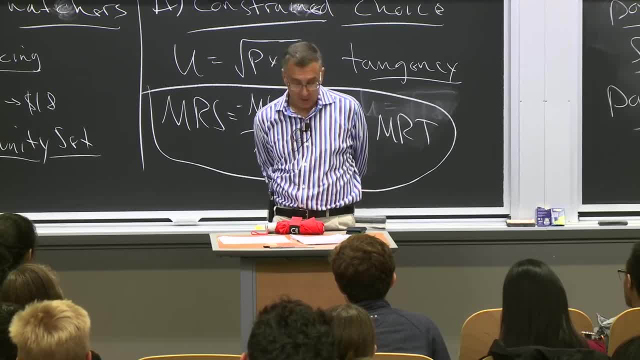 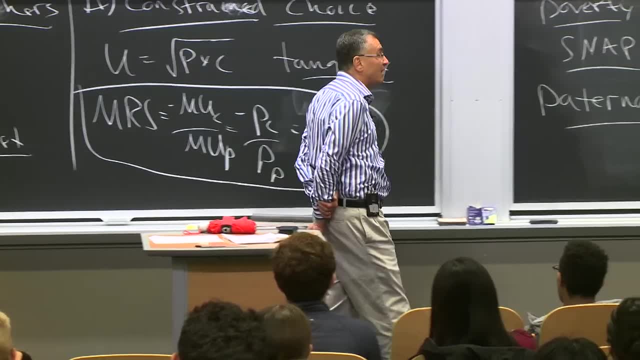 That's 50% to 100% of annual income in Uganda- $150.. And what they found was after 18 months, these women had used that money to start businesses and that actually raised their earnings. that actually effectively doubled their earnings. 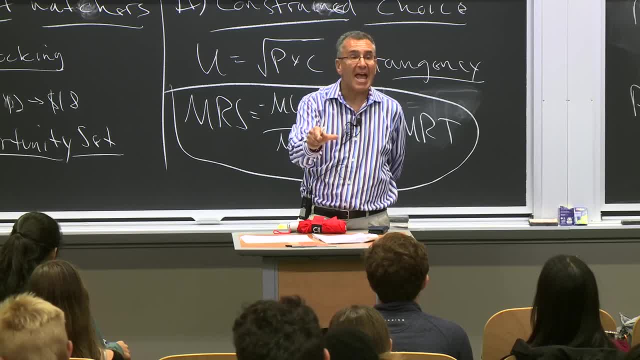 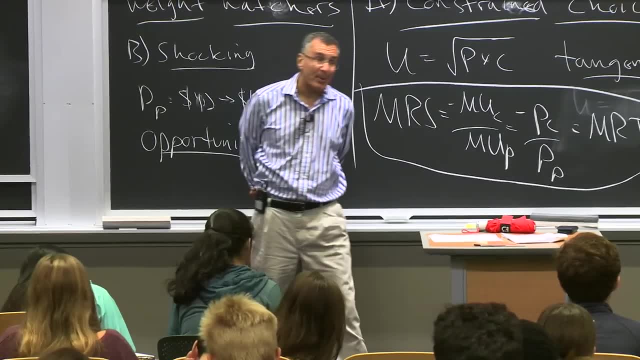 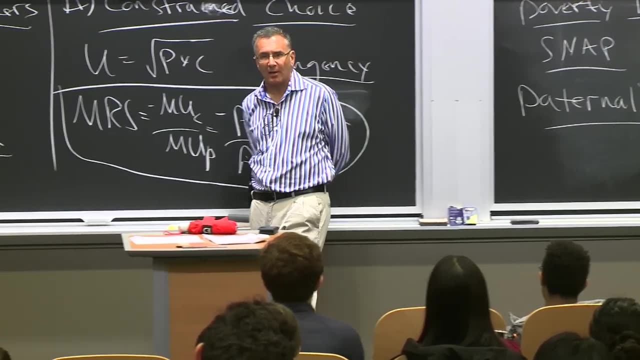 From that one injection of cash. it led them to actually double their annual earnings, So that leads one to think that maybe we should stop being paternalistic and just give cash. Unfortunately, if you're a reader of policy websites like I am, the best one of which is Voxcom. 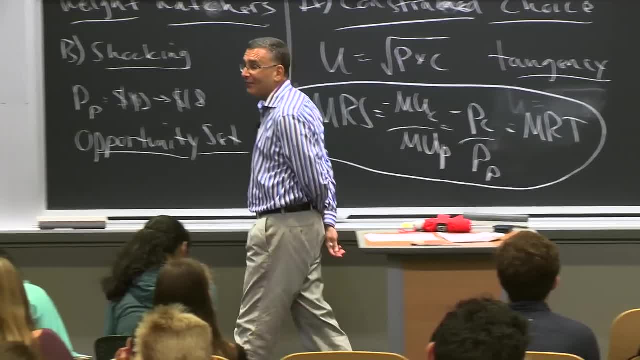 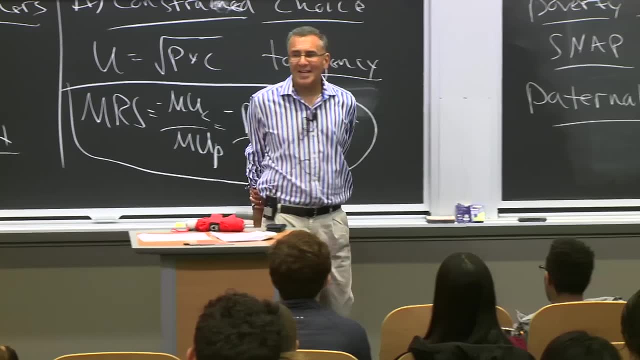 It's a great website. They had an article just the other day pointing out how they actually fouled these women up nine years later. And nine years later the effect had totally gone away. So until you know, the story isn't quite necessarily. 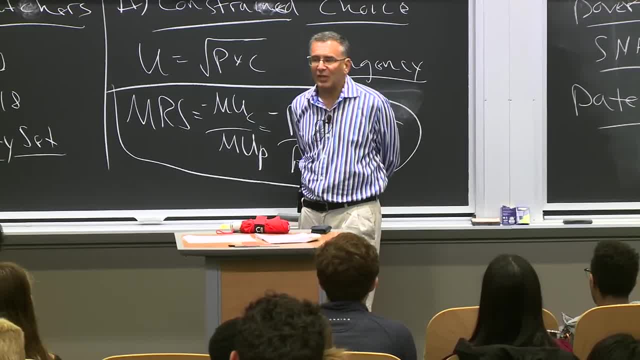 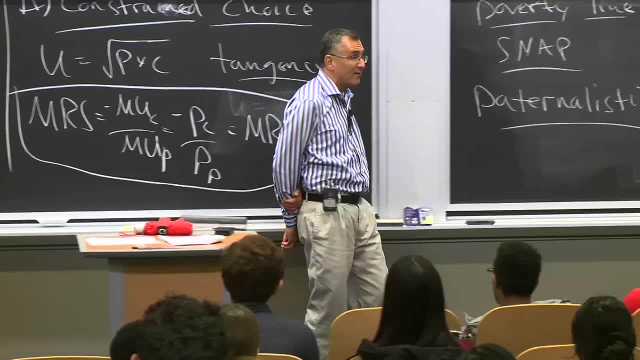 positive, but it's not negative. They're not worse off, But it looks like it at least was in the short run made them better off, while that effect fades over time. But the bottom line is, at this point I think the evidence is sort of probably in favor.